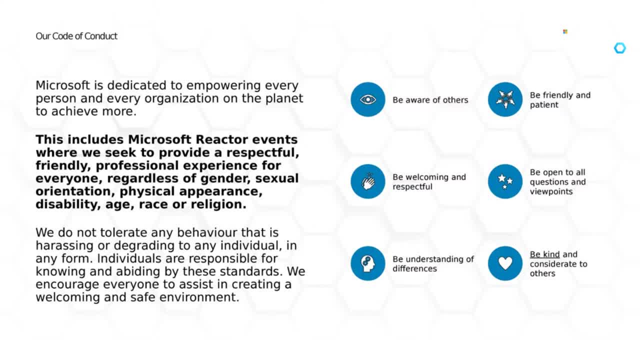 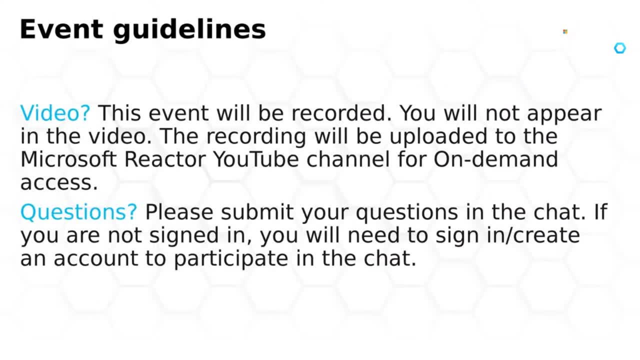 a respectful environment for both our audience and presenters. We encourage engagement in the chat, but please be mindful of your commentary. remain professional and on topic. Useful links will be shared throughout the chat. The session is recorded and will be available on the Microsoft. 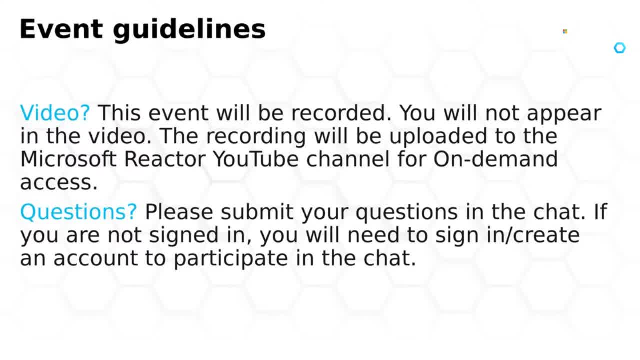 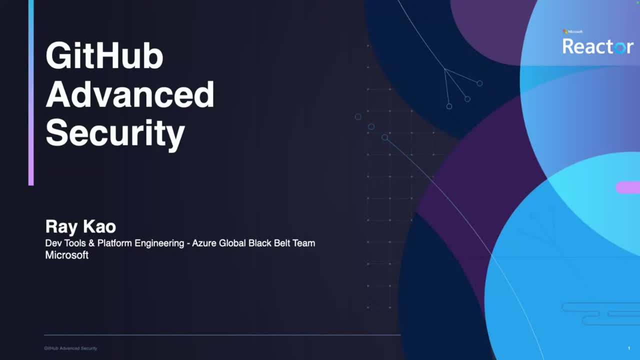 YouTube channel within 24 to 48 hours after the conclusion of our event, Which brings us to today's session. It's going to run approximately for about one hour and there'll be time for questions throughout, So I will now turn it over to our speaker for introductions. 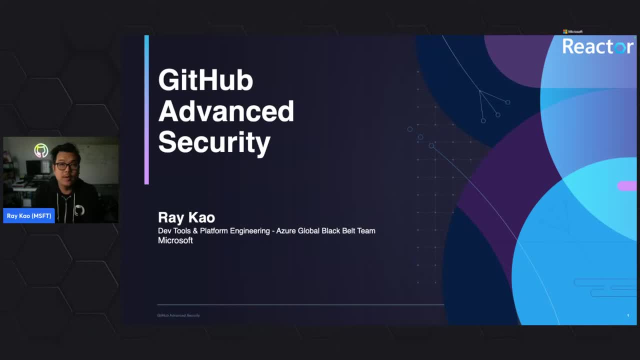 Yeah, thanks, Eskia. Hey everyone, I'm Ray Coe. I am a DevTools and Platform Engineer. I'm a DevTools and Platform Engineer. I'm a DevTools and Platform Engineer, I'm a Television Engineer, And today I'm going to be talking about Gateway advanced security. 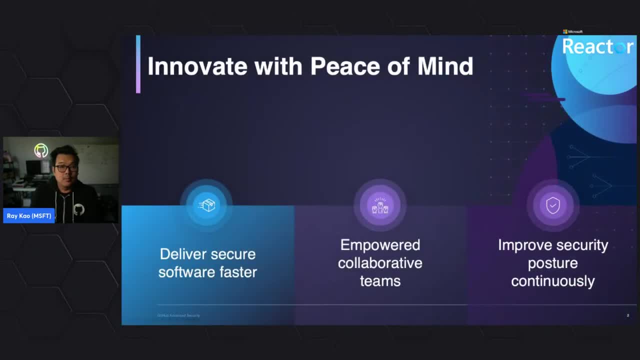 So let's get started. So, GitHub advanced security: what is the point of it? right? What we want to try to do is set the way developers create workloads. In order to do that, we want to provide you a feature that allows you to deliver software faster and empower collaborative teams. 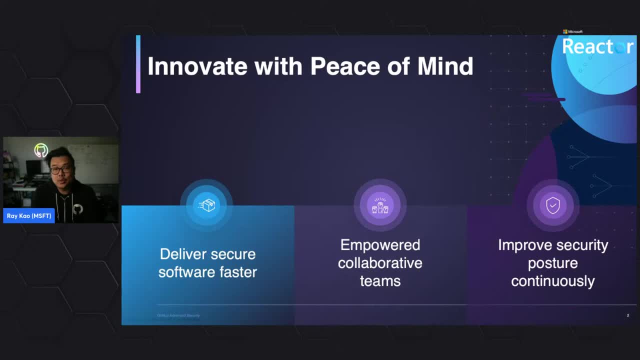 and improve security posture continuously as you write software and deploy it. So how do we go about that? I mean, there's actions, there's code spaces that allow you to deliver software faster, right to set up your environment, But here we're going to focus primarily on the security, end of things. 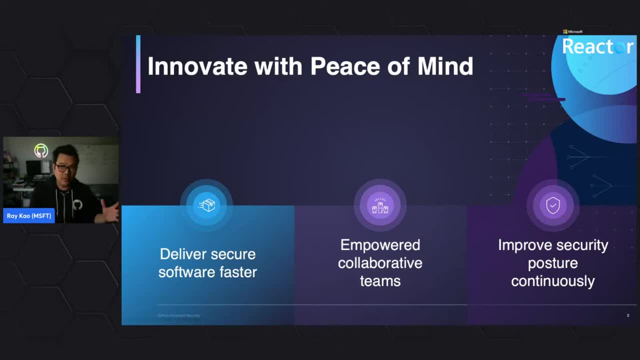 where the whole shifting left movement, DevSecOps and all the other buzzwords around. that is what we're trying to introduce and make easier for you. So the experience is injecting better security practices, catching things earlier and being able to plug into your typical development workflow as a developer, day-to-day. 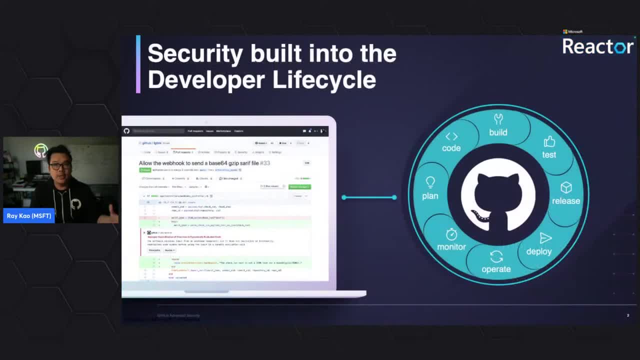 or an engineer day-to-day In order to do that. we're building in the full security lifecycle. I wouldn't say full, but injecting security into your developer lifecycle throughout the experience. So not every piece of this sort of endless circle of development life is going to be injected with security. 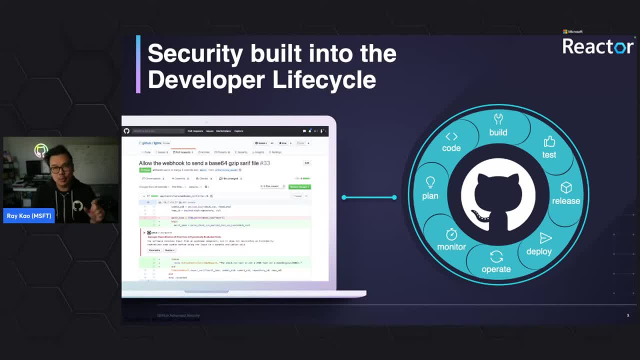 The idea is that at the right points in your experience, in your workflow, that there will be a security checkpoint that you can leverage. Our opinion on that is going to be primarily around the umbrella of GitHub Advanced Security, but there are tools underneath that umbrella that you can integrate accordingly. 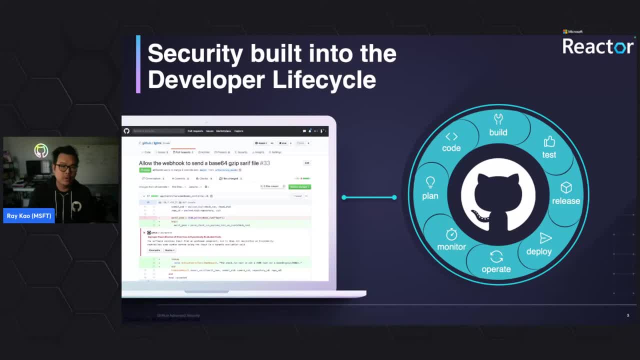 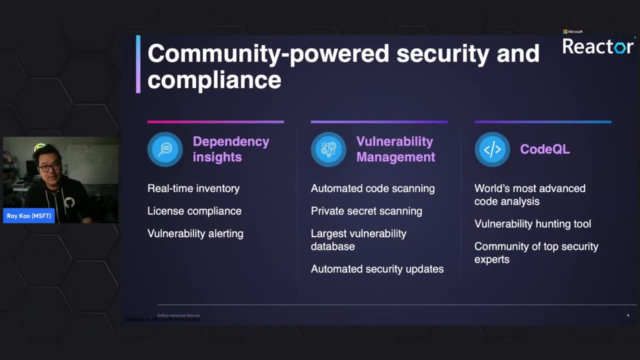 depending on what you need and what's missing in your workflow. To that end, overall, what we're going to be taking a look at is dependency insights or the dependency or supply chain vulnerability issues. You may have heard about that. You may have heard about that. 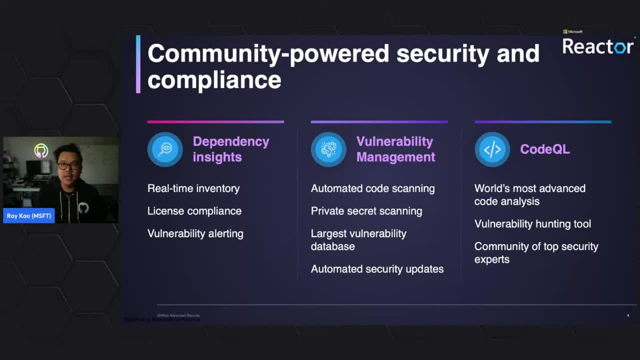 So we will have a capability of seeing the other packages that you rely on. If you write Node packages, if you're a C Sharp developer and you get Ruby, it could be Gems, et cetera, et cetera. This goes on and on. 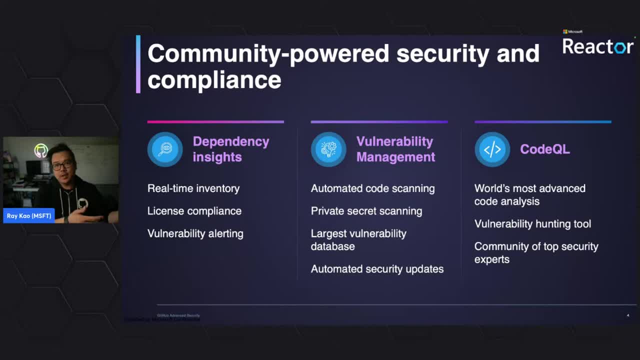 But being able to see that are there critical vulnerabilities in things that I depend on in open source or potentially in the future in a private repository as you build out advanced models around your own software. The vulnerability management itself. the good thing about this when you use Dependabot. 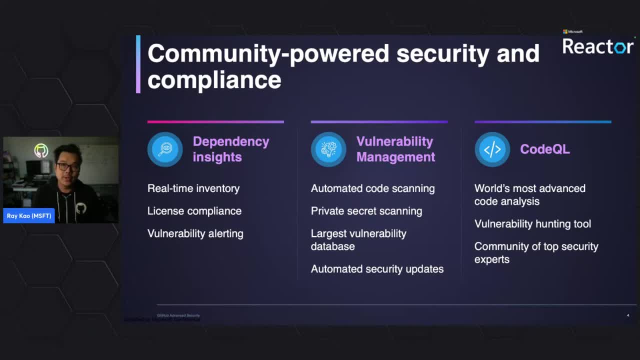 which is the service of the feature inside GitHub, Advanced Security, that will protect you is that it can actually create automated code scanning. It can also provide you with automated updates or revisions or PRs to suggest to you what you can do to actually make your software more secure, and without you actually having to write it. 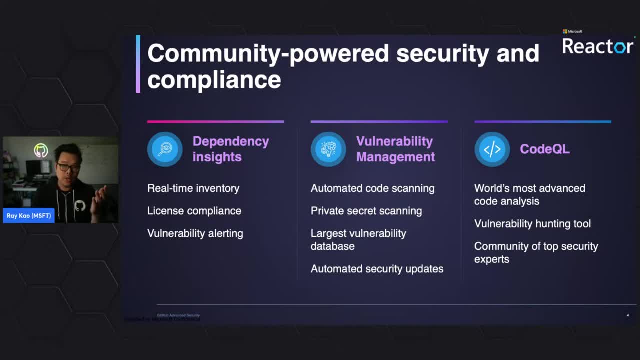 Ultimately one of the most advanced features of this and something that, if you're in sort of bug bounty or bug hunting kind of world or you have a hobby on the side on the weekend, that's what you like to do was just taking a look at CodeQL or our code scanning feature that leverages CodeQL to allow you to generate queries against your source code. 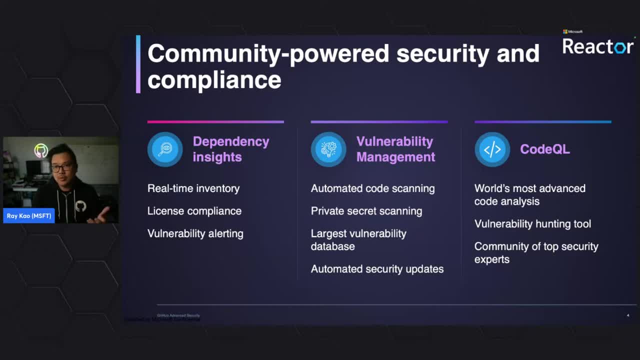 to see if there are, you know, leaks that you might have created. You might have created a SQL injection attack by accident. Hopefully it's by accident. We'll show you an example of that today And you can actually model around trying to catch these things in advance. 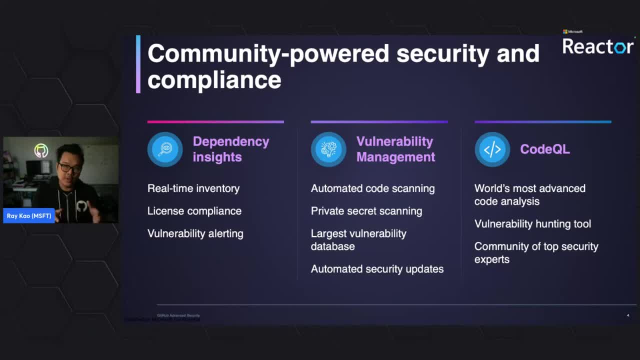 and then put those into your whole development lifecycle, Typically inside your build pipelines and your test pipelines themselves. catch it early, before you actually ship the end product, which could be a jar, file, container, compiled, binary, whatever it might be, before you ship that into production. 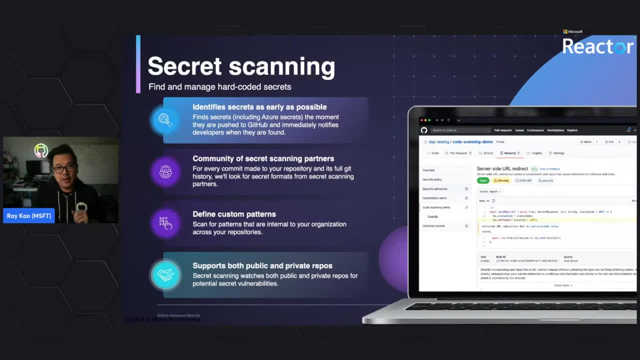 So, in order of the things I'm going to show today, I'm going to start off with secret scanning. I'm going to go through the slides first to kind of do a high level of what they are, And then I'll go into a live sort of walk through the experience and show what it might be. 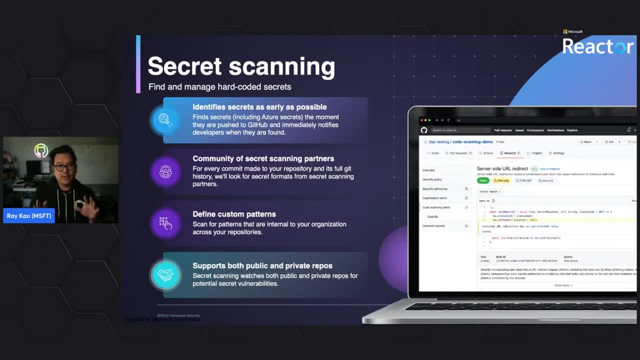 And then I'm going to go into a live sort of walk through the experience and show what it might be. So first, one off the bat, it's going to be secret scanning, And so this is an easy one to implement If you're in all these features under GitHub Advanced Security. 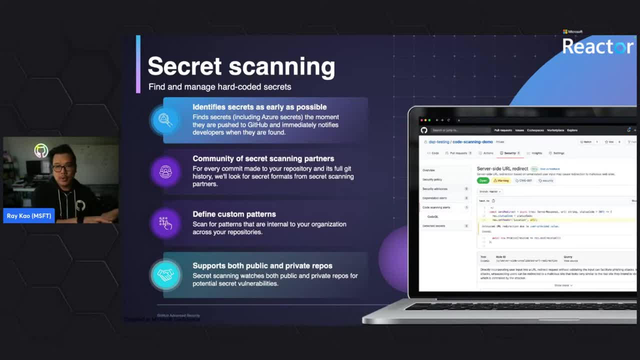 they are available free. if you're in a public repository And then in a paid private repository, it's a different model. That said, you can get started right away with secret scanning. It allows you to basically block or identify. if you haven't turned it on yet, 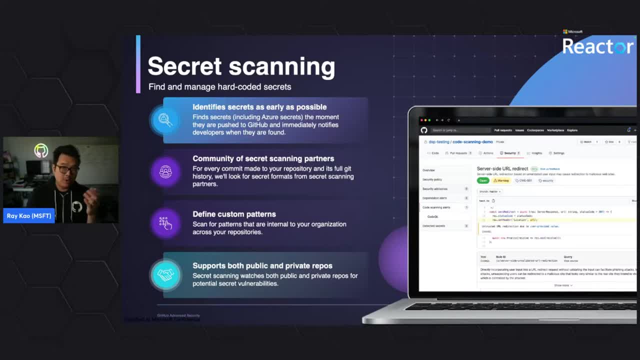 any secrets you may have exposed. It allows you to basically block or identify any secrets you may have exposed into your source code, or it could be readme files or documentation that is part of your repository, And so we work with vendors behind the scenes. It uses AI to scan your actual repository. 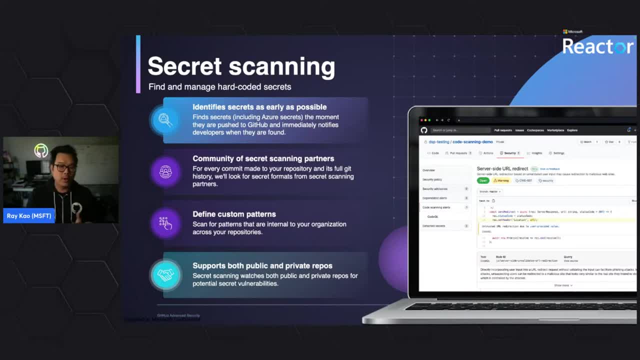 It uses built-in models to check for patterns. So in today's example, we're going to be showing certain API keys from other vendors, like Stripe as an example, that you may have put into documentation which are not actual live code. So in today's example, we're going to be showing certain API keys from other vendors, like Stripe, as an example, that you may have put into documentation which are not actual live code. 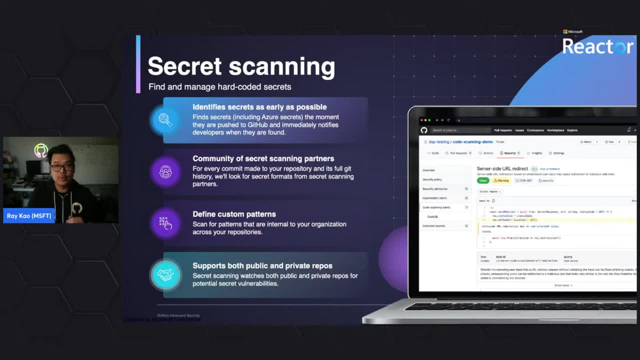 But the feature does detect that and gives you the opportunity to say: hey, you know you should be aware of the particular secret. Do you want to accept it? because it is not actually a live token. Perhaps it's used in testing only and therefore it's not actually a risk. 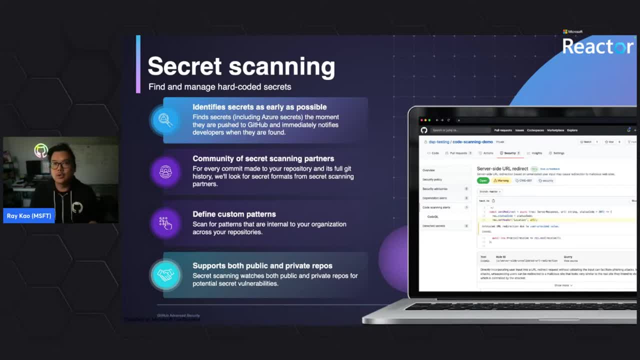 So secret scanning, first and foremost, easy to do. turn it on and it'll check for any hard-coded secrets, passwords, API keys, etc. that may be in your source code. It also just a note and I'll show it in the demo as well. 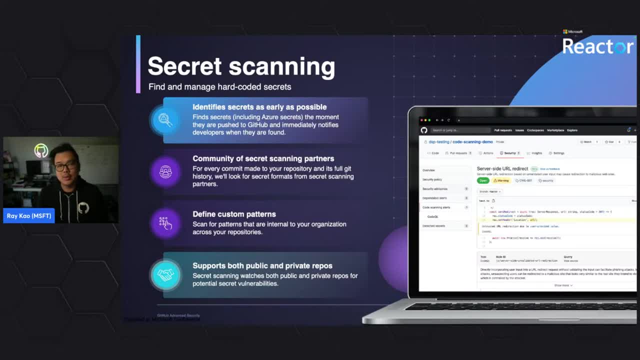 It has the capability, Once you turn it on, to actively reject any commits that you try to push to your repository as well. So it's not just an afterthought, So it's not just scanning after your code is pushed to your repository. It actually actively rejects and prevents you from actually even having that committed into your Git repos. 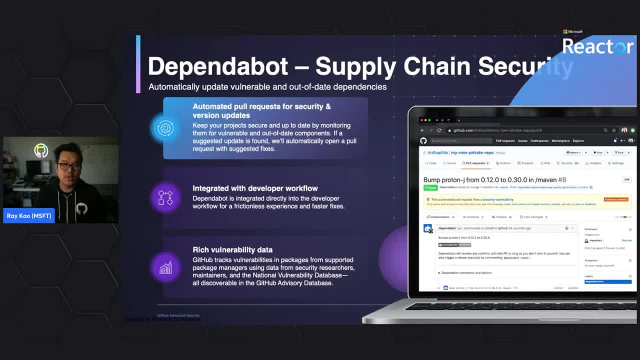 All right, Dependapot. So this is really more in the realm of supply chain security. So you write your own custom line of business application. You depend on additional packages and software From Kubernetes, You have your own community and open source contributions and what have you? 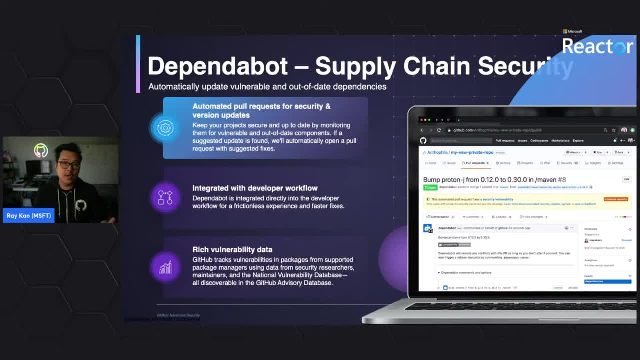 Dependapot is able to see: oh, are you a certain number of versions behind? Is the version that you're using? if it is behind, is it exposing any CVEs or CWEs that are known and reported on? So this does give you the opportunity to see it for yourself firsthand. 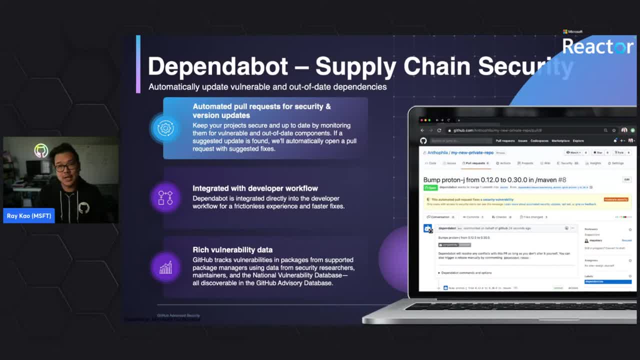 But I think the most important feature about this is that Dependapot itself is able to send you alerts Either via email Or, probably more importantly and better again, as part of your developer workflow, submit a PR to update it Or, at the very least, submit an issue so that you're aware that, hey, this given package is so many versions behind. 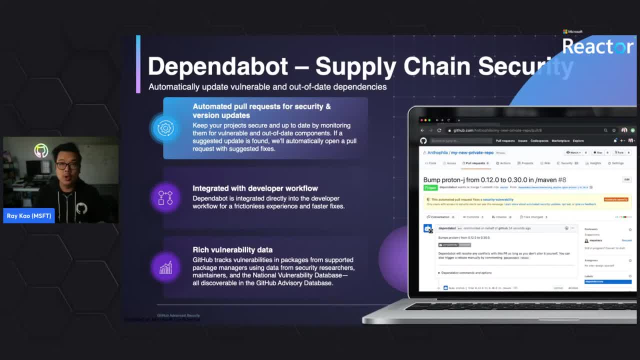 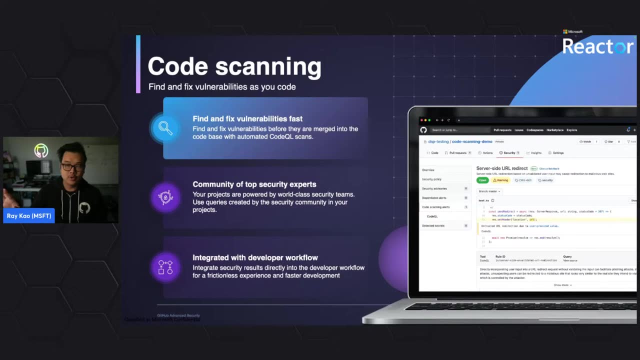 Here is the actual issue behind it And here is a suggestion or an immediate PR to remediate that particular issue with the dependency that you have. All right, Last, before I jump into sort of live demoing how this all works With the contrived application that we have available to us is the code scanning feature. 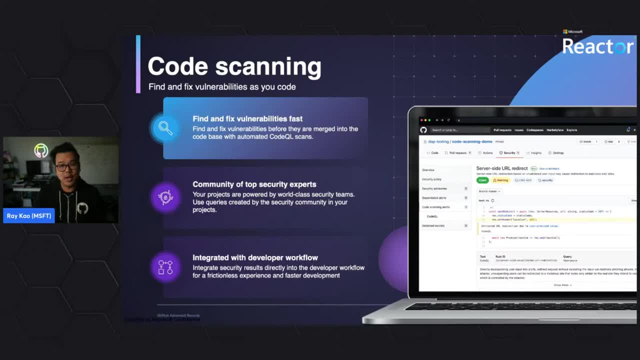 So code scanning inside GitHub Advanced Security is powered by CodeQL. What it's able to do is it models a custom graph database against your actual source code, So it's able to go through and figure out your application. You may have certain expressions, variable assignments. 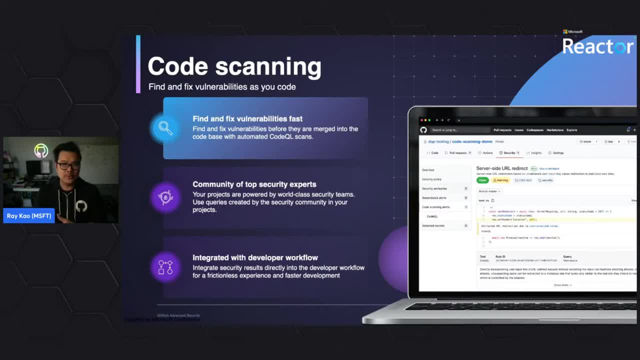 Where Are they being used? Are they passed in as parameters or arguments throughout your other functions and methods in your application? That graph right based on what type of thing is it Again? is it an expression? Is it a method? 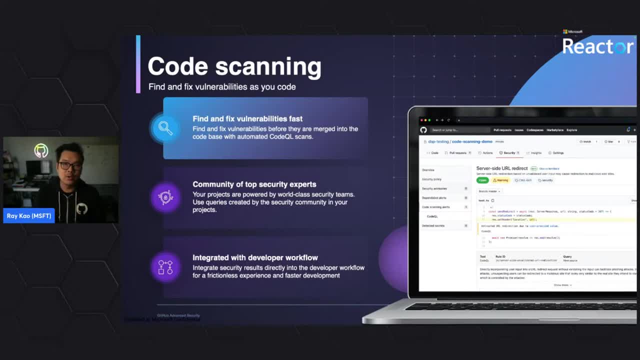 Et cetera. You can search and query against that using CodeQL. to understand functionally, how does my application work? Are there certain patterns that I should be aware of? Do I look for arguments that are being passed in as sources That have been? 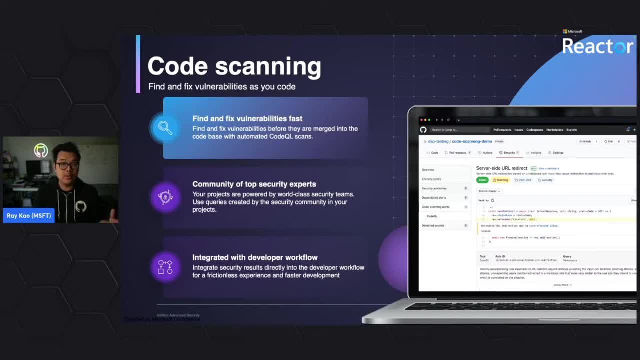 Are they unsanitized, have not been passed through a method that would sanitize and help you avoid things like SQL injection as a result. So super powerful tool. What I have been seeing more and more of is that it's being used in research circles- CodeQL, that is to say, to help detect, generate and actually contribute back to the GitHub Security Lab and CodeQL itself. 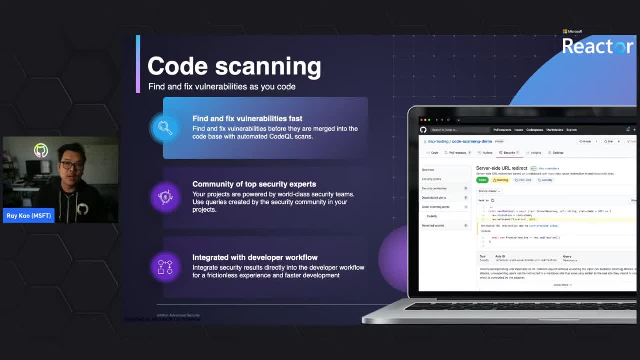 Additional query packs to help protect all of us from known or un-sanitized code. And also it's been used a lot of times in real-time and, whether you are in configuration or perhaps yet to be fully-published, critical vulnerabilities or weakness enumerations right. 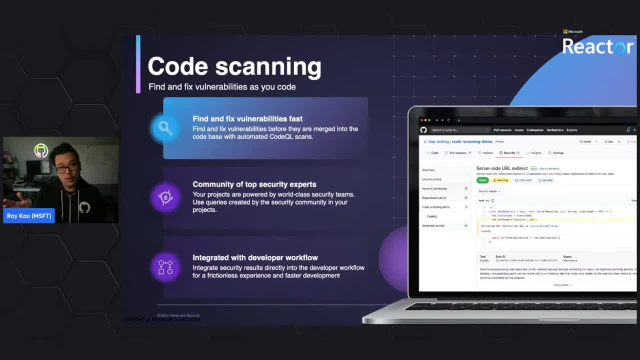 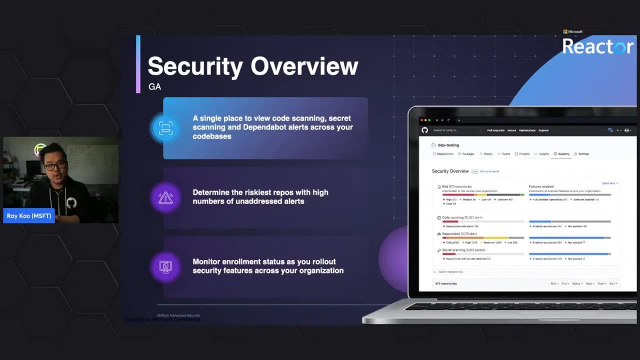 So it's all out there, it's available for you to use and we're going to go through an example of how it detects and how you can actually see it through the security overview. The screenshot here on the right- my right, hopefully it's your right as well- is a little bit outdated in terms of the UI and view of this from the security overview. 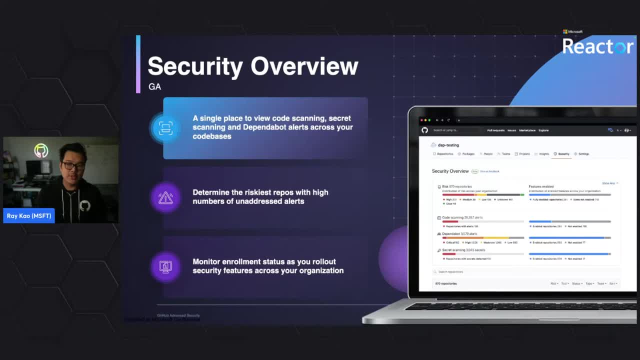 But I'll get into that in a minute and a little bit in the demo. but this will show you at a glance all three of those things, your dependency or supply chain security risk. if there are certain alerts, indicate to what degree is it a high, critical, medium, low. 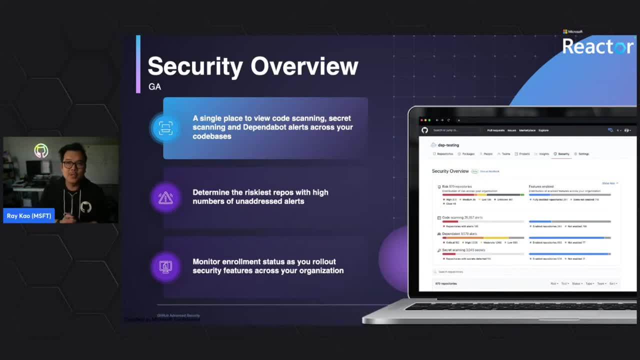 or perhaps it's just like a warning this might be a potential issue in the future kind of thing. So again, I'll show you from dependencies, secret scanning and a code scanning perspective as well. So the reason for this is that there are other ways. 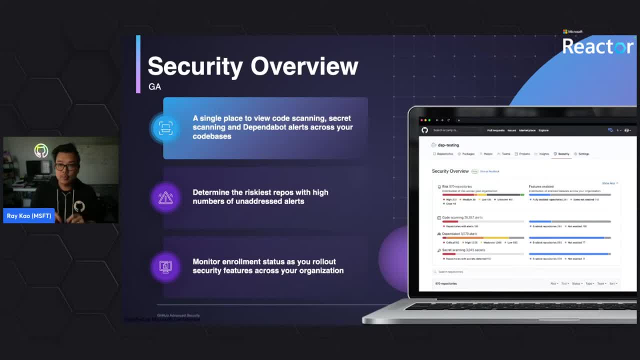 to get that information. Secret scanning as an example, if I try to push a commit where I have a hard-coded API key or secret in there, the CLI will actually my Git push itself will be rejected And you'll see that in your command. 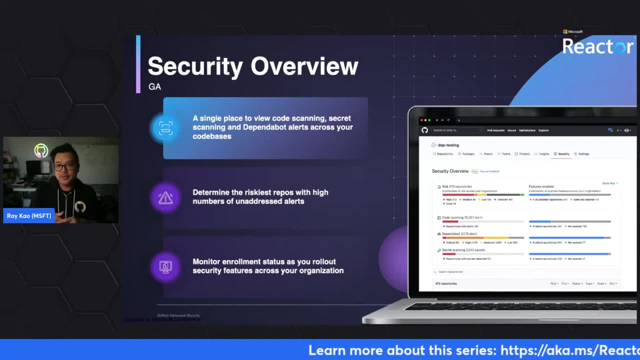 their terminal and command prompt and all that. but perhaps it went through and you want a way to be able to see it. You don't want it to interrupt necessarily your workflow but you wanna have a sort of one-stop shop panel for you to review. 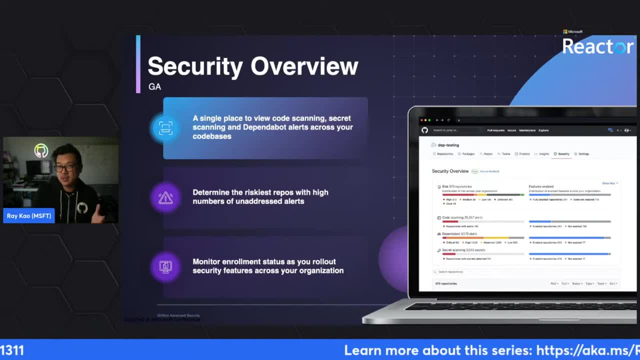 And this also helps with others in your organization who aren't necessarily developers or engineers working directly in the code base itself. Perhaps it's just cybersecurity analysts. I don't say just, I mean other folks in your organization who are responsible for security. 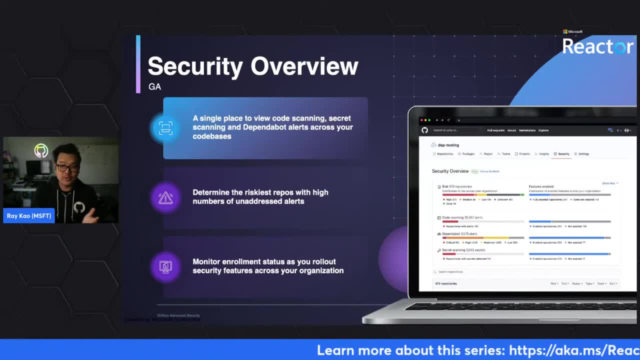 who aren't developers may want a view of this, other stakeholders, et cetera, And this provides a nice view of this. In addition to this, tied or correlated to this dashboard, behind the scenes is an API And GitHub Advanced Security. 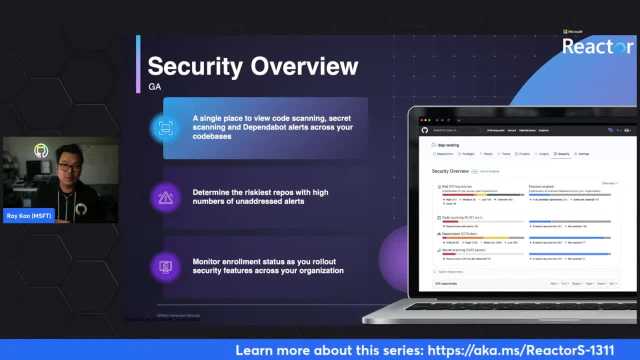 when you tie it to a GitHub Enterprise license, you have access to an audit API So you can generate reports and what have you, and be able to export this information as you need to. All right, So I wanna stop talking after 10 minutes. 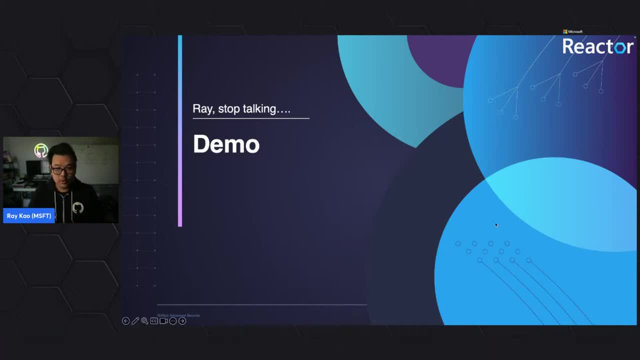 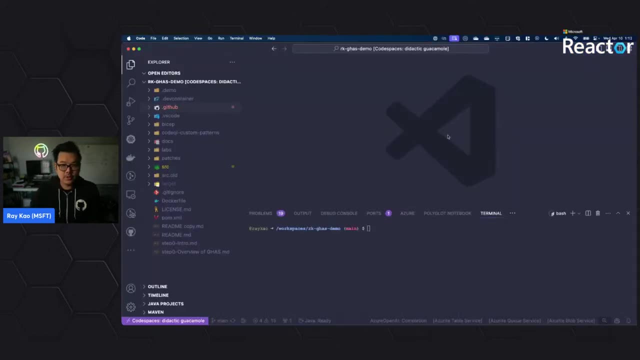 and get into the actual demo of showing you the various features here. So if I context, switch now over to my VS Code session. things to note that I'm running today. just so that you're aware, this is a demo repo built on the shoulder of giants. 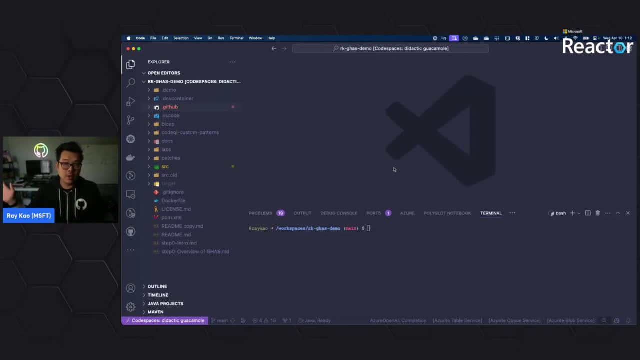 So I'm on the Microsoft side of the house, but our good folks and counterparts over at GitHub have created numerous demos. This is built off of one in particular. You might've heard of Octodemo or whatnot. Hat tip to Peter Murray. 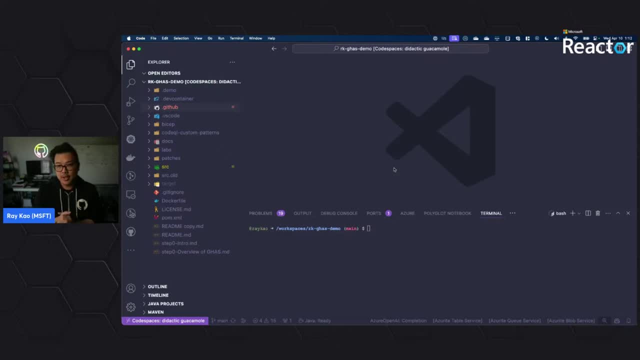 who has helped get this going in the past. I've bugged him a couple of times in terms of setting it up, So appreciate the work that the good folks at GitHub have contributed to this as well. This is spun off of and if I switch to, here we go. 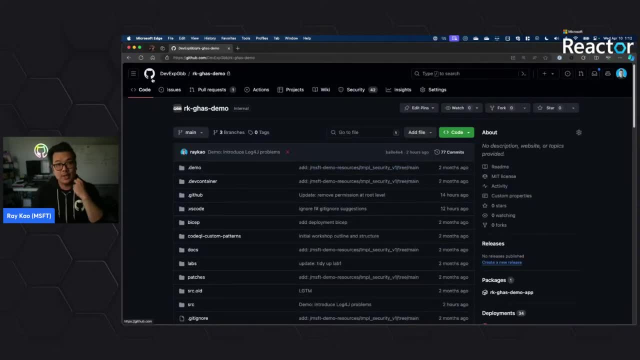 So I'm gonna switch to here a repository I have in my team's enterprise GitHub account And what I was able to do earlier is I'm just as a developer, again part of my developer flow. perhaps I don't have a very powerful machine. 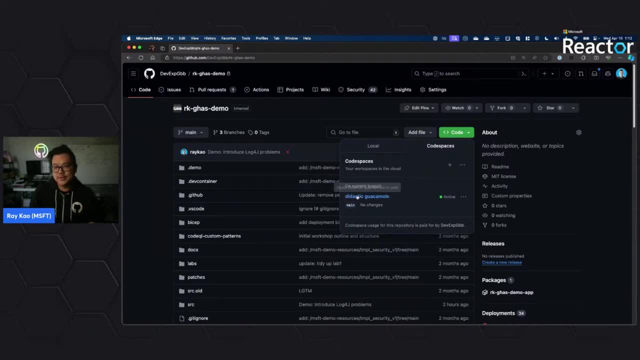 What I can take advantage of here just for future reference, is you can create a code space, And that's what I'm actually working off of. So this is actually a container, kind of behind the scenes, that has my repository loaded and everything that I need. 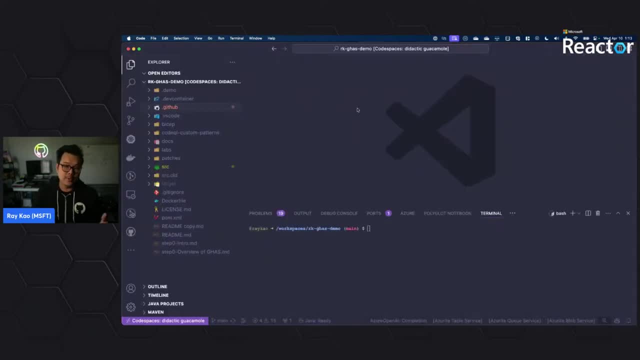 And I can actually load it into my desktop or basically remote into that environment for my desktop VS Code session, And so this looks like it's on my local machine. It's actually GitHub code spaces, All right. with that said, what I want to start showing are the features. 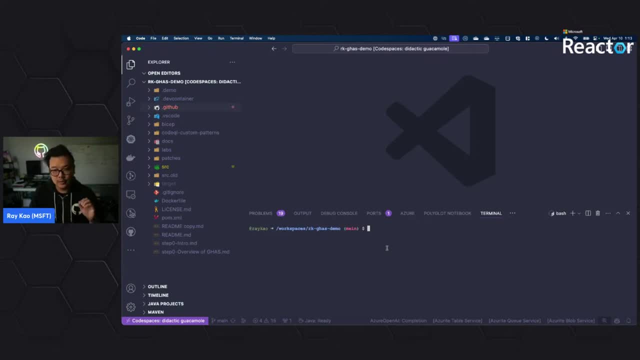 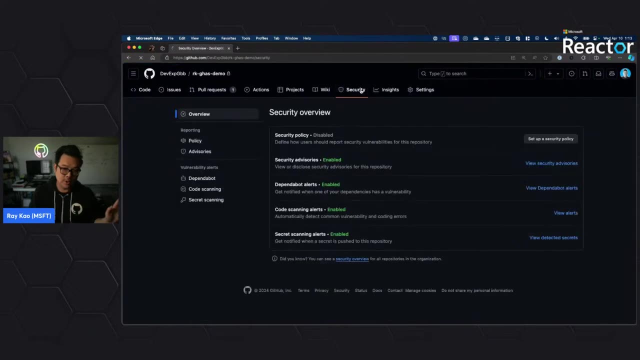 So first off, I wanna go through code- sorry, secret scanning- And I will dive into the security dashboard which is changed from that sort of screenshot I showed a sec ago And this is the default view once I click security. So in any given repository. 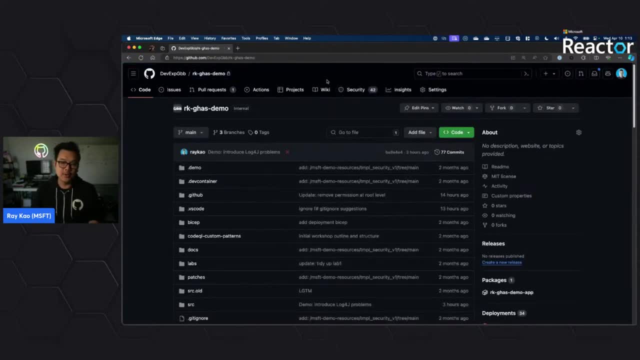 you may have. once you have security enabled, advanced security enabled- you'll see this security tab here. Notice I have 42 alerts. That doesn't mean that it's 42 critical alerts, everything's on fire. It's just you know alerts to say. 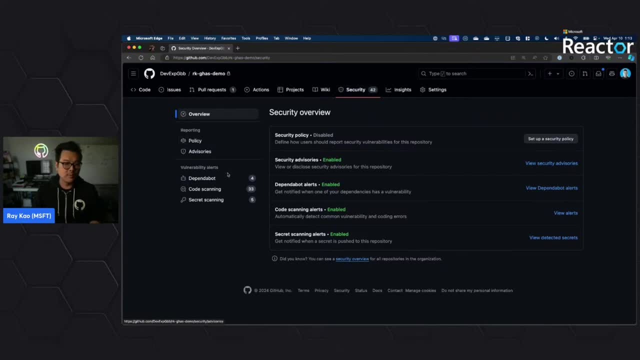 there are things that I should be aware of. Hopefully that's zero, but that would be an ideal case, And this is contrived demo anyway, so I've got a number of them First off the bat, again secret scanning. So I'm gonna go ahead and do that. 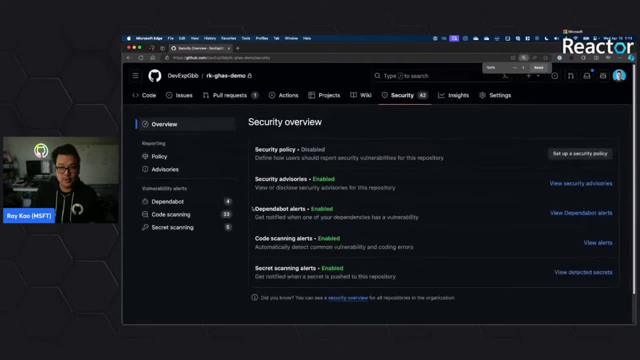 So I'm gonna go ahead and do that. So here you'll see on the left-hand side, if I just increase this a little bit, in case you can't see that too well at home, I've got secret scanning. If I click on that, that'll provide me. 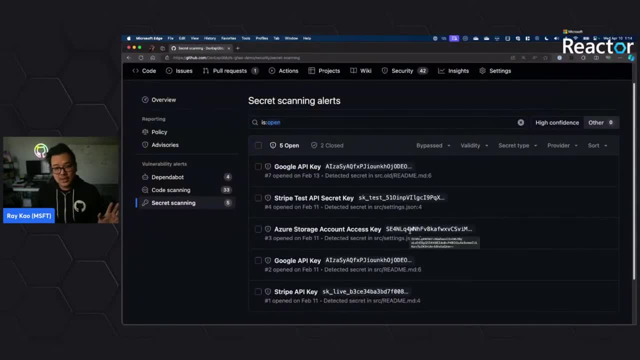 you know the five alerts in here. None of these are active keys. In fact they've already been sort of scrubbed and kind of randomized anyways after the fact when they were generated. So what it will be able to do is: 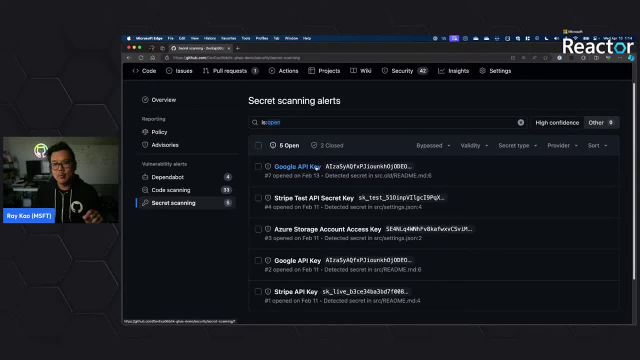 one. if it isn't a known key, it may predict that: oh, this looks like an API. that could be because you've used keywords like password, API key and you've set or hard-coded the variable within your application or somewhere in your README files along those lines. 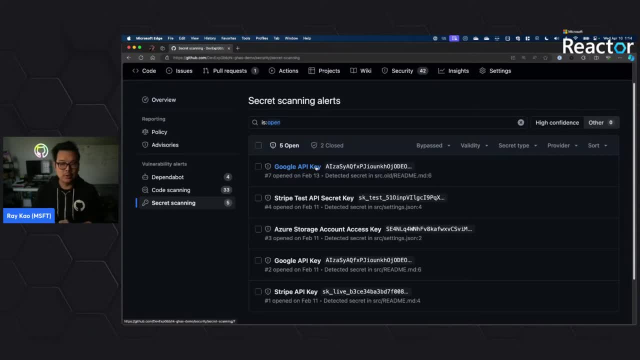 that this could be something that could be a potential leak or risk In this case here. it scanned my repository with commits that were pushed to the repo before I turned on secret scanning. So all of these ones here you're seeing are old ones from before secret scanning was enabled on my repository. 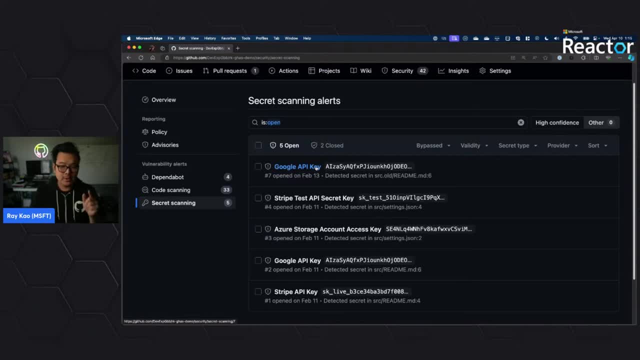 What you're able to see here are the different types of keys from vendors that these keys are likely from, as well as what they're likely exposing. It might look like a blob storage key- storage account key in one of these cases, And the second one, which is what I'm gonna go into. 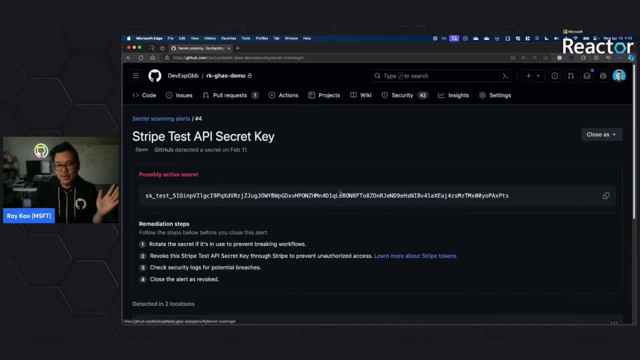 is a Stripe test API key, So a test one, not a big deal. right, That's just test environment, but you still don't want to necessarily expose that. Or perhaps, in the case that I'm gonna show, this key is just for documentation. 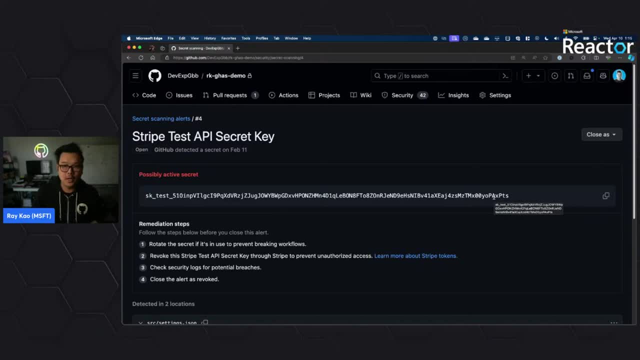 It was just put in there for like handshake in the future for a new developer entering the organization. Or if you're like me, just a note for yourself, because you like to leave inline comments, because you forget things later. Either way, you have the ability to remediate this. 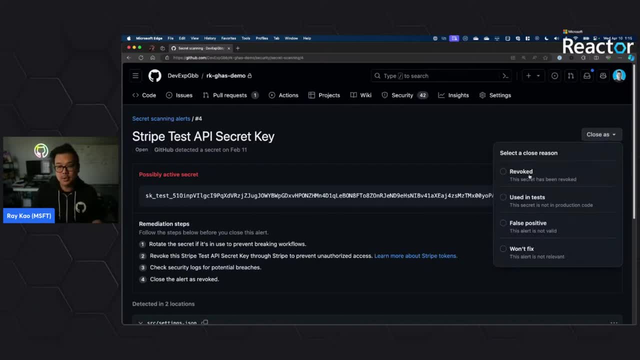 in one way, shape or form, either to say that the key has been revoked- it's actually not production key, so it's only used in testing- or in some cases it might be a false positive, or you're not gonna fix it. 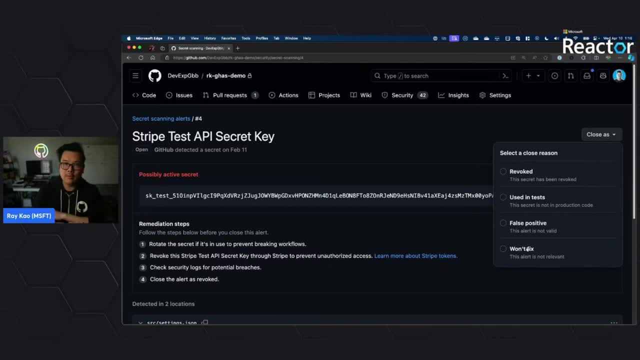 because the alert isn't relevant because, again, it could be used for documentation or whatnot. The reason's up to you. So in our case, here we can click one of these. I'm gonna keep this here because I reuse this repository for other demos. 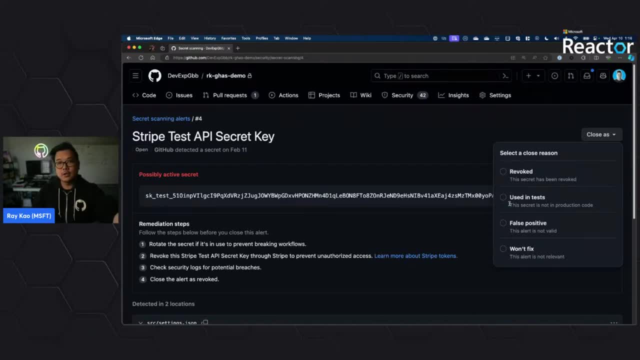 But once I click on this, this generates and creates an audit trail. right? Who actually said to close this particular alert and then post the reason as to why that was the case? right, What I want to show, given the time, it should be good. 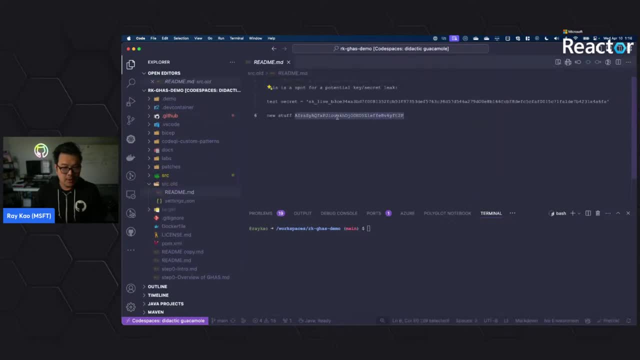 is. I want to go through, you know. I want to go through, you know, a. so this is one of the alerts that we got earlier. I'm just gonna modify this key every so slightly, just to just kind of increment that, so to speak. 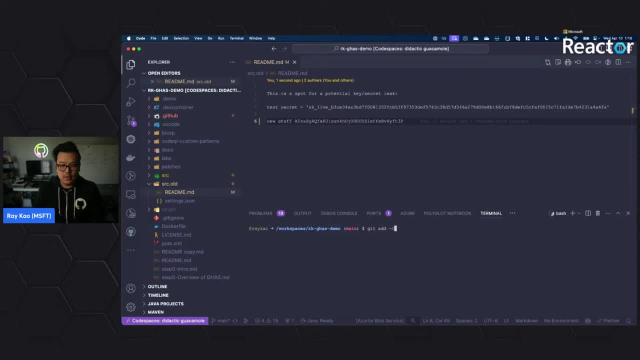 and just to show how this would look if I try to push this with it activated. So I've got secret scanning turned on. I've got it to auto reject any new commits that may be exposing or, you know, adding a new key. 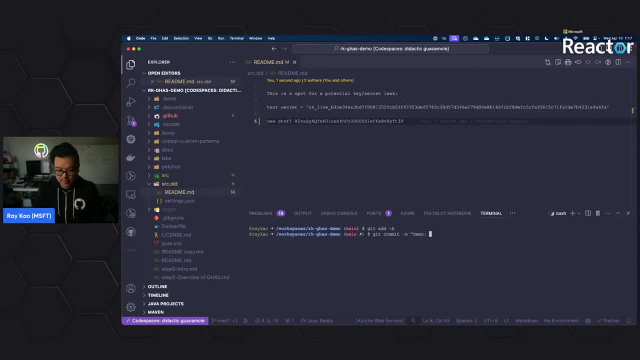 If I did this correctly earlier, demo, just to make a note for myself, creating another API key exposure. Okay, so that looks. you know, usual flow, don't experience. I'm now gonna push this up. What you're gonna see is it did not reject. 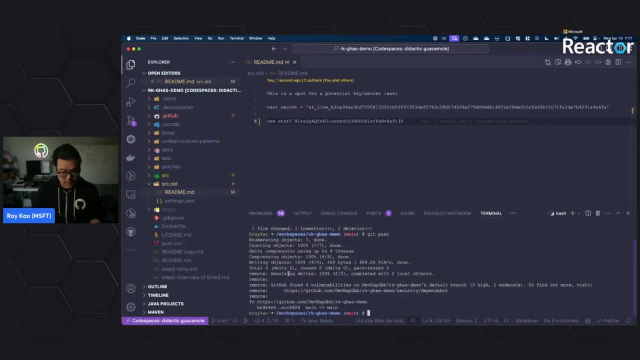 probably because I had turned it off earlier. What you should have seen here in terms of the demo is it would have rejected it and provided me a way to actually circumvent this in a sense that much in the same way that I had the capability of being able to close this here. 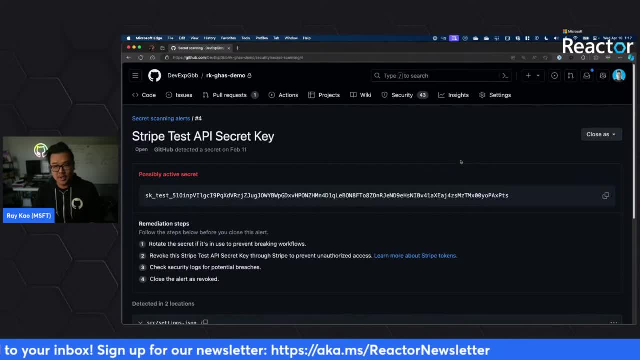 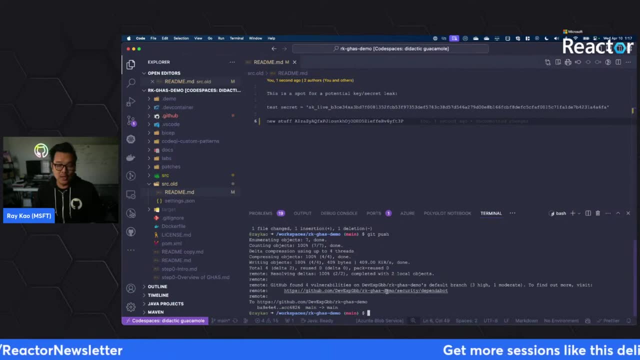 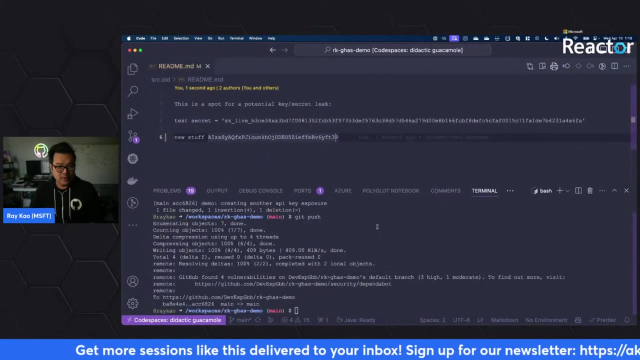 in the UI for a key that was already added to my repository earlier. that would have provided me here in command line a URL for me to open up or click a link, essentially in the terminal here I'm gonna close up- close my panel here. 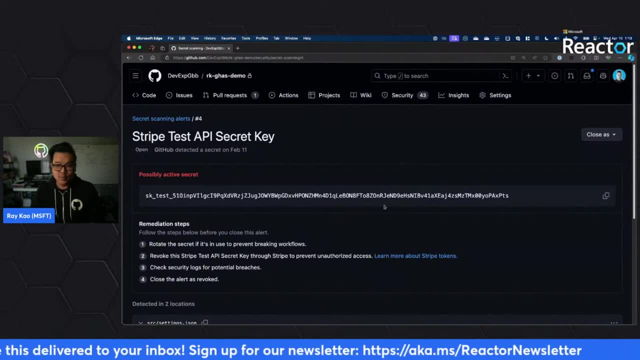 Provide me a link to open up another URL that provides me a web UI that also provides essentially these same close reasons for allowing that particular key. in right, It creates a gated barrier. let's call it so that, if it is indeed a false positive. 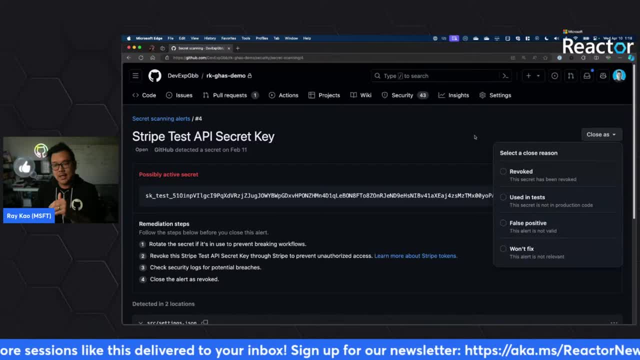 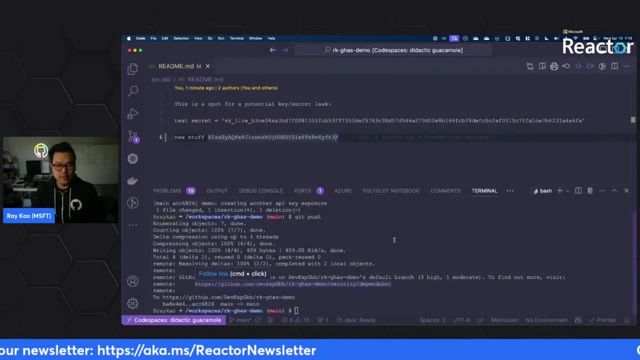 or something that's not a production key, or again the scenarios that we've reasoned before, that allows you to still be able to push the secret to the repository. should it be perfectly fine, all right. This case it didn't reject. 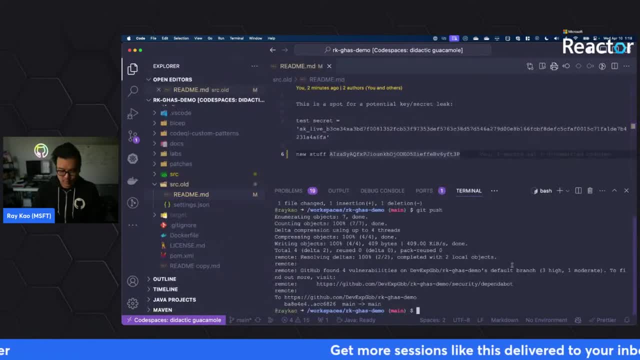 I turned it off in the demo before, so I'm not gonna walk you through. make you watch me turn that back on for now. All right, so that's secret scanning easy to turn on, something I would probably suggest to folks. 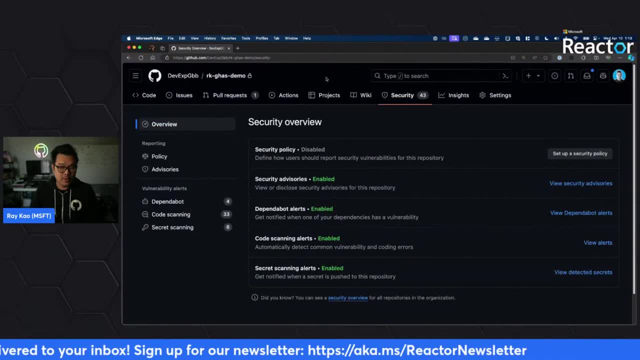 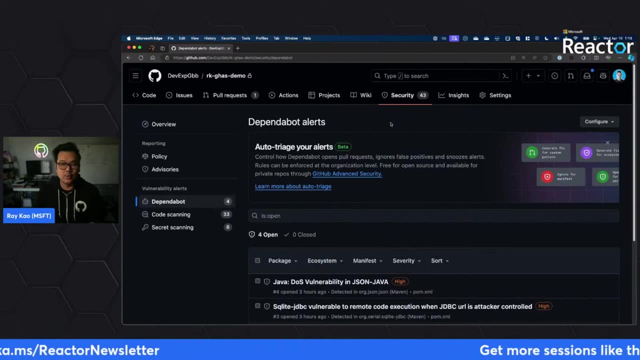 especially if you're running an open source repo, public repo, to turn that on as soon as possible. Same with Dependabot or your supply chain security tool. And so in this case here the UI is gonna be a little bit different in the sense that, if I go back to secret scanning, 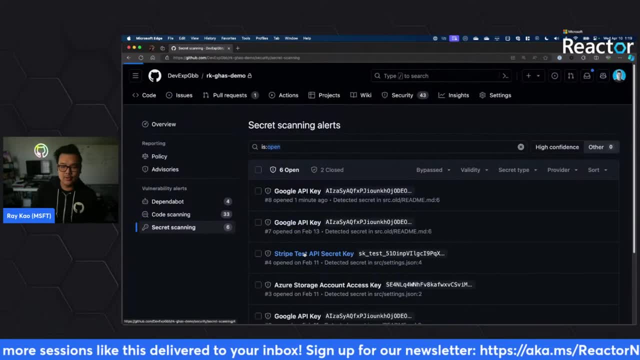 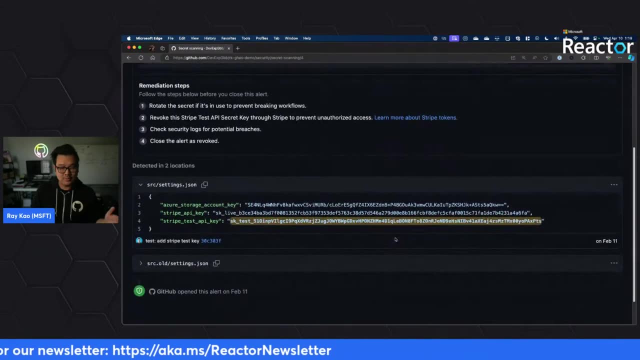 it's a little bit simpler because it's just talking about keys. I can actually click on the given key. Again, it gives you some details, what you can do to remediate it, where is the actual key being exposed, et cetera. 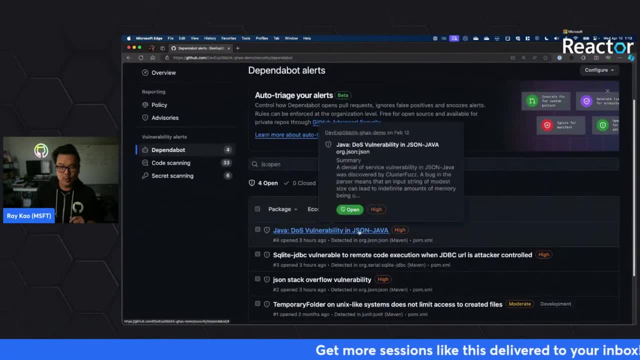 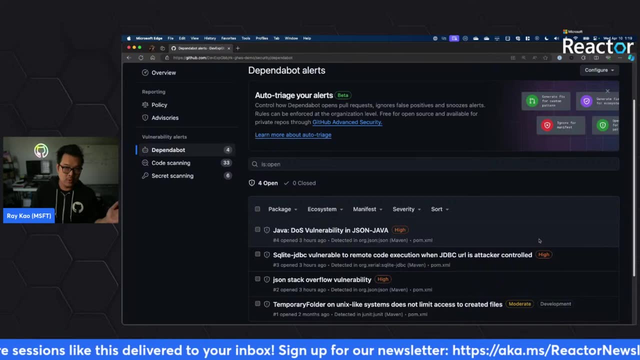 With Dependabot, kind of similar in that sense. but what I can do is I can actually again see the alert. Is it a critical or high? In secret scanning? it doesn't give you. you know how critical is that exposed key. 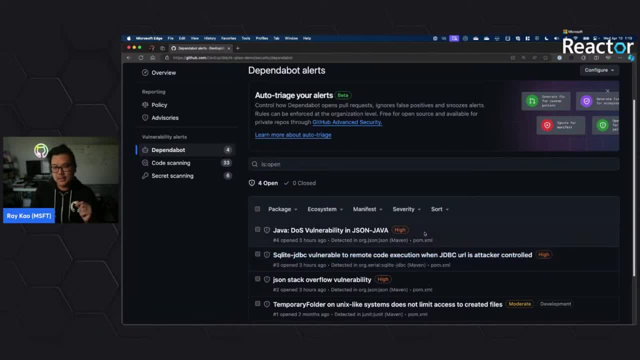 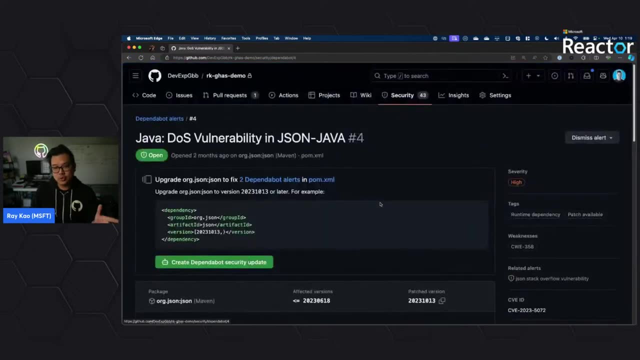 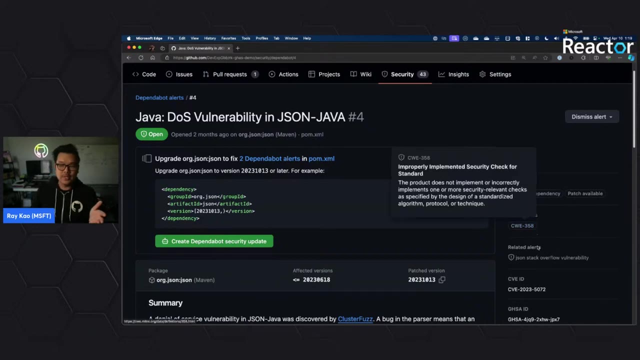 In dependency or your supply chain, or in code scanning. it does give you severity levels. So here's high and here's a moderate one. What I can do now. this provides me links to the given vulnerability or potential vulnerability. how high? what CWEs or CVEs is it related to? 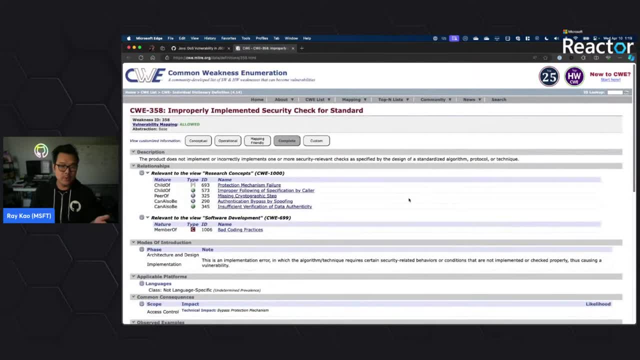 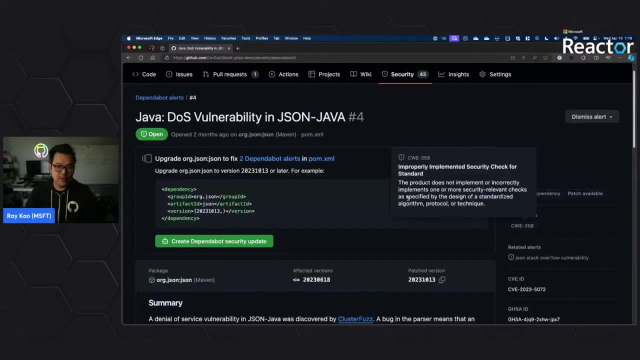 that I can look up and provide additional information. So I click on the CWE. This gives me information pops up. the new page from a common weakness enumeration database provides me information about it. Not only that, but within the portal here. 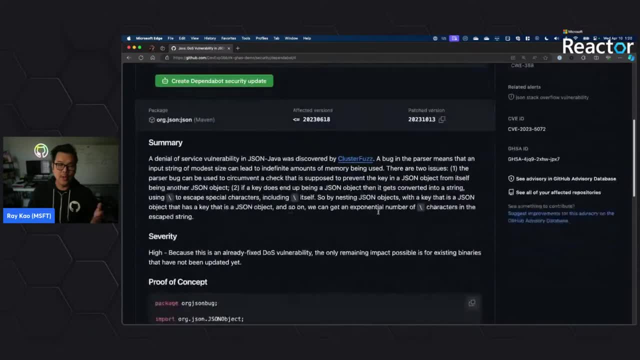 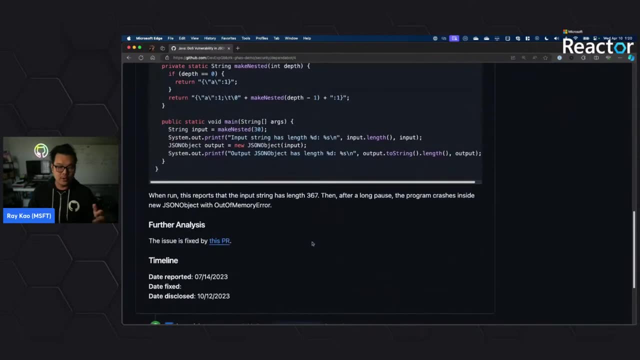 it also provides me a summary of like: what is this actually doing? How bad is it? the severity level, A proof of how bad it could be right, An example of where it could go wrong, And then you know further analysis and things like that. 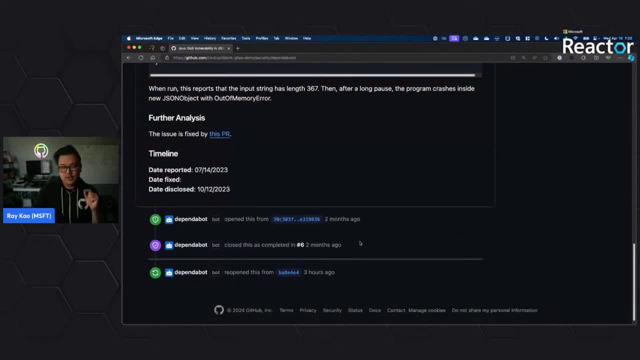 It can also- because I've run this a couple of times before- show you a history of how many times has this been exposed and in which previous commits was this done in, Because I could very easily reintroduce the exact same dependency problem, because maybe we push it. 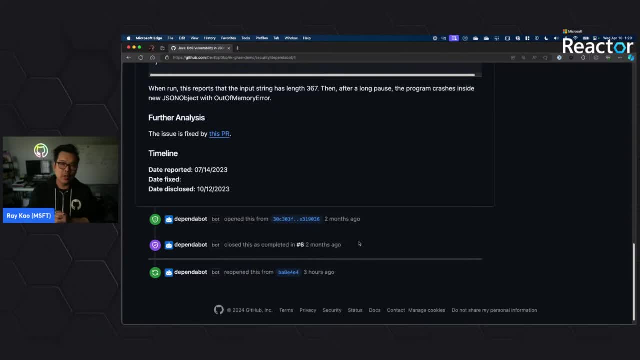 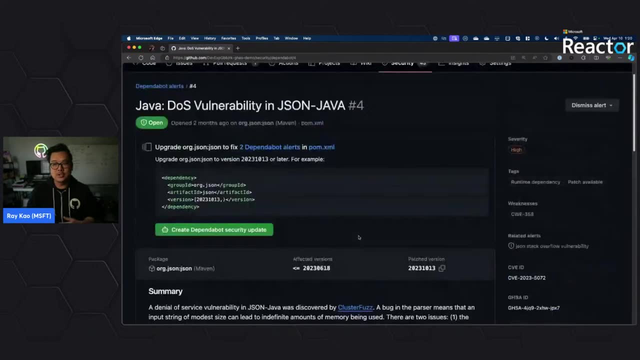 it commits, we're out of sync, or something like that. A number of things can happen when working in a distributed team, So this provides you with some of that as well, as well as the audit trail again to dismiss the alert. 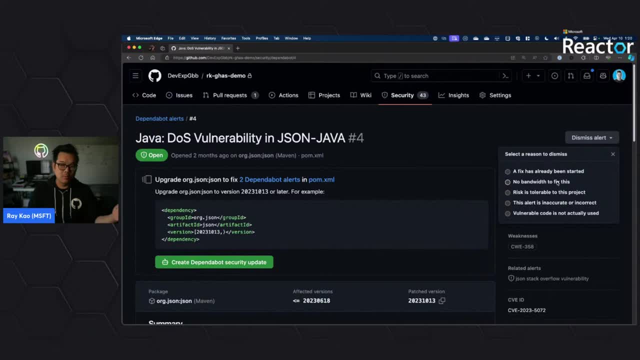 right. Maybe we dismissed it before and then it reappears again. Maybe it's actually not exposed publicly. It could be used only in testing and therefore it's not gonna be an issue in our production site. Number of reasons: So same thing in that sense. 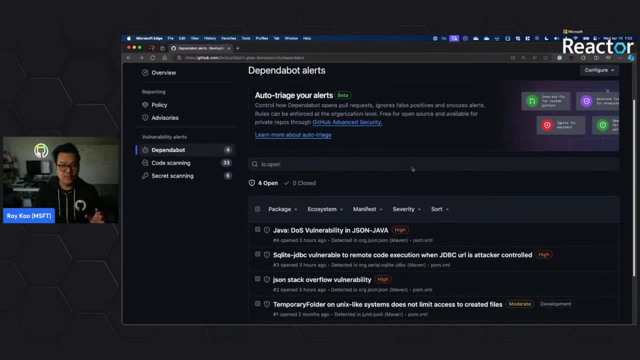 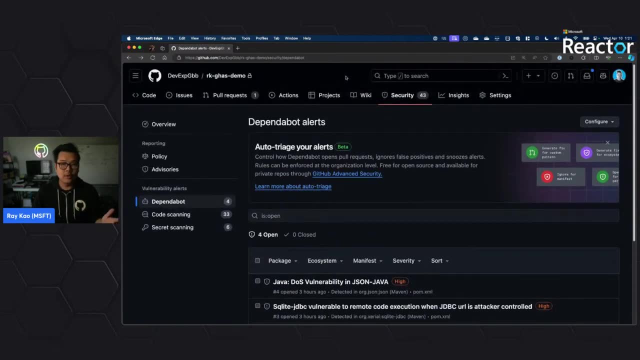 So Dependabot you turn it on, it's going to. it'll be actively scanning for and checking for this when we push commits. but, more importantly, you're likely working in a different Git flow where you have feature branches and you're gonna submit PRs. 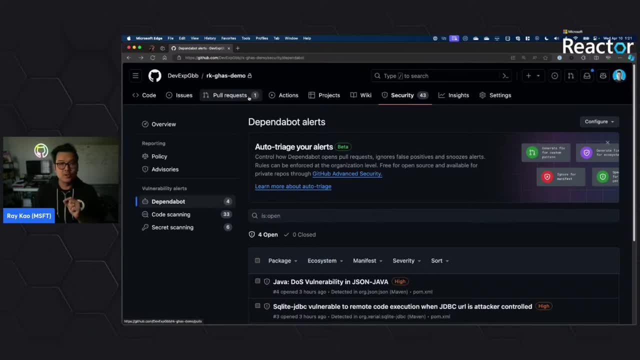 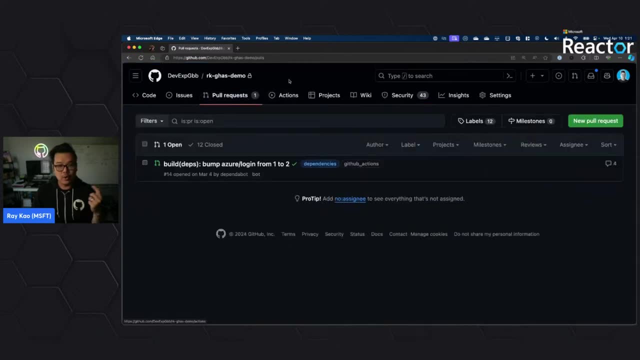 Similarly, there we go: instead of pushing directly to your main branch of your repository, you'll be pushing likely to a feature branch And, as a result, you'll probably be generating pull requests Well before we get to our own pull requests. 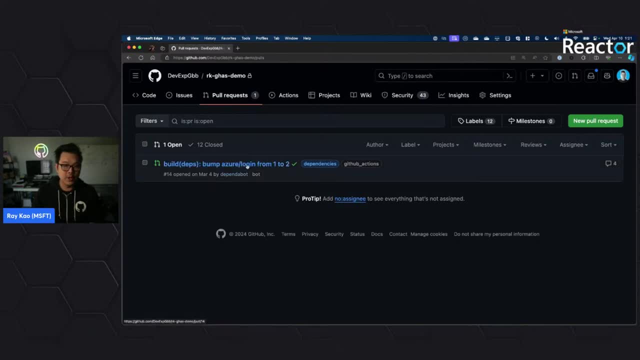 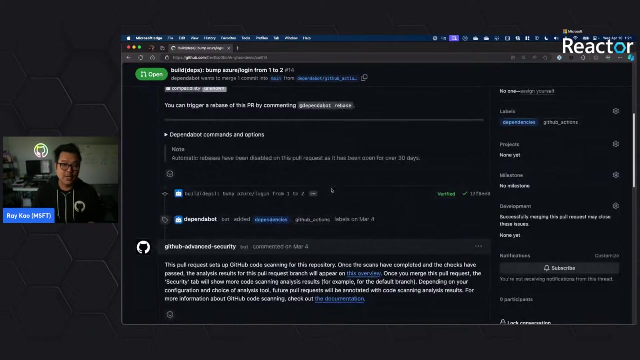 Dependabot can also generate its own based on what it's able to discern from our given flow pipeline, and it tries to, if you've turned it on, to submit PRs. that will actively help contribute back and make your code more secure. In this particular case, Dependabot is 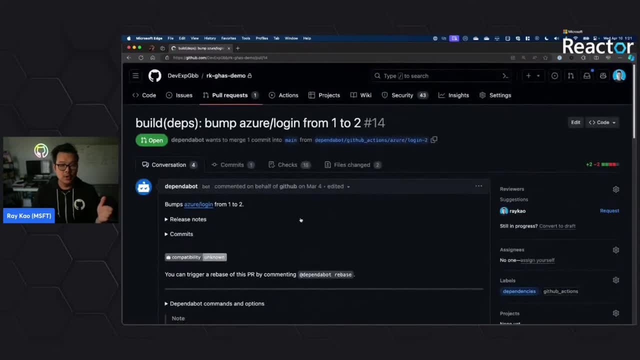 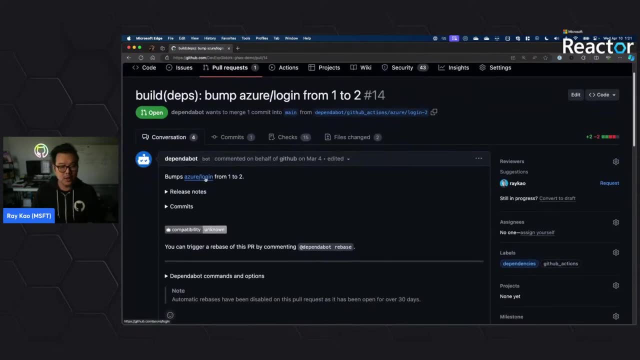 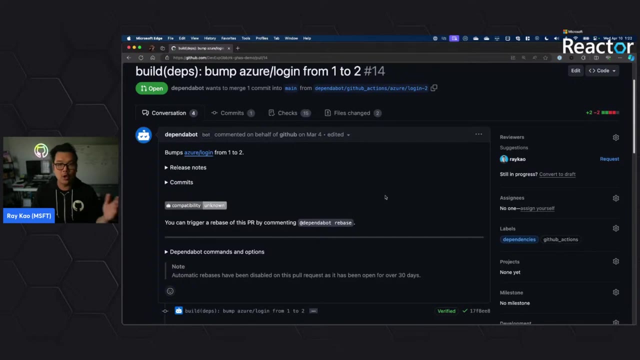 in GitHub Advanced Security is able to create an issue comment inline as to what the problem is, And in this case, in my actual GitHub actions pipeline, I'm actually using the example files that are used today, using an old or outdated version of the azure cli or azure login action, um, and it's suggesting that. 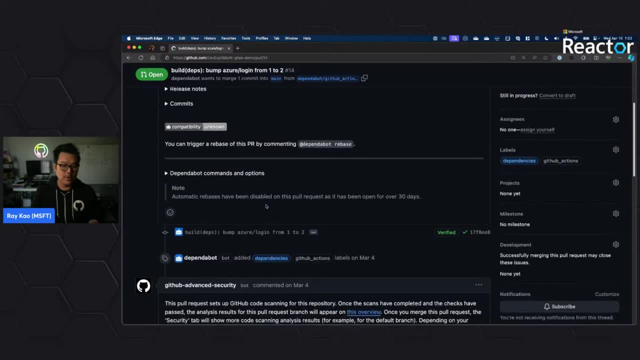 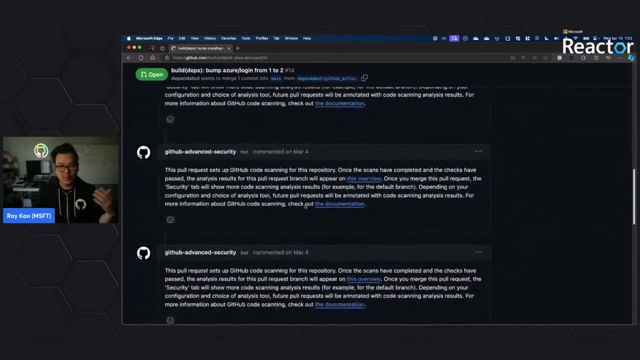 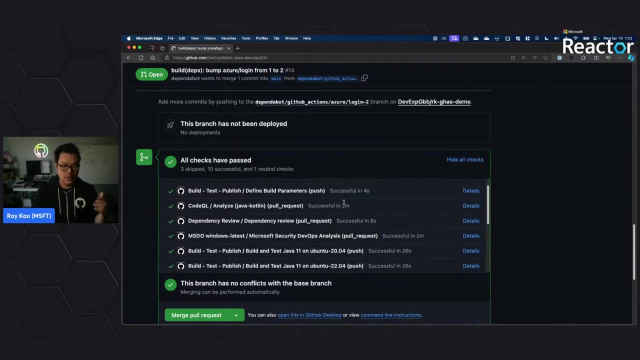 i bump it from version one to two. all right, so there are pilot issues about compatibility issues and other features here that um i should be aware of. it will provide you know what needs to be done, overview etc, etc. every time i push it into the repo it will check etc. so i can also have um as. 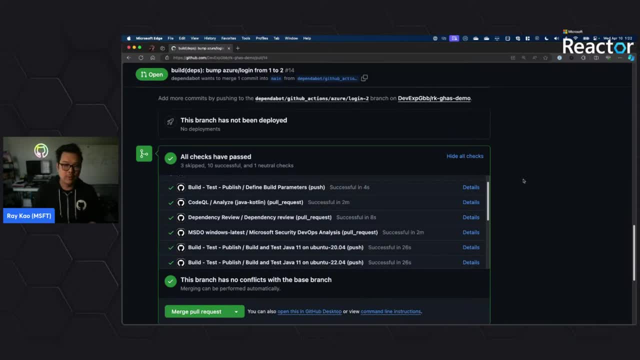 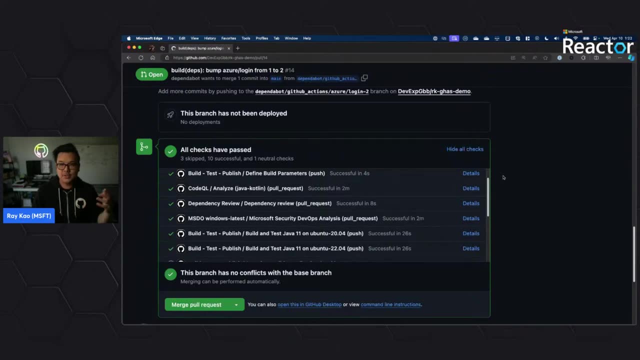 part of any good pr- and we'll see this later also with the code scanning portion of it- the ability to kick off as part of a pr, github, action, workflow, um, any additional tests as well, so it's not just depend about doing scanning my full. you know test suite can be run on a given pr. it could be included. 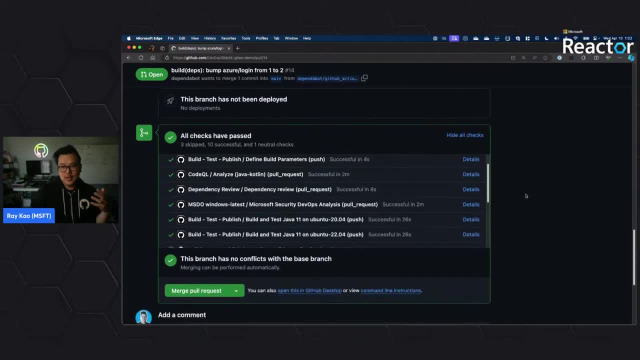 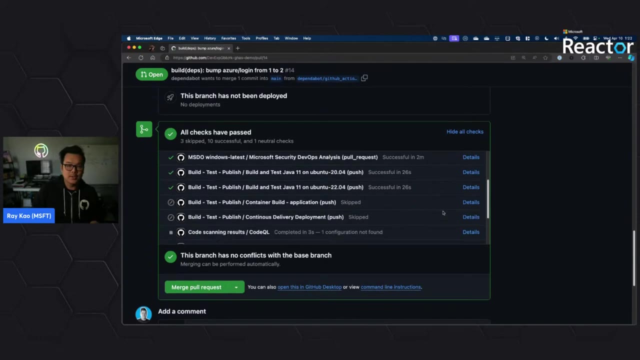 in here and gate uh this pr as well. so this way again, as part of your developer workflow, it's trying to do, um, some things for me, some of the undifferentiated heavy lifting, if you want to call it that, the boring tasks, right, things that i i don't necessarily enjoy as a developer, but are are critical, uh, to securing. 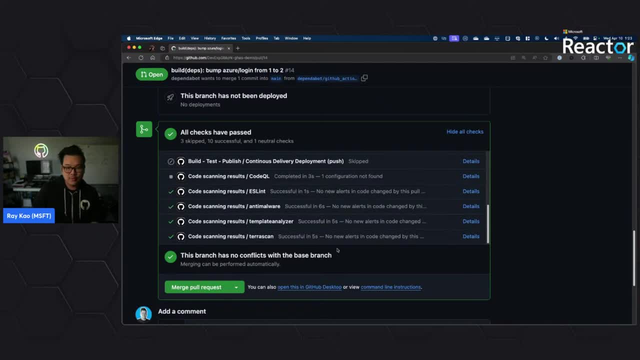 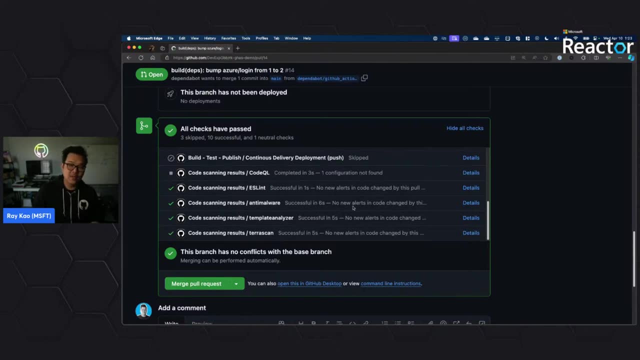 my software so again goes through the whole suite of things that we suggested to go through. we've got a green check mark. i could merge and pull, merge that, merge that, pull request. uh, in line here, just as i normally would with any other teammate or human being, but in this case it's. 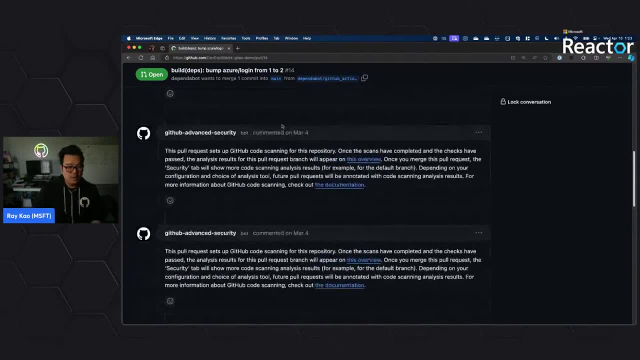 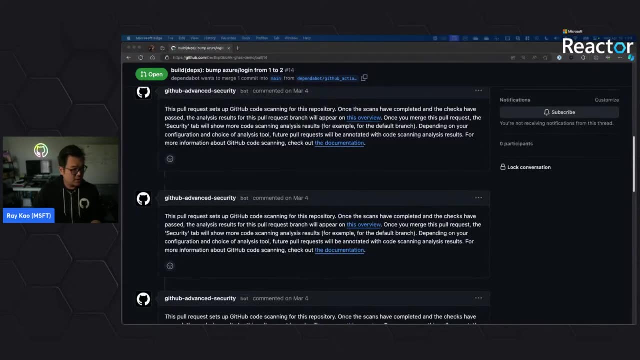 it's a dependent bot doing this, okay, so, uh, let me see here. uh, there's a question from the audience. how do we know that the pr generated by whoops- i didn't catch that quick enough- um, it's safe to be merged and it won't break the application. um, so that is where. 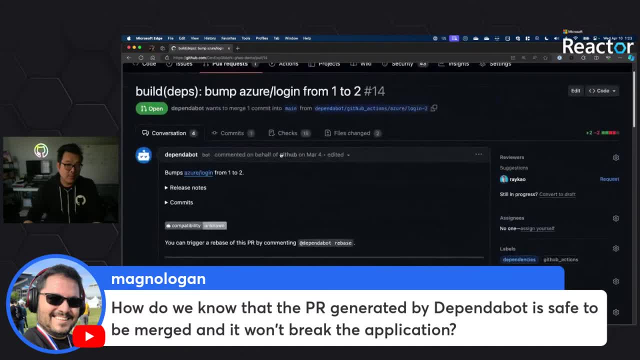 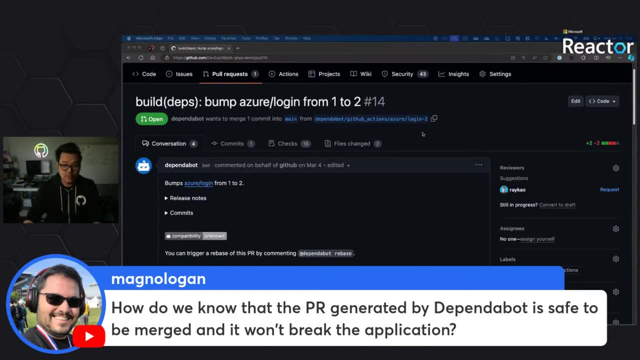 so great question. so the question is: um. how do we know that the pr that um dependent bot is suggesting or submitting won't actually break our application itself? so that is where all your test suites here in here, in terms of github actions, in terms of getting the green check marks and whatnot. 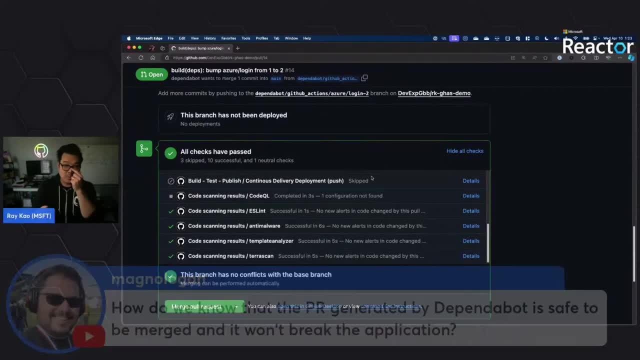 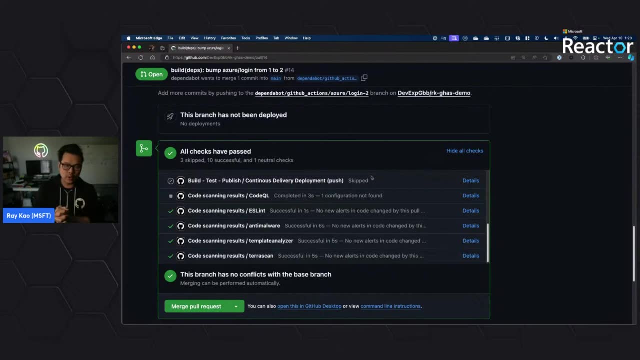 need should be in place. it's up to you in terms of how you build that out right. so this is all: your whole devops process, your um, your runners, cicd process, whatever you want to call it. ideally, this is just scanning your code, so this portion of it doesn't have integration tests. this is primarily unit tests. 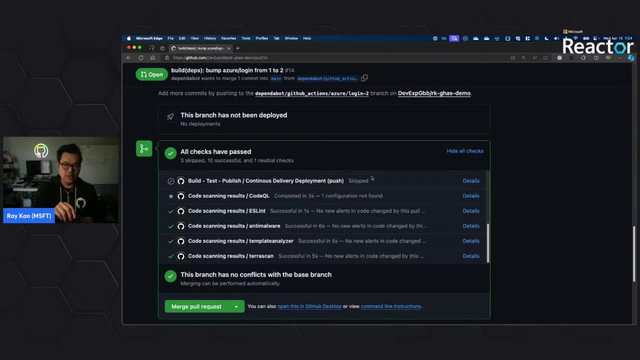 malware scanning, static code analysis, etc. whatever i've defined in my actions. there should be another step where you promote the code into a pre-production environment. it could be test environment, non-prod staging, whatever you name it- and that should have a suite of integration tests in there as well. as a result of that, they can manifest themselves in here as green check marks. 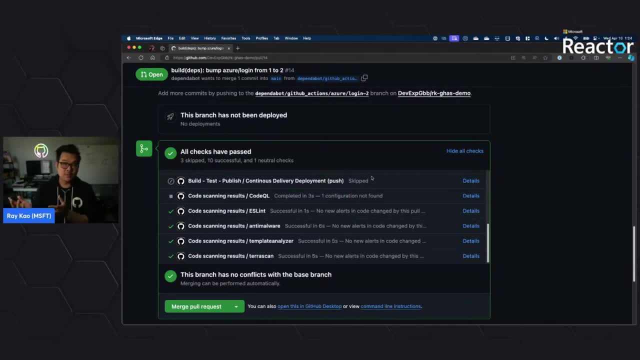 red x's right to say: did those tests pass in terms of integration? that itself would help to ensure the best coverage. there's no silver bullet, but the best coverage to ensure that the pr that dependent bot is submitting- or anyone for this matter- doesn't have to be a dependent bot, pr or 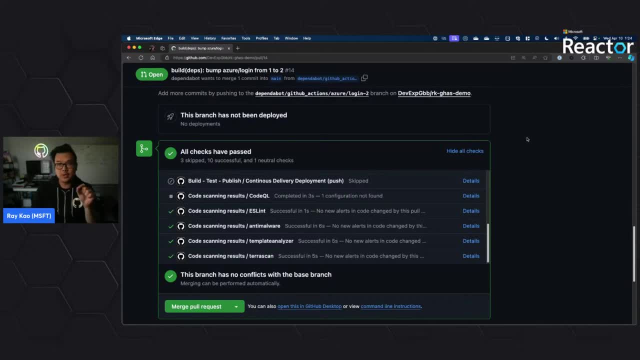 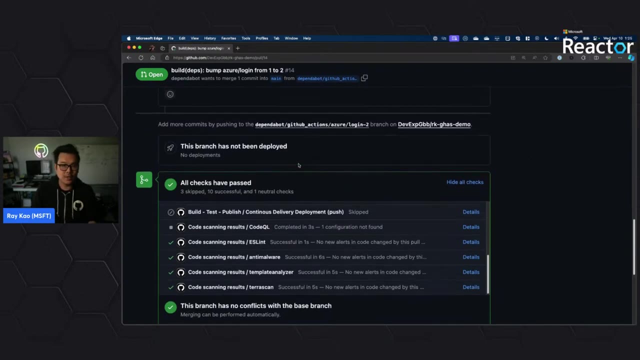 to run through this gauntlet. uh, doesn't break. you know, not just your application but your application as a whole ecosystem of apps, if you're especially running service oriented or you know microservices in your organization. so hopefully that is clear. we can, if not, put back into the chat and we'll. 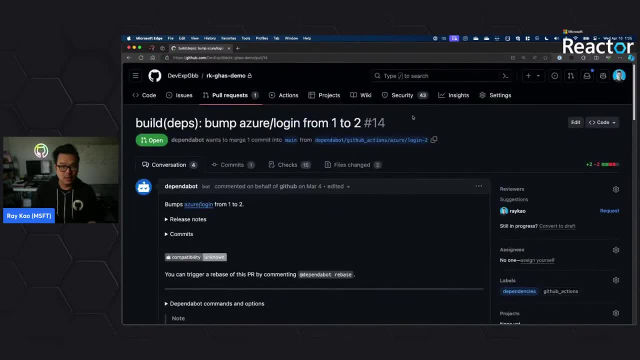 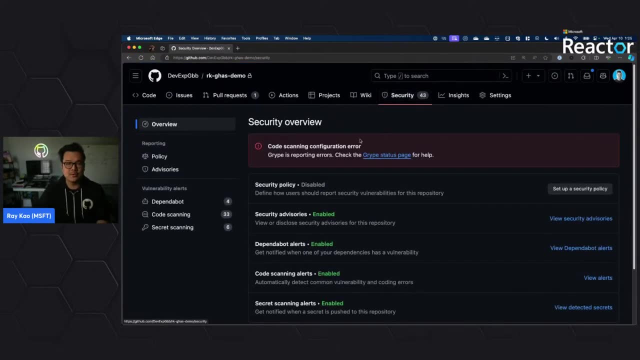 clarify a little further later on. all right, so, uh, i think that's what i wanted to show from a dependent bot perspective. um, the next thing and the- i think the bulk of the rest of this time will be primarily digging into uh, code scanning. um, mostly because the custom 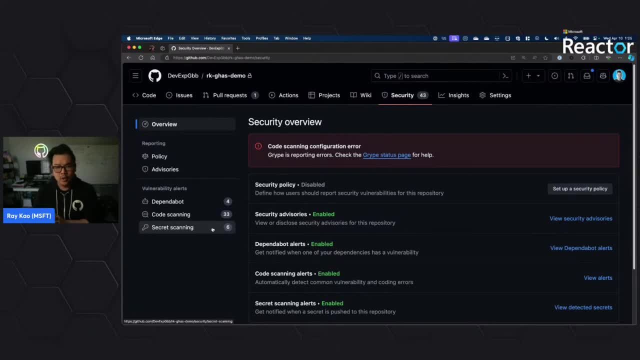 ization, um, which i won't dive too much in in there. code scanning is probably the most complex and the one that is uh more relevant to you directly, uh, in the sense that you know, uh, secrets are just hard-coded strings. you know nothing too fancy there. they are either live keys or they're. 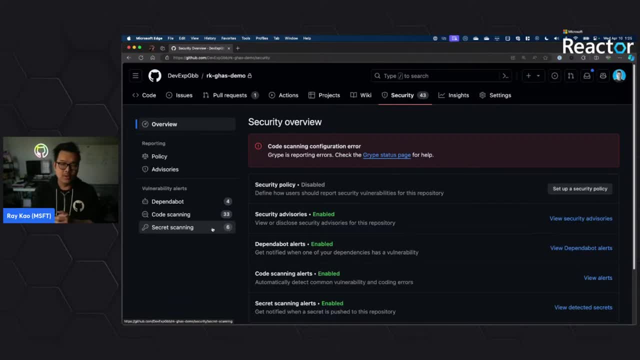 not. it just kind of warns you that it's there and do something about it. dependencies, you know, typically that's just bumping the version to a latest known secure version or to be aware, and then you can help to submit upstream prs to fix the issue that's been detected, if it hasn't already. 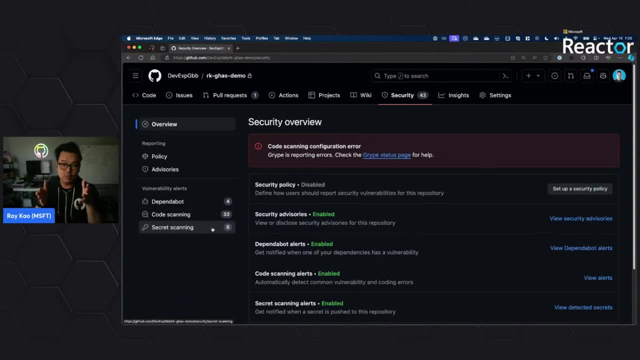 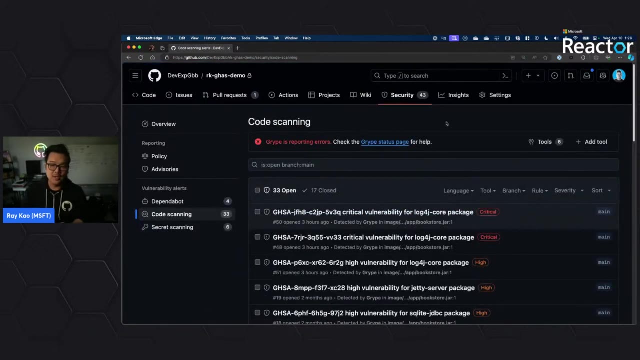 typically they have been uh. and then secret scanning is pertinent directly to your actual uh line of business application, your, your custom code itself. um, in my case, here i'm going to dive into secret scanning. sorry, uh, code scanning is the one i wanted to go into. i've got 33. 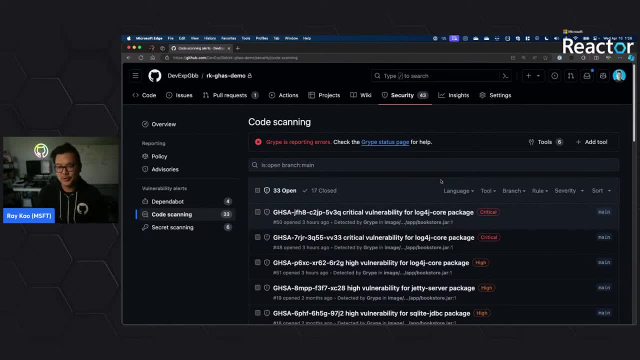 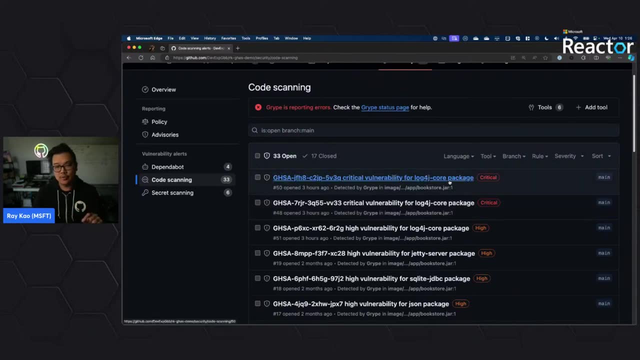 uh issues in here um all self-inflicted uh for the sake of a demo uh and, as you can see, uh they have different levels of severity. they've got additional information about what's um happening and they can actually come from other things other than codeql um, in this case, the top ones. 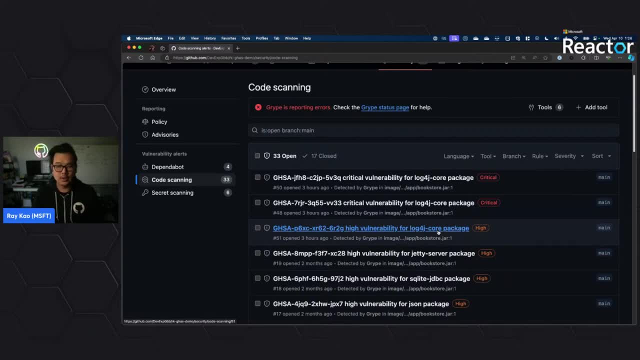 here are coming from another uh scanning tool, uh called gripe. uh uses anchor behind the scene or anchor and core. i'm always bad with pronunciation, but it's a container scanning tool. check for vulnerabilities within the container itself. um, so you can use essentially any additional scanning. 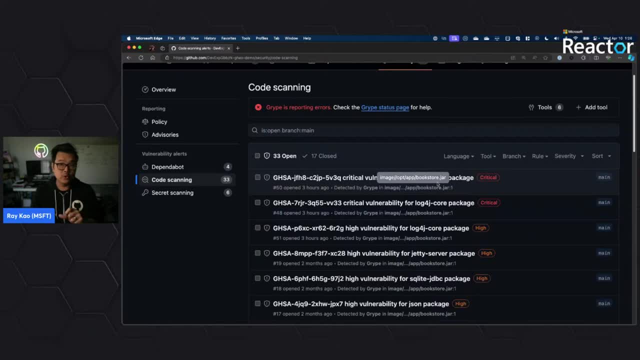 tools that you want. so you can use essentially any additional scanning tools that you want. the key thing is that that tool should output and generate a serif file, which is a particular file format, structure, syntax to generate security reporting such that github advanced security can. you can through actions in your pipeline or through the 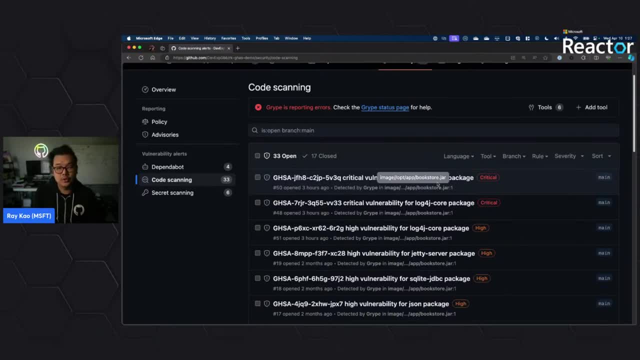 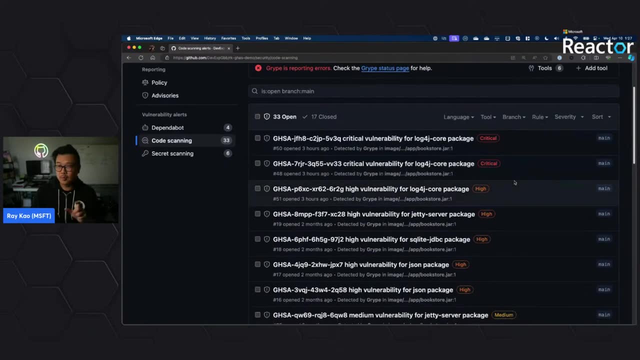 command line: upload the serif file to the github advanced security and then it will manifest themselves as alerts in this portal accordingly. uh, the other benefit- and just like a quick tan here- is that it's a little bit more intelligent in that sense if you're from the cyber security. 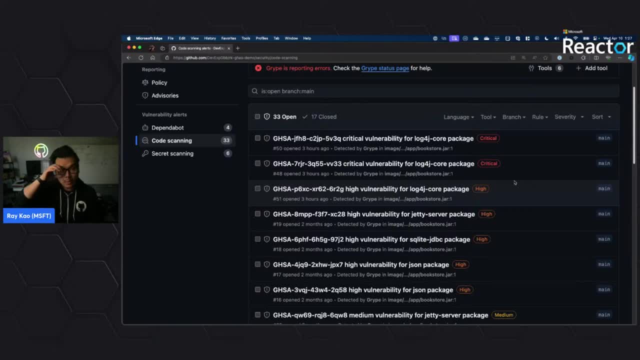 side of things, from the microsoft side of the house and use microsoft defender for cloud. there is an integration between uh defender for cloud, devops, security- if i haven't butchered the name for that product- the ability to read or basically export or extract from the same serif. 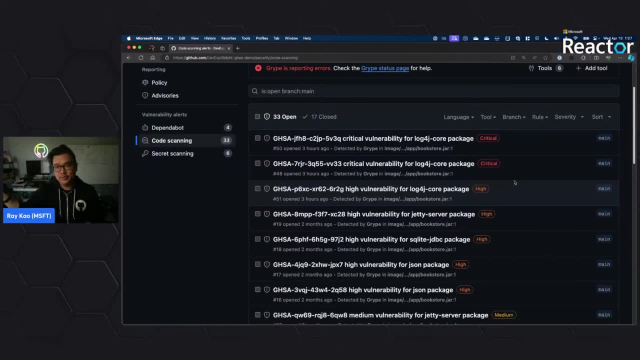 source that's stored in github advanced security and kind of report the same information inside microsoft defender for cloud. so if you're on the cyber team or security team or you want to call yourself on the uh sort of traditional uh github advanced security, you know you can just go to the 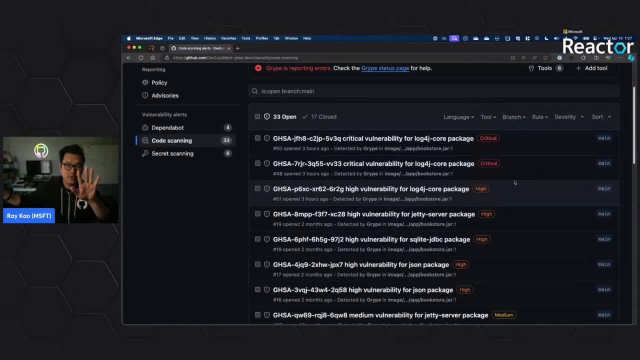 functional infrastructure side. right, but you want to be. no, you want to know or see information from the developer side, and you're not a developer. that is a great way to kind of have this ability to export the information and see the exact same thing that your developers see, and 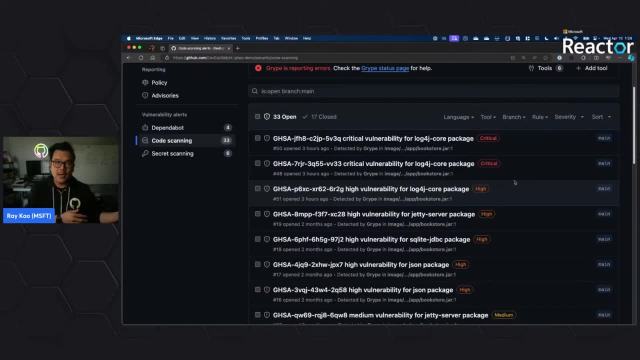 be able to essentially submit a pr back into github for a developer to remediate that issue, and that you as a analyst don't have to deal with, but there's a way for you to report, etc. all right, that was my small tension there, so what you're going to see here is i've 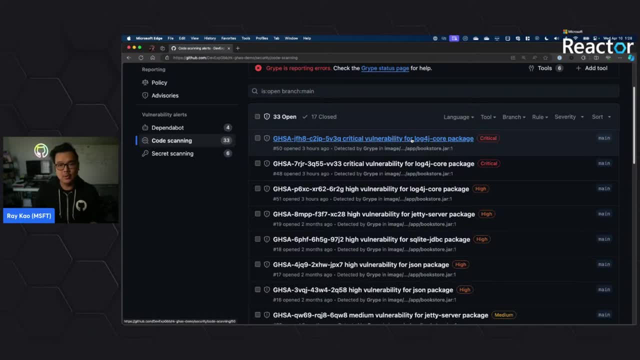 intentionally informed you by this, but if you're not a developer and you're not using your own real infrastructure or you're using a server or a github application, you just have to execute the. I reflected a log4j vulnerability into this demo. I wrote code that used an older version. 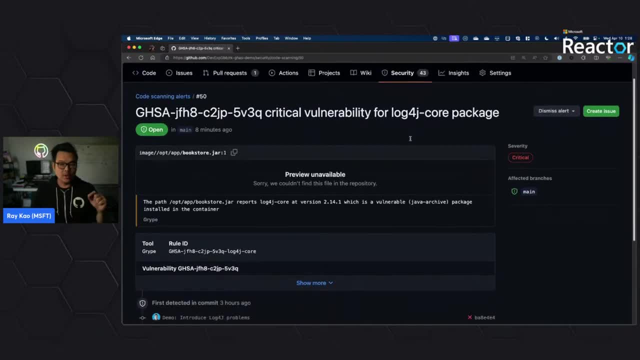 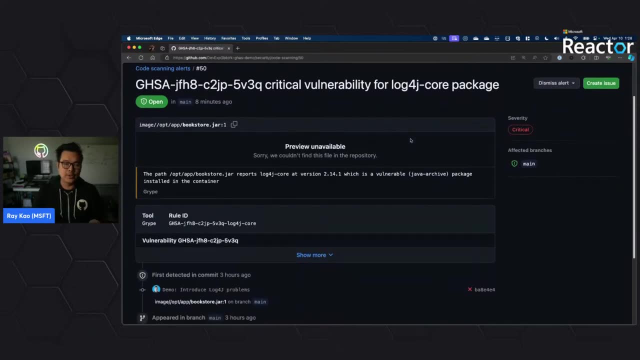 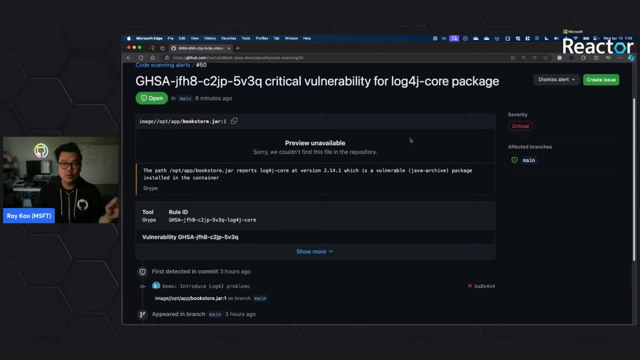 Oh, spoiler alert, I used an older version intentionally And this particular tool was able to detect it in the built container itself. There's gonna be an alert later on in that list of things that shows the version of it that was generated by CodeQL as well. 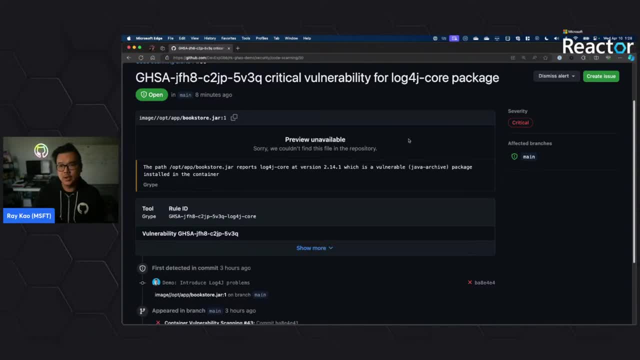 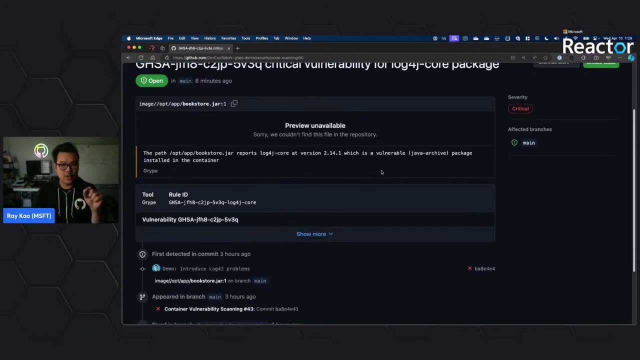 Out of the box using the CodeQL model packs, or QL packs that we call them behind the scenes that get run default as a suite for a given language. But this in particular is going to generate- okay, what is the vulnerability that we created? 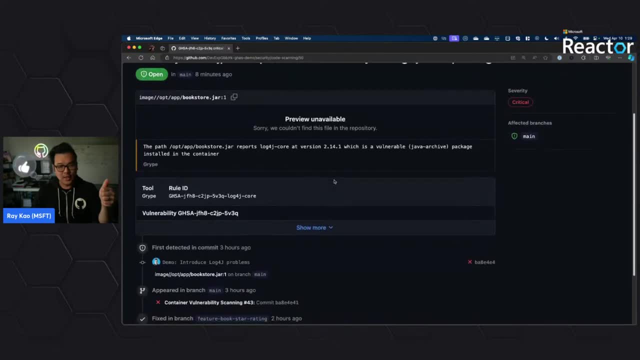 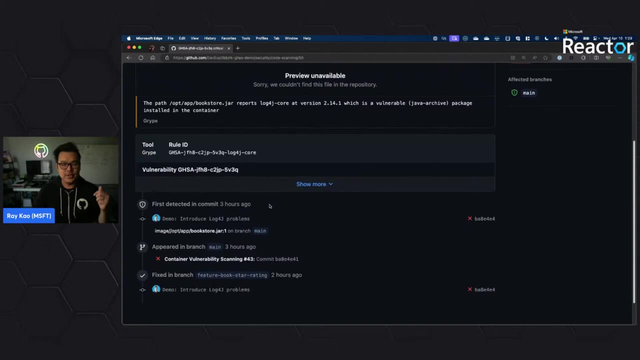 You know, is this related to potentially a CVE or what is it? And this is typically information that is derived from the serif file that this given task generated. We'll also be able to see when the particular issue was created, the vulnerability, the commit. 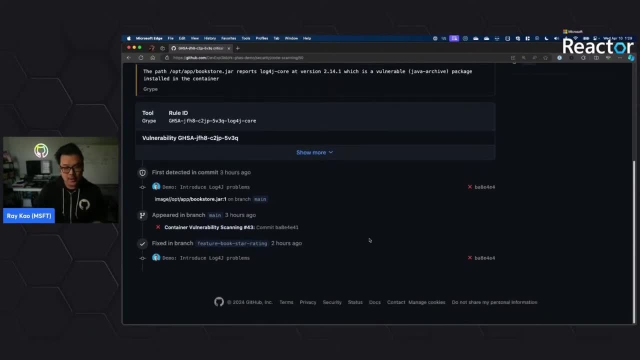 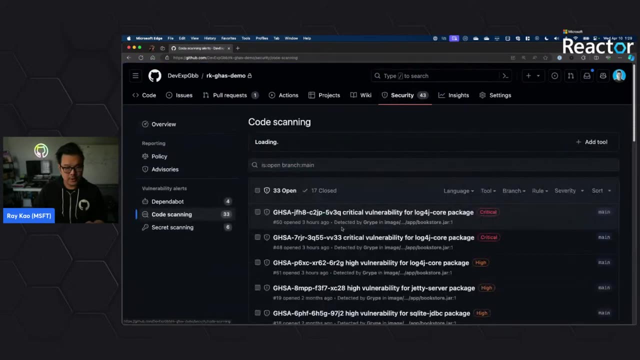 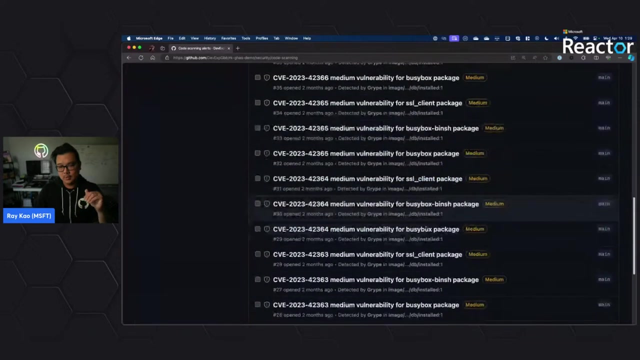 and which branch it was done on. Okay, so that's this in terms of the view. Let's go to code scanning again And then you can see again. there are a number of different, many different issues in here. Could be solved with a few, but we can go through them. 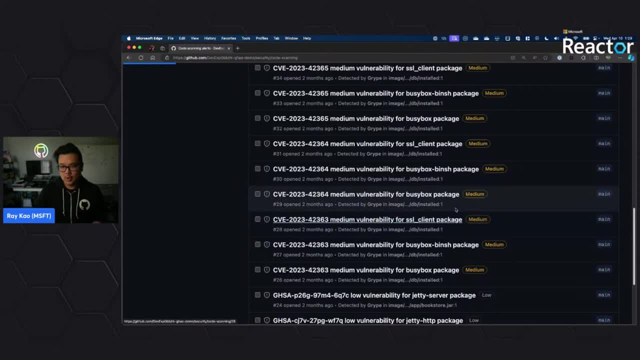 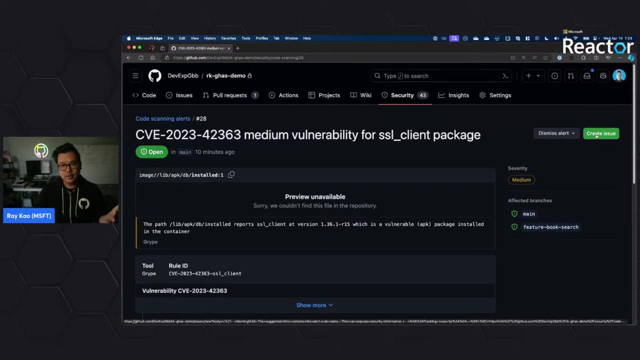 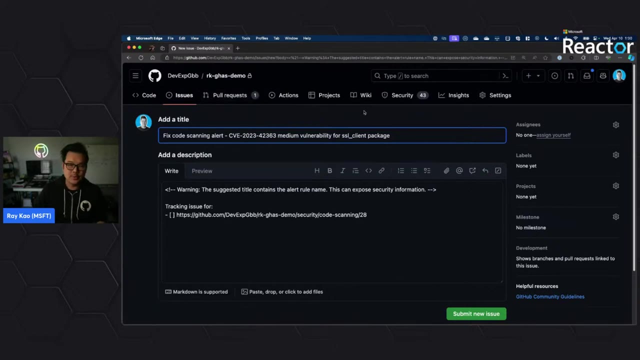 and kind of burn through them. What do they want to show? Oh, one thing I forgot to mention is that I can actually generate an issue off this alert right away, So I can create an issue. It can get created and put into GitHub issues itself. 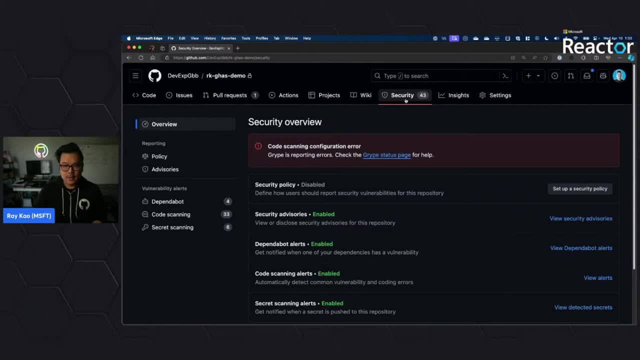 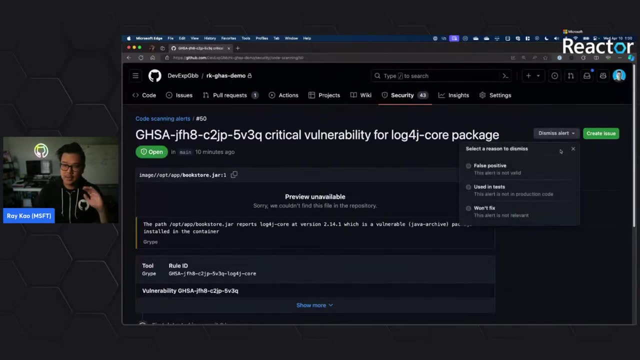 and I can start burning down accordingly. And, more importantly, if I go into code scanning again, just pick any one of these same thing as before, I can decide to say, hey, this security alert isn't that big of a deal. 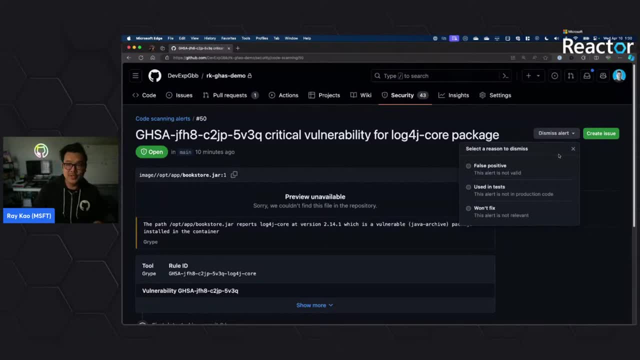 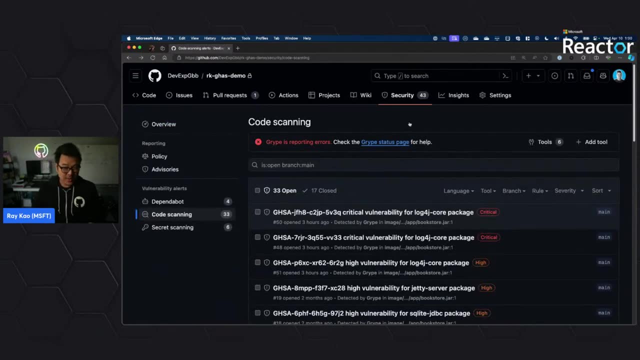 um, probably it is, if it's saying it's critical, but again, it could be in an environment that's not production and, uh, you can generate essentially an audit trail accordingly for this, okay. um, so, with code scanning, i want to want to move on. uh, for the sake of time, i want to make sure to leave. 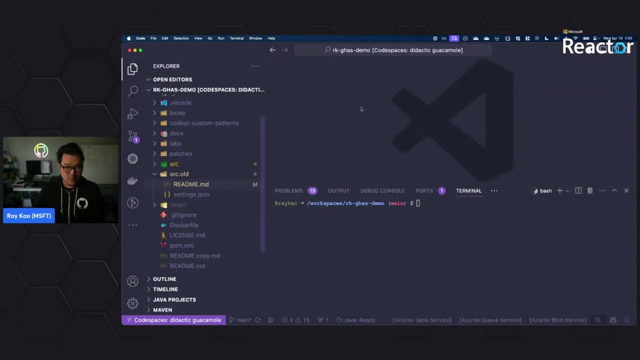 time for additional questions. uh, i am going to uh just run a task here to um generate a feature here. um, because they want to watch me write code, uh, during this time and session i've created. so what happened is i ran a vs code task that automatically wrote um code for me. thank you. 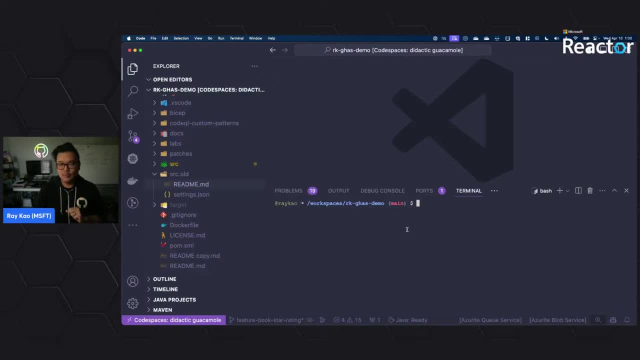 again peter murray and team um that created a vulnerability. essentially it's an unsanitized parameter that's coming in from a user and then it is going to be used in a sql query. so in theory, i've introduced a sql injection vulnerability in my application. 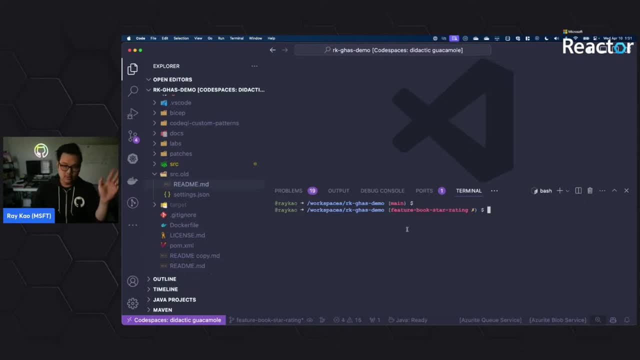 what i'm going to do now. so, just to show you um, that automatic script uh created a branch, added the vulnerability, and now i'm on a new branch and what i'm going to do is, uh, i'm just going to add everything. um, actually, before i do that, i'll show you um from what i 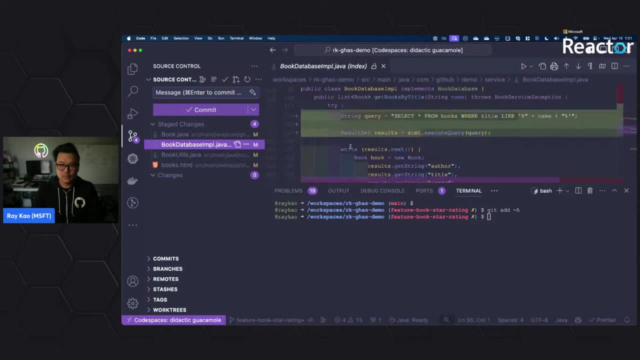 believe is: uh, uh, here, um, this is part of the vulnerability that was kind of generated in in the code, right? so it just concatenates and adds the string that was passed in um and queries the database directly. so i'm going to do is commit now, uh, demo. 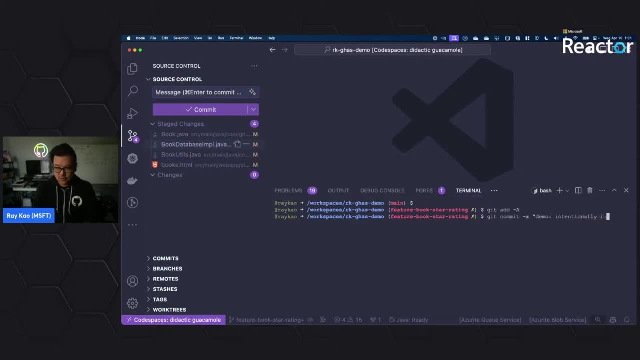 intentionally, if i spell that correctly, introduce sql injection. you wouldn't know this in advance, of course. right, this is just for me, so i can look back at my git history later on when i uh try to fix this um, and then i'm going to push this up to: 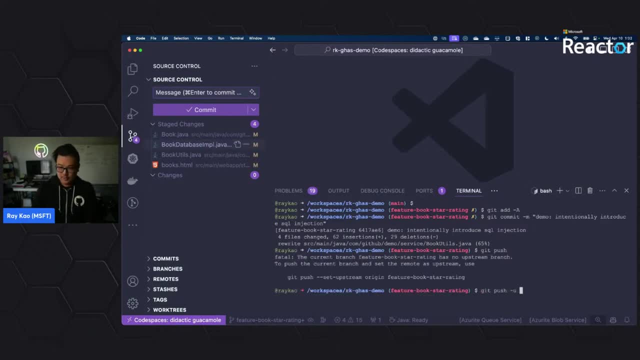 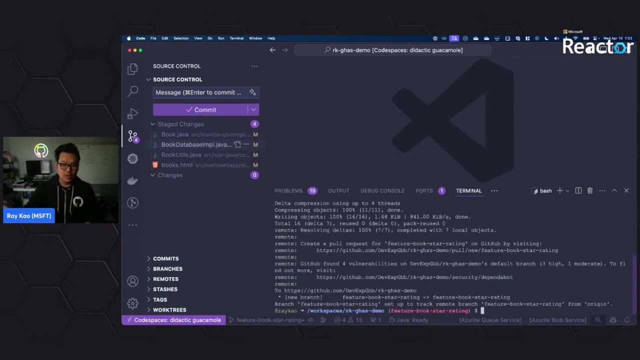 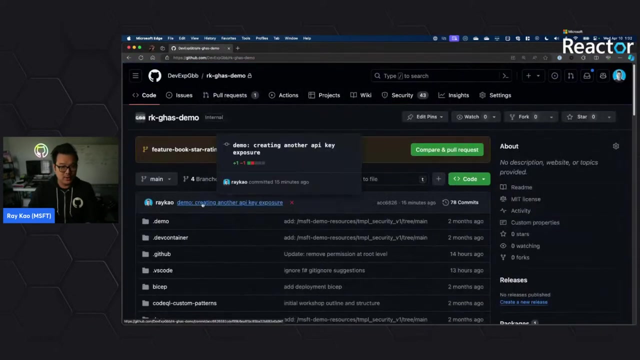 my repo, oops, because i haven't upstream or region or region feature. oh great, sorry. so that's gonna push my new branch up to, uh, my, my repo. so up here you'll notice that you know, demo create a well, nope, so here, uh, create a new. 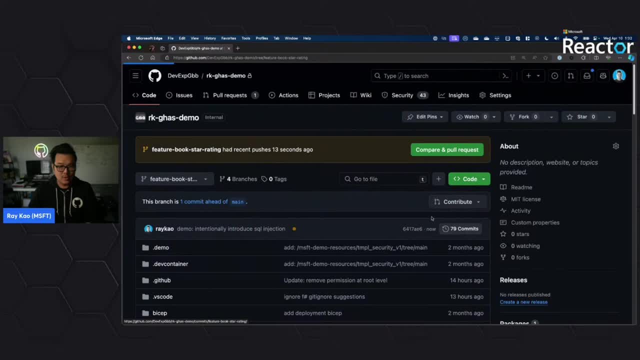 branch that itself will have a new commit, which is the demo, intentionally introduce the sql injection. what you're also going to see is: automatically this is kicked off because i've already created github action based on um a push to my repo on that branch, it's automatically started up actions or my cicd process. 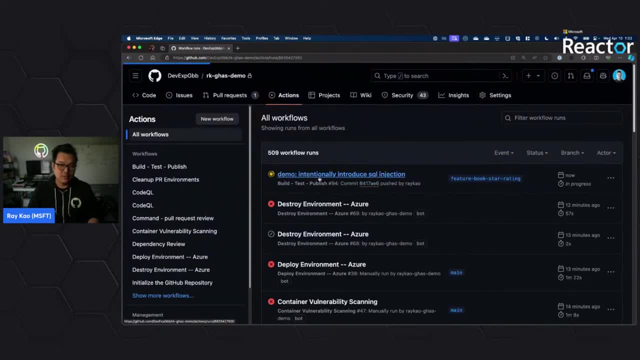 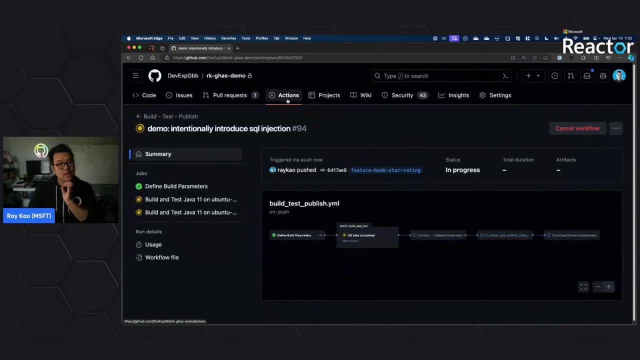 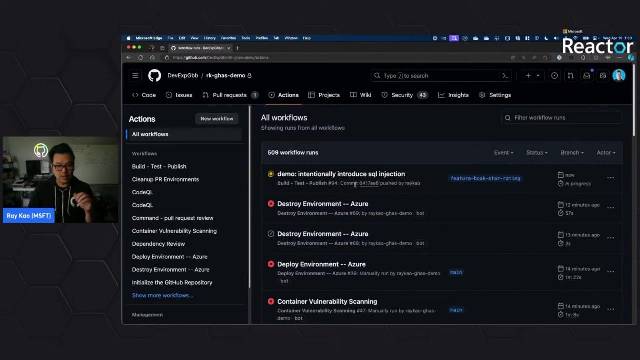 so it's going to start this build process here. it's going to run through the jobs, it's going to run through scanning and all that good stuff behind the scenes. um, i'm going to let that percolate. you know, depending on the runner, that's going on. um, it will run. it'll come back to say: did it pass? did the build itself fail? and it'll. 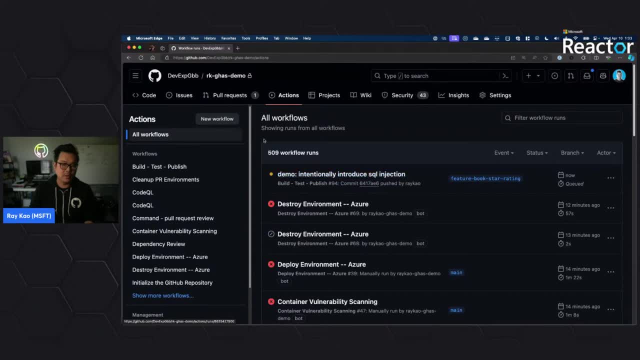 also upload at the end of that whole build uh suite, along with all the other workflows that are running at any given time: um, uh, the reporting for um for the security center, and then i'll remediate that in a sec. um, for, while that's percolating, i'm going to go back over here. 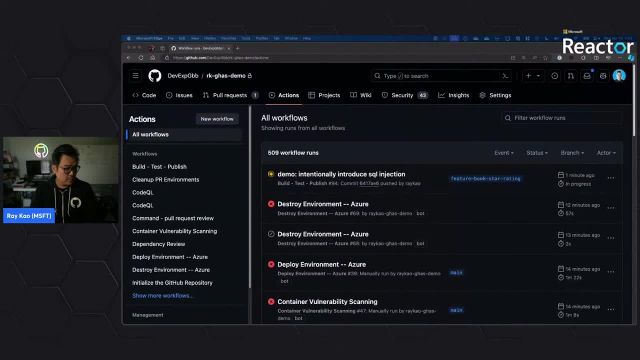 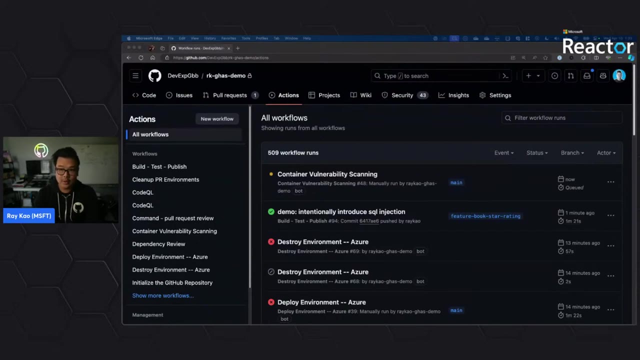 and just to check the comments: um will code scanning be able to generate prs to fix bugs in the future, just like dependent bot does? uh, yes, so that that is um on on the roadmap there. uh, that's going to be in combination with, like copilot and enterprise. 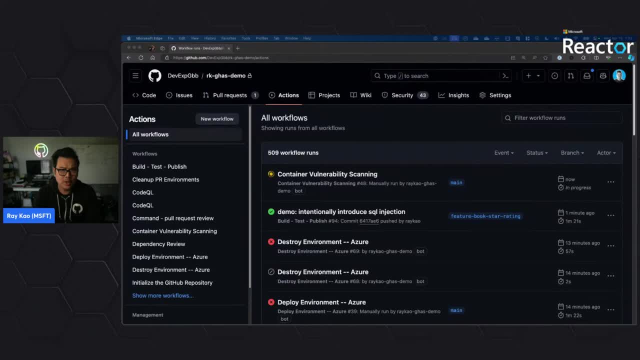 features in there. um, i believe there's probably a you know scheduled future conversation around this, but, um, yes, uh, that is going to be one of the um uh features in the future. uh, another question: are there web hooks we can use to build integrations, just as github apps, with these features? um, so, 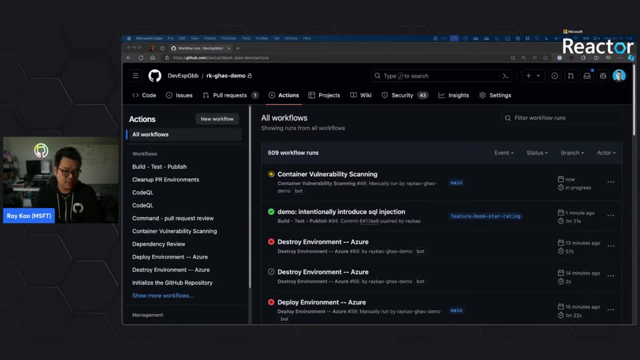 there. you can access the information via the apis. i'm curious in terms of what web hooks you're looking for in terms of building integration. um, can you basically emit, uh, can you admit that the alert has occurred and like read off of it from like an event hub or service bus or? 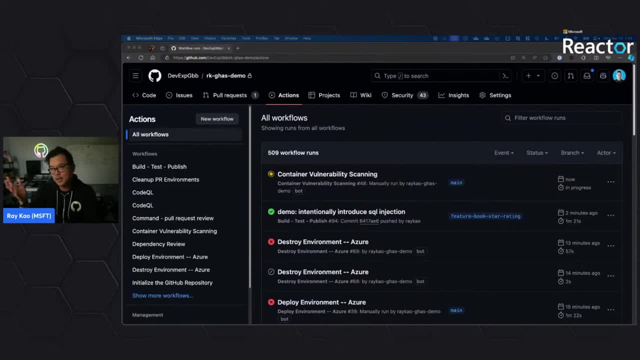 you know, push that itself in your case. here, webhooks are probably like event grid: um yep, but there's a whole api around that. uh that you can, you know, create your own workflows to remediate things, send an email, etc. uh, should those alerts occur, pop up as they go, so yep. 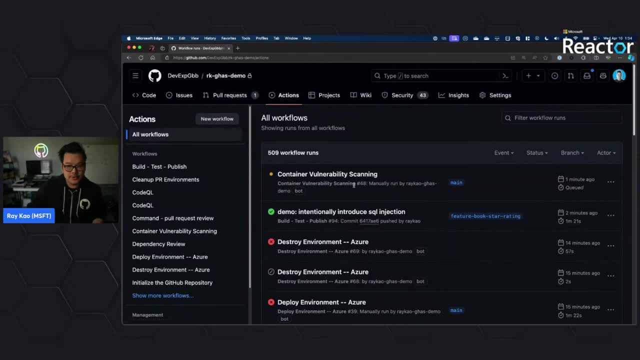 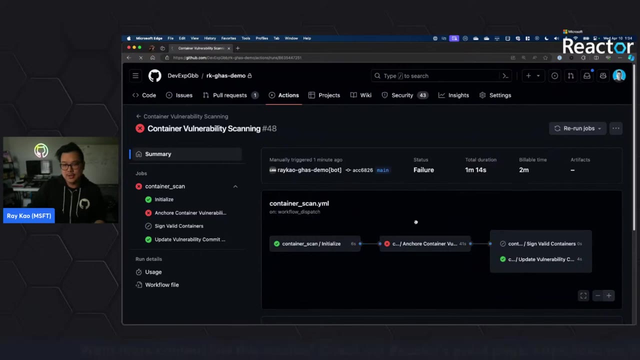 totally take advantage of it. um, so this is still going. you notice that i built the actual application itself. there's container availability scanning, which is the uh, gripe, um, or anchor anchor tool, and scenes. you notice that it's going to have an issue. it's going to stall out here because 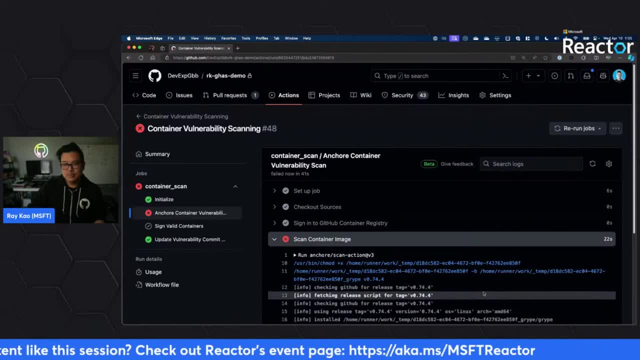 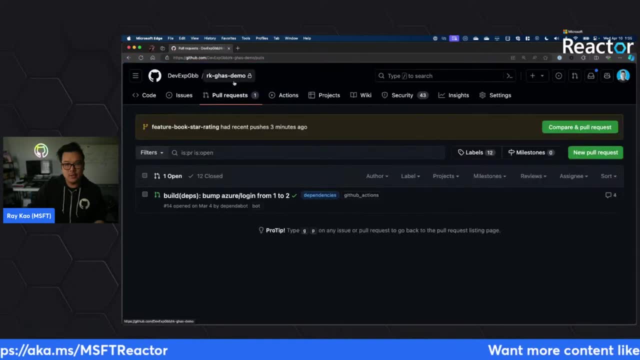 during this. it does a scan, it knows that the container scan itself was bad and it stops that process and it's going to report back and have issues and what we can do in a second here is that was as part of push, so you should fix and remediate that. what i'm going 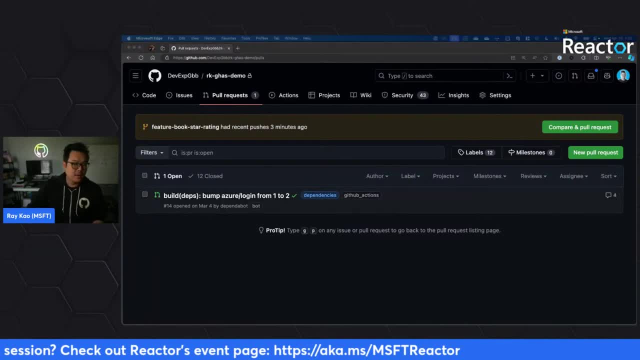 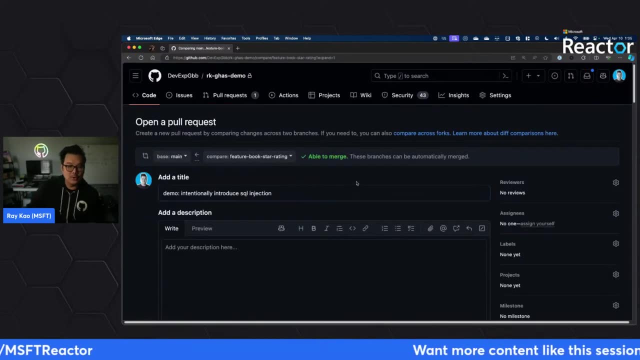 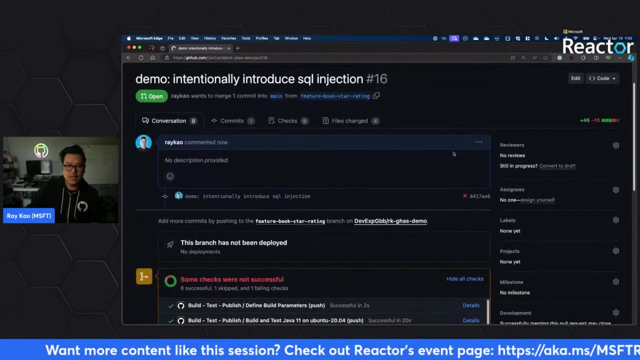 to do is assume that, oh, you know, my, my, uh, commit and push. look good, i'm going to actually hit a pull request, even though i didn't fix it. i'm going to here hit create pull request and you're going to notice that on a pr there's a whole pipeline of things that are going to run. 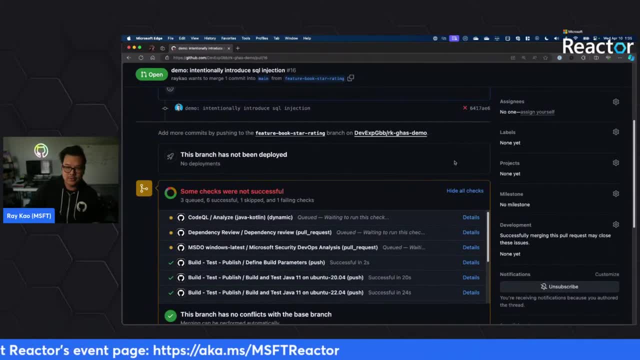 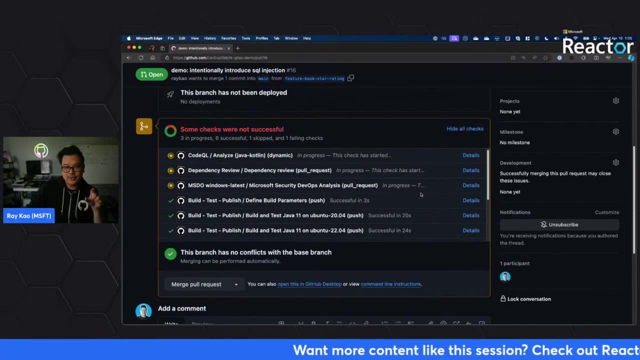 as well. much similar to what the commit uh was doing itself or the the push uh to my repository on that given branch. same thing happens on a pr. what you're going to be able to see is, instead of going through action and seeing it there, or you know, the indicator status indicator on that given commit, we can actually 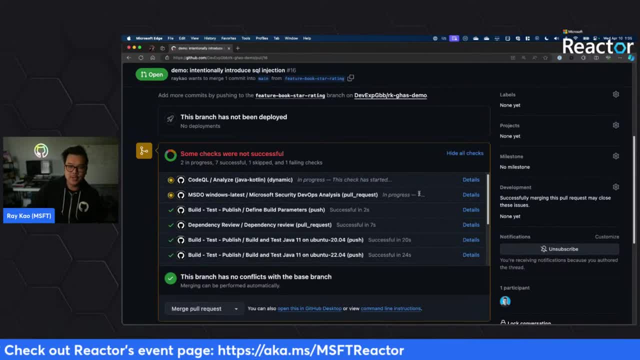 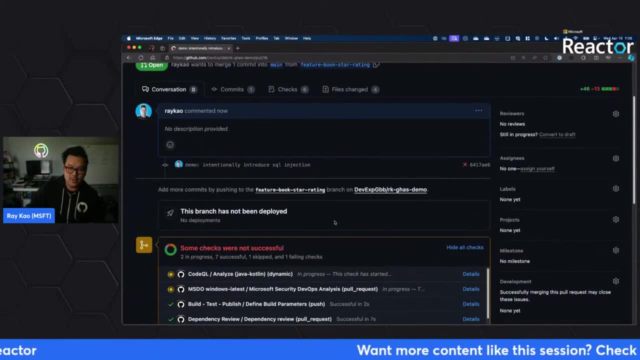 see the full uh rerun and build of this particular um test suite. let's call it in line with the actual pr itself and in a moment, um, once this percolates uh based on time uh, we'll see in line here as well that github advanced security is going to add a comment um, i believe just above. 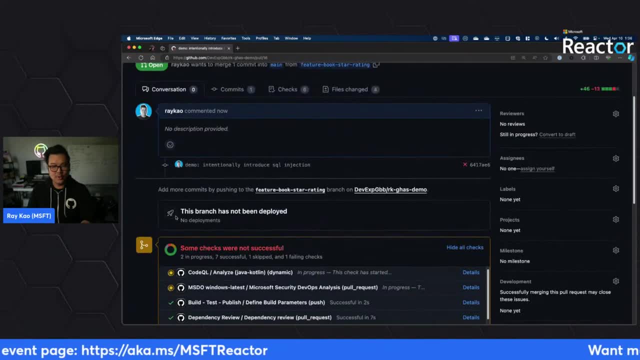 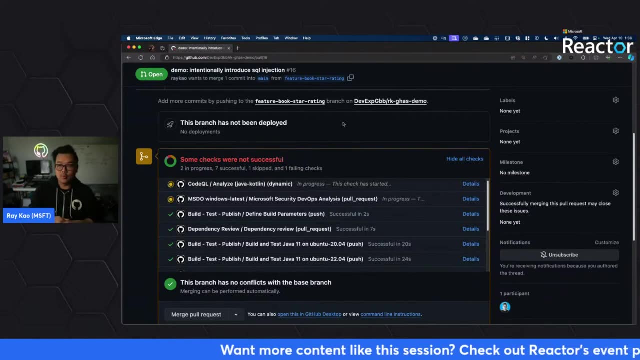 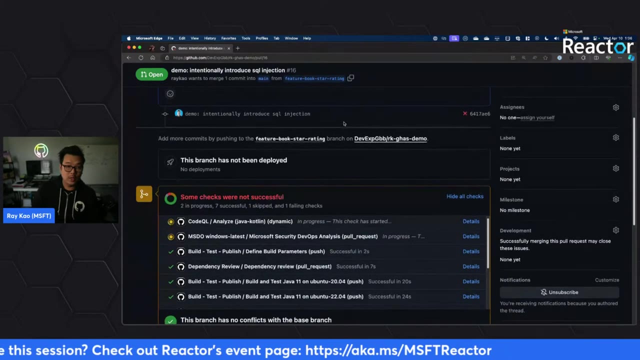 what we see in terms of the ui here, in terms of the test flow right above here, um it should, or maybe below um it will. it'll come up and say: hey, you know, here's what we've noticed, here's the cve that it's related to. you'll, you'll want to fix it? uh, accordingly, um, and so, uh, the next step after. 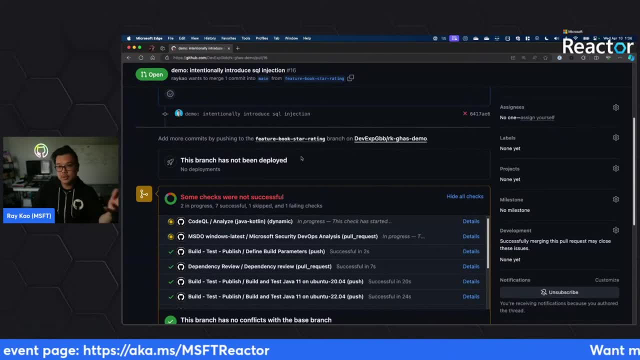 that, once that goes, is to actually show and demonstrate. you know, let's go through the process of uh, remediating that, um, the, in our case, um spoiler alert. all we're going to do is bump the version of log4j and our jetty version up to a newer one to protect us and 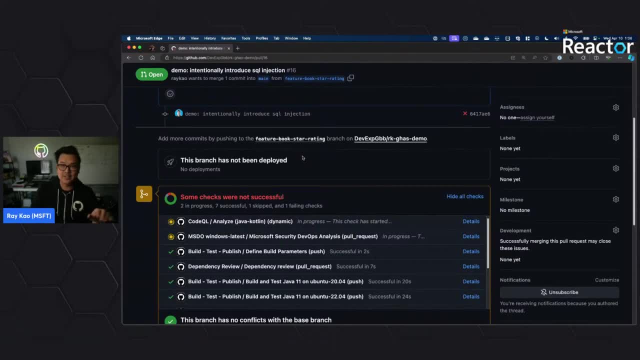 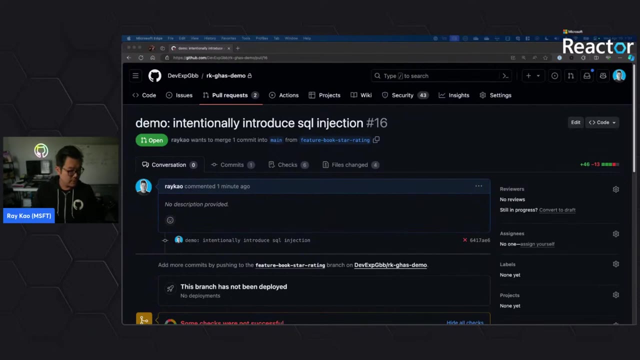 also to remove that sql injection, sanitize it and put it through a um proper, proper method to actually run the query. all right, so let that percolate. i want to check back again for questions. looks like they're, uh. will code scanning generate pr's? fix it all right? answer that? so yeah, uh, code. 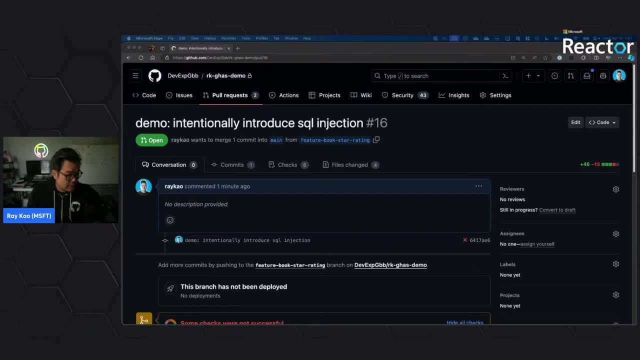 scanning will feature: have pr. what are the links? the api documentation for bowling alerts about code scanning? um, don't have that immediately available in terms of the documentation, but a quick search online will provide. if you github rest api, um, it'll, it'll give you. uh, what's there? 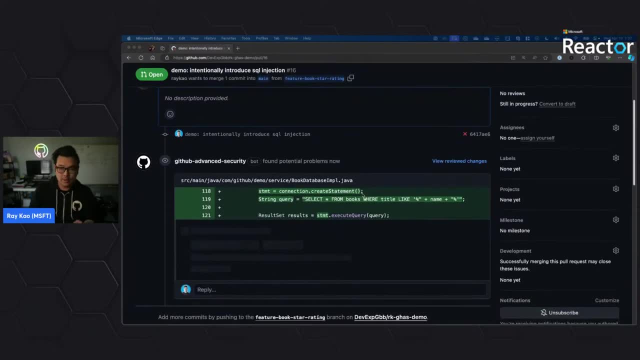 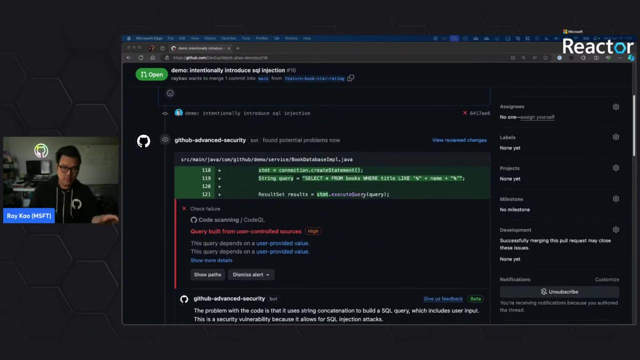 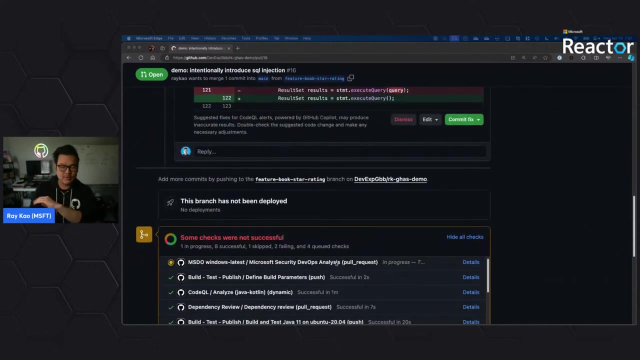 okay, paint has dried somewhat, still generating the full inline comments it, but you notice that um get advanced security scanned through it. as ran through the pipeline, uh uploaded the serif file. um, it's probably still percolating on some of the jobs down here. this is the msd01, the microsoft defender for cloud. um uh plug-in, uh extension app, whatever you want. 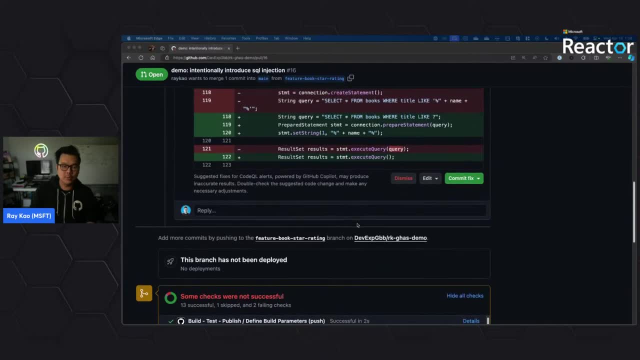 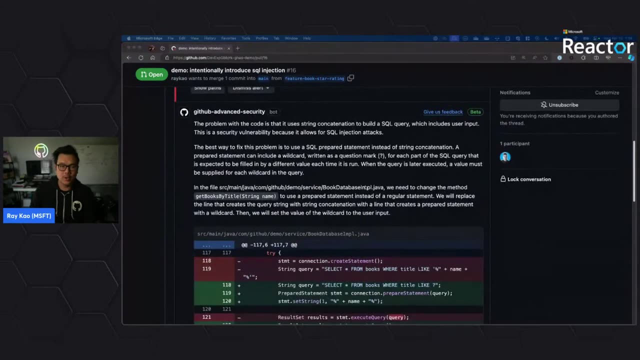 to call it. that's trying to upload or report the summary back to microsoft cloud. so that's still running. what you're going to see here is that the generate output, uh, in part from our own, you know. uh, get up advanced security, uh, quick search, online application management- uh, that's. 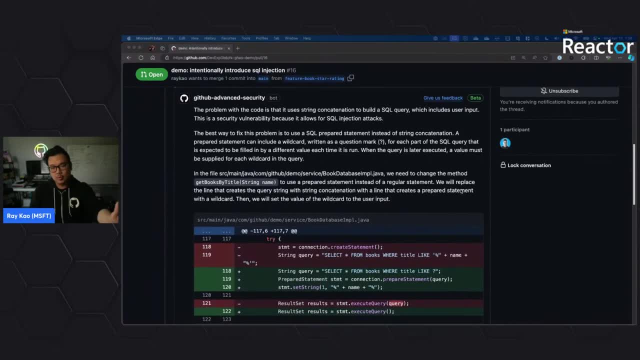 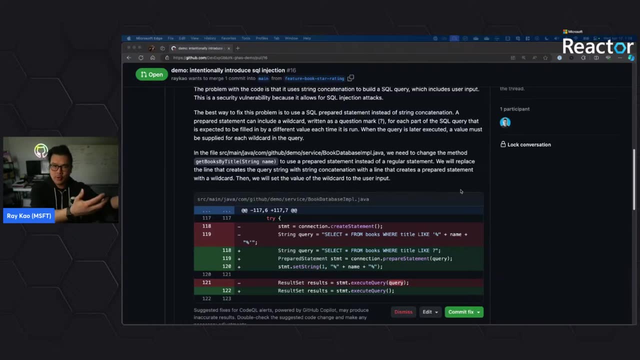 the msd01, the microsoft defender for cloud. you'll see, here's what you can see. here we are actually AI and tooling to say, hey, you know, we've scanned through your code, we've created the graph, we're able to actually see that the source of an input, one of your arguments. 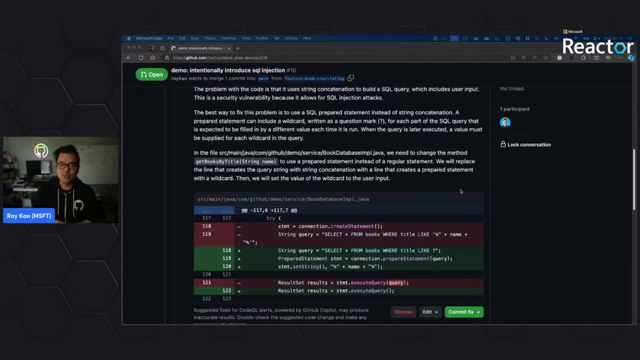 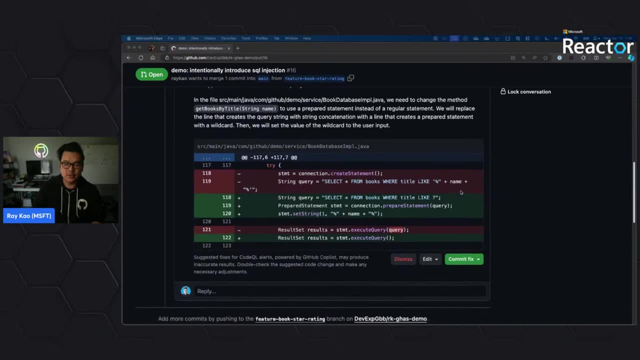 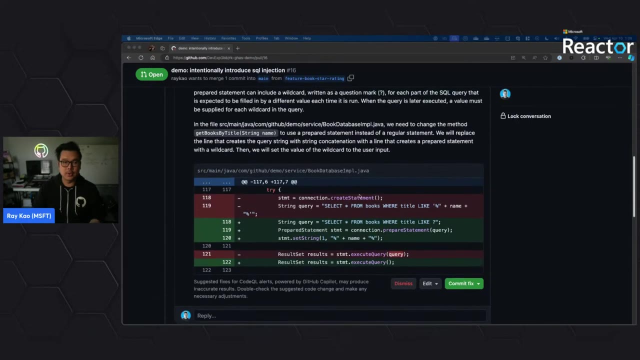 parameters right is being passed through your whole application and is introducing a potential vulnerability in your SQL injection, essentially right. Here is the suggested fix for that given issue that you have. So this is part of the code scanning, as you mentioned before. here it is its feature. 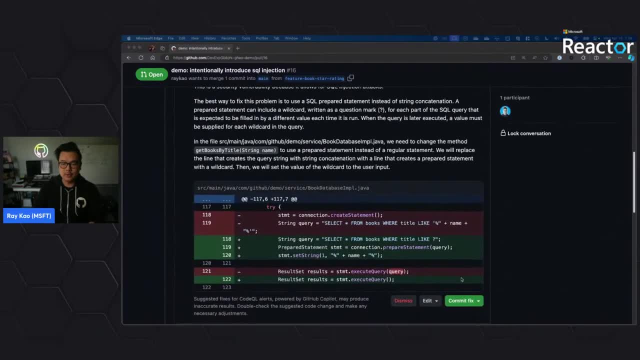 is already here. it's generating the PR that I want to do or not the PR, pardon me, asking me if I want to commit the given fix that it has suggested and we can do so. So I was going to say, yes, commit the fix right. commit and apply changes, say demo. 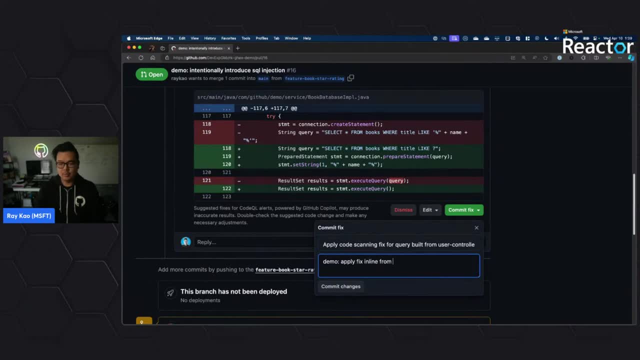 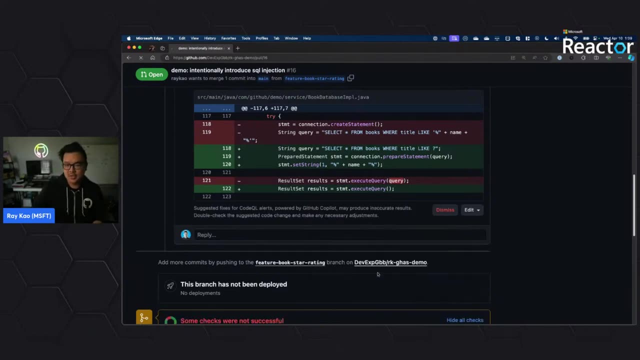 apply fix in line from gaz comments. You know I'm not very good with commit messages. Hopefully you are, and I'm just going to say commit changes. Hopefully that was descriptive enough so that in the future we'll see why. 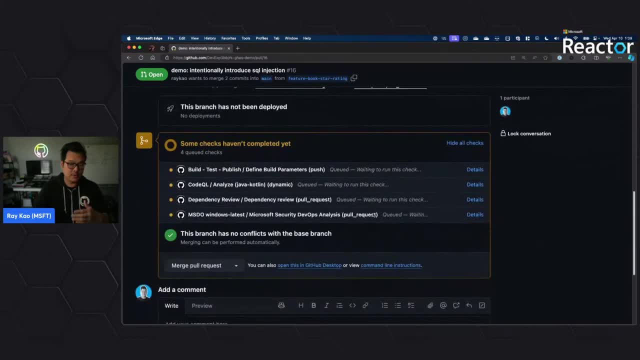 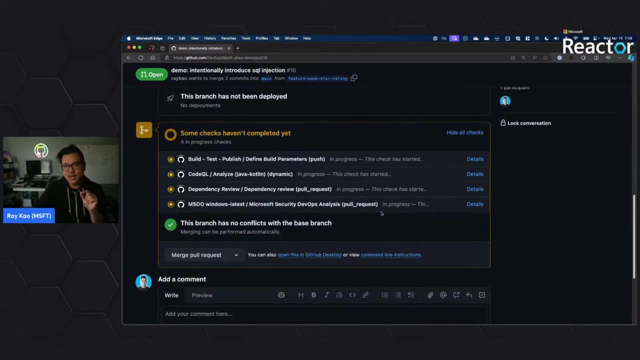 So it'll go through the testing again because essentially I've added a new commit to the same PR. it'll go through the same hoops. it'll likely still come up with an issue because I haven't actually resolved the log4j problem in my code directly and bumped the 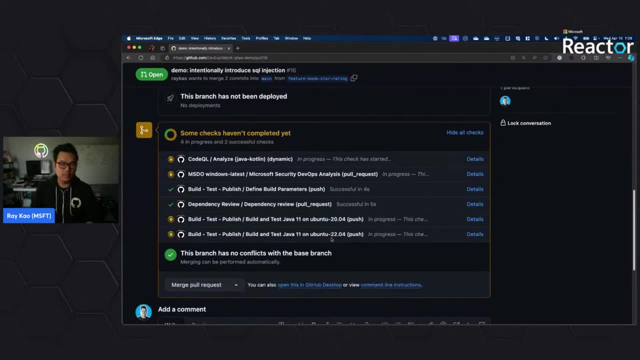 version, but it'll go through the same hurdles to get this done. Questions: am I planning to share this repo publicly after the presentation? This particular repo? no, because there are, let's say, components to running it that have requirements that I can't share. 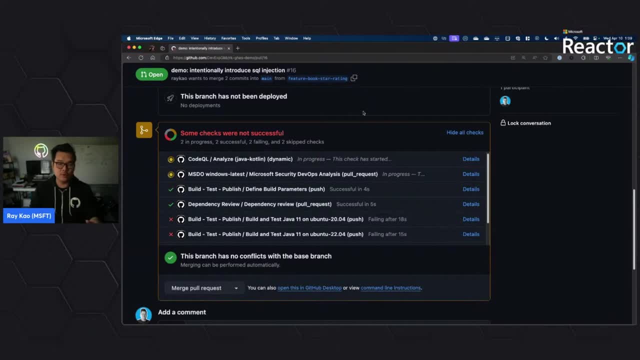 What I will attempt to do is have a sanitized version of it that I can share. I apologize in advance that I didn't have a public one that I could share immediately available. you know, day job concerns and what have you. But, Magno Logan, I will attempt to get it out for you. 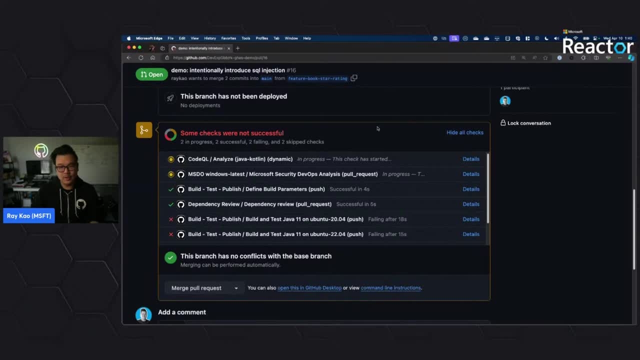 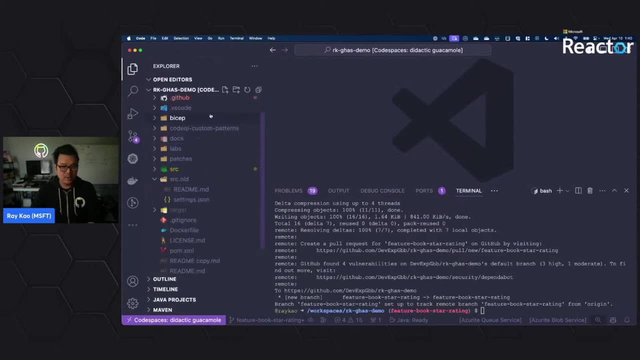 So it's going to go through the gauntlet. it's going to have the same kind of issues that we saw earlier. What I'm going to do is actually go back to my code and just kind of remediate and push it back and hopefully- if I didn't mess up the demo- I'm going to fix the vulnerabilities. 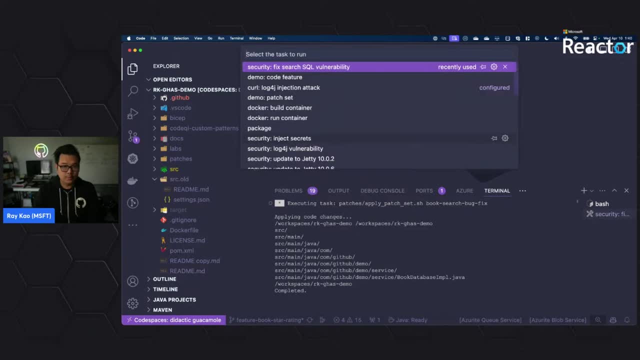 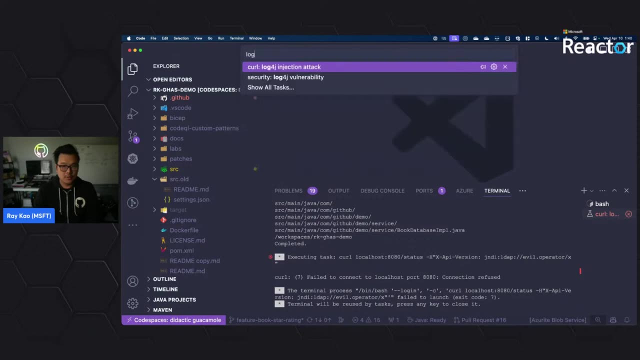 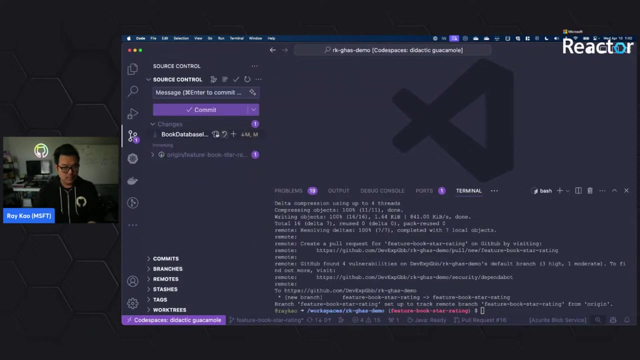 and then fix the log4j as well. Oops, no, that's a curl. one Log patch should have been All right. Hopefully I did my job properly, Okay. so this one's asking for incoming? That's okay, I don't need that one. 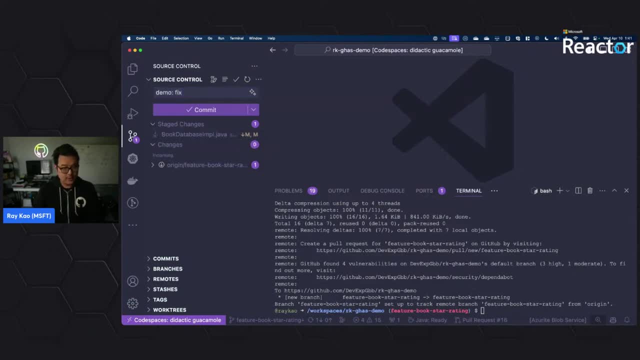 I want to add the update demo fix, Let's call it bugs, let's call it, or self-inflicted problems commit, and then I will push that one up Because it doesn't want me to. It's the UI, it's not tripping me up. 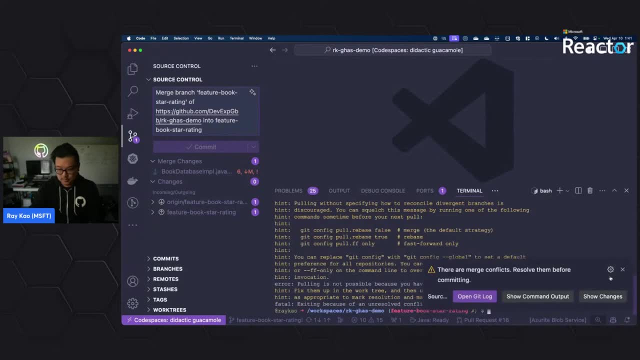 Always do command line. Hmm, Hmm, Hmm, Hmm, Hmm, Hmm, Hmm, Which one? Always demo problems? Okay, Good poll, I'll fix it. Fix them up on tree and remove appropriate unresolved conflict. Which one is it? 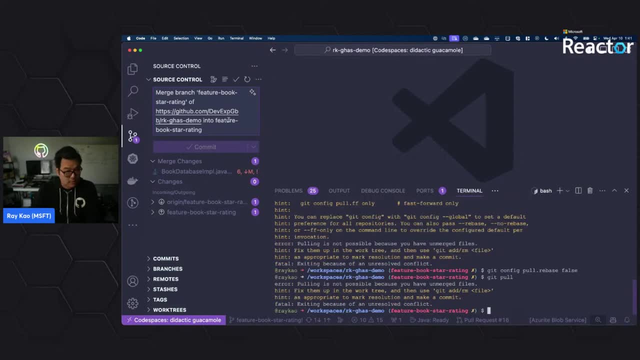 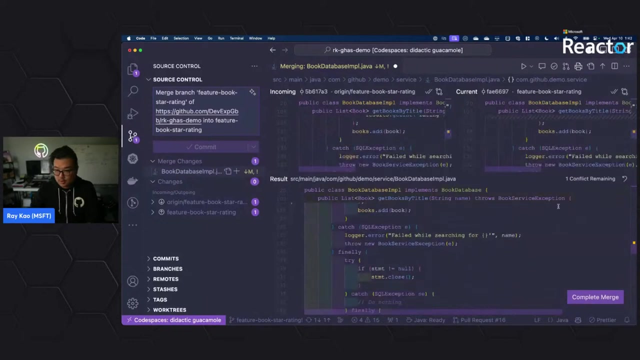 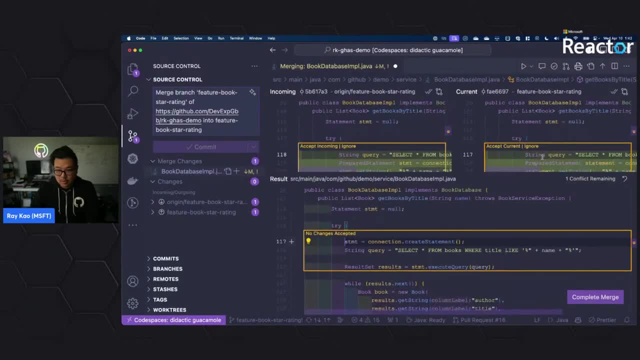 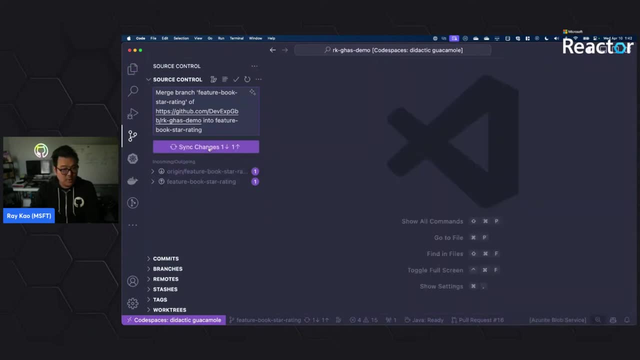 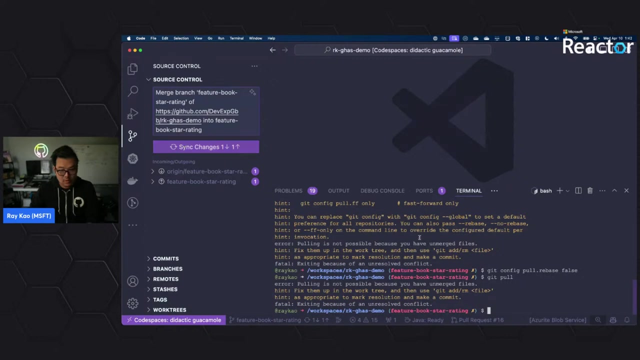 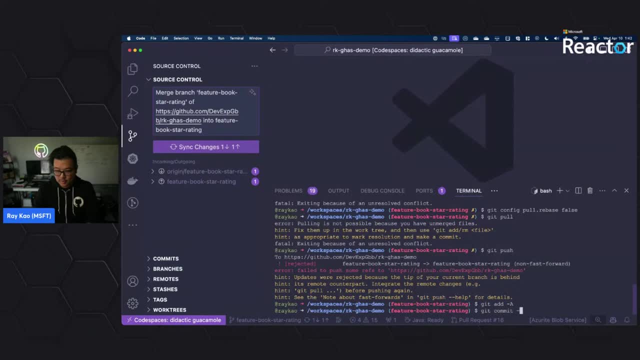 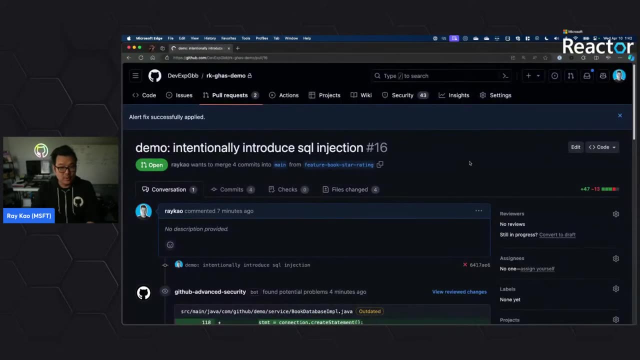 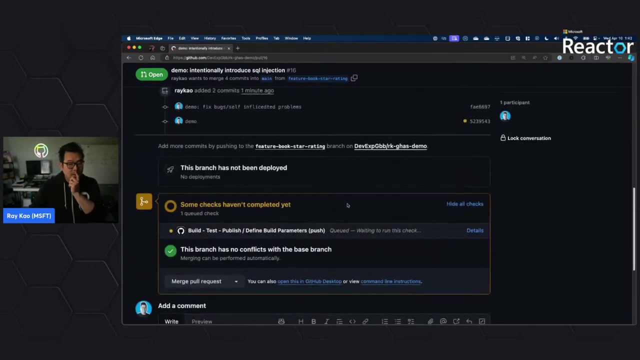 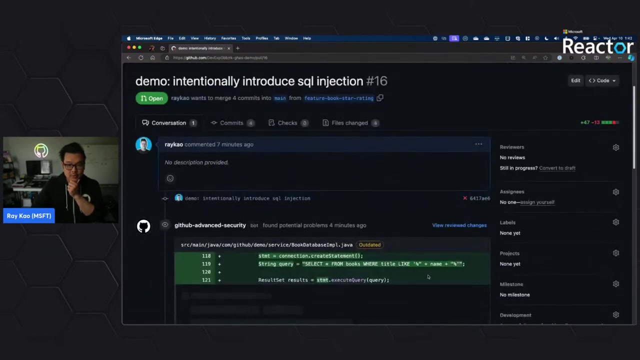 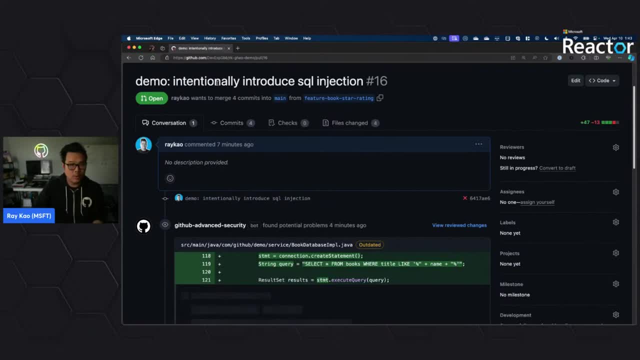 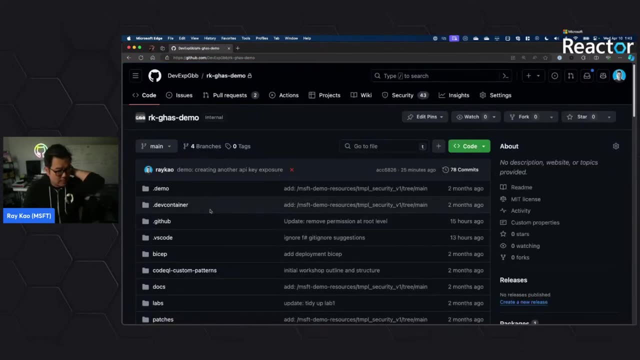 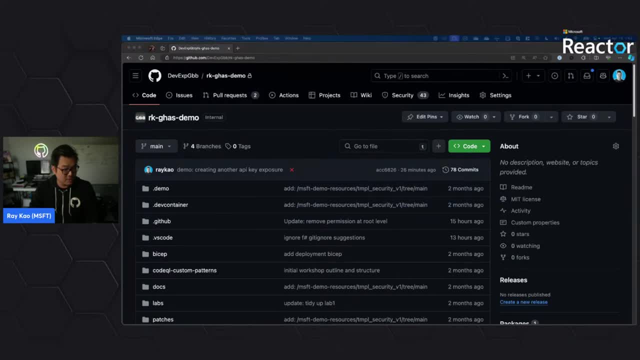 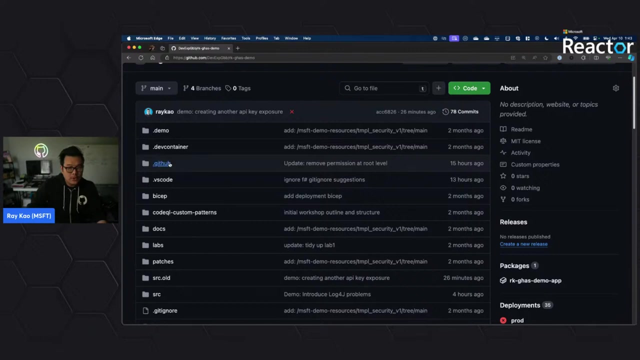 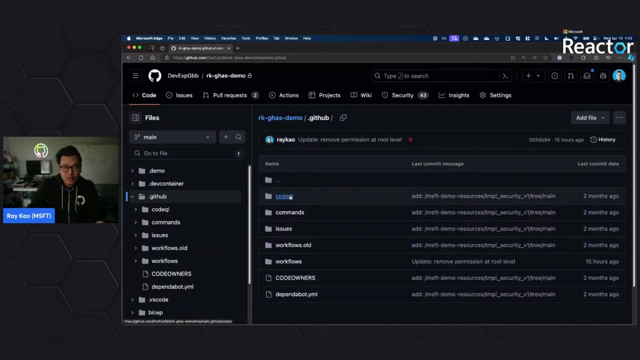 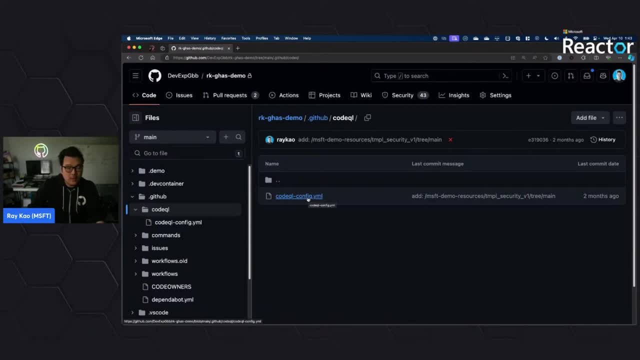 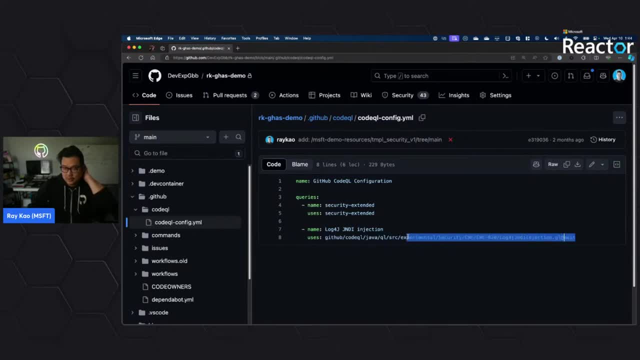 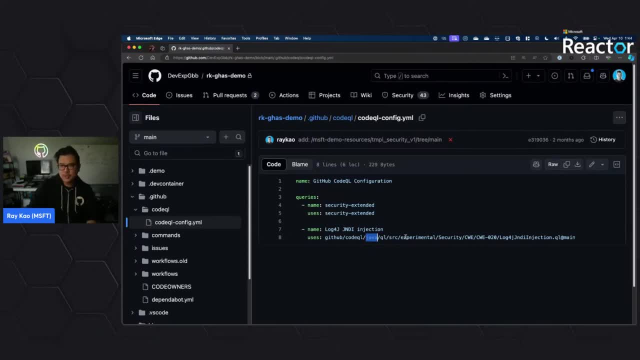 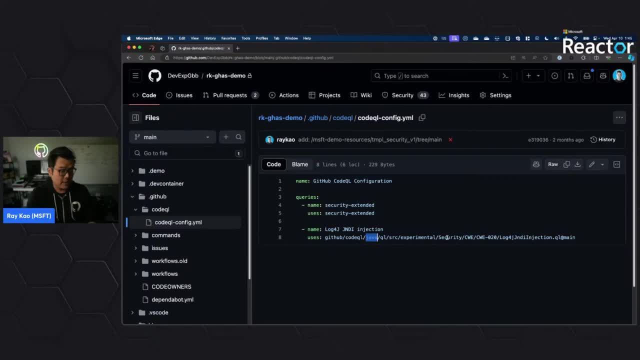 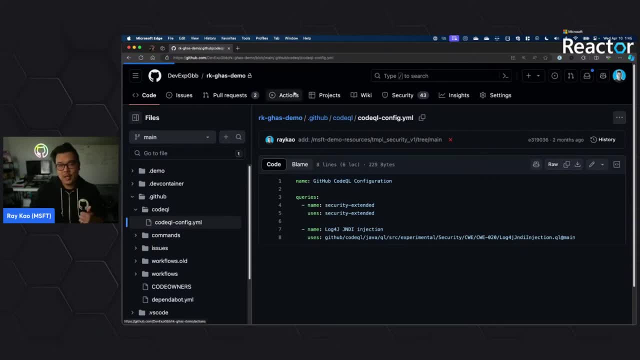 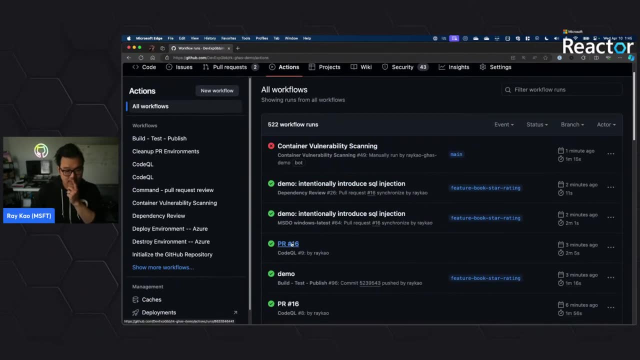 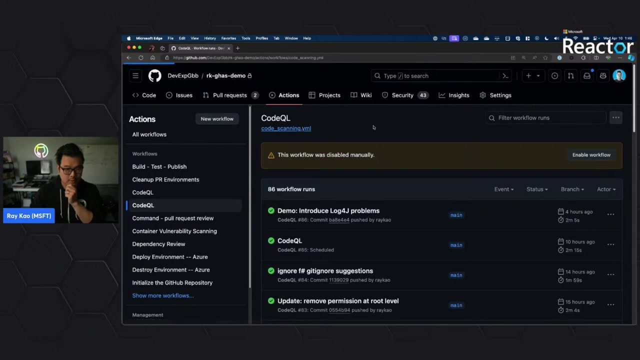 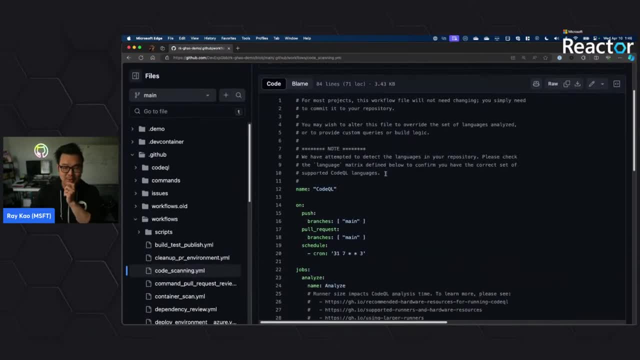 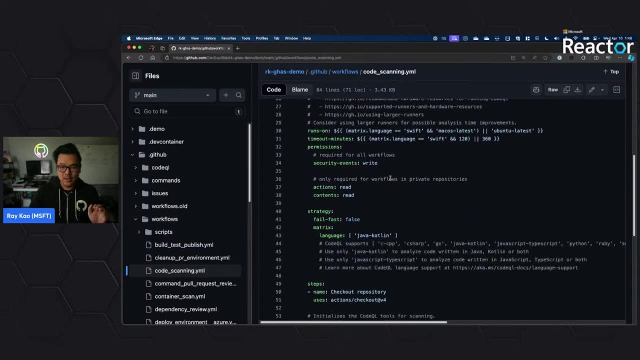 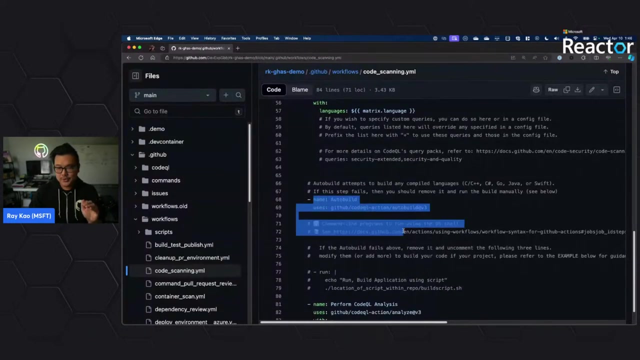 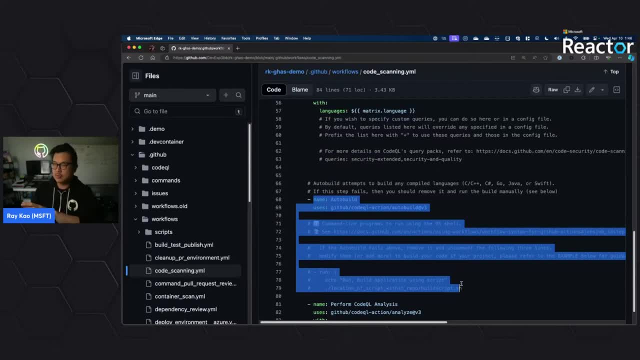 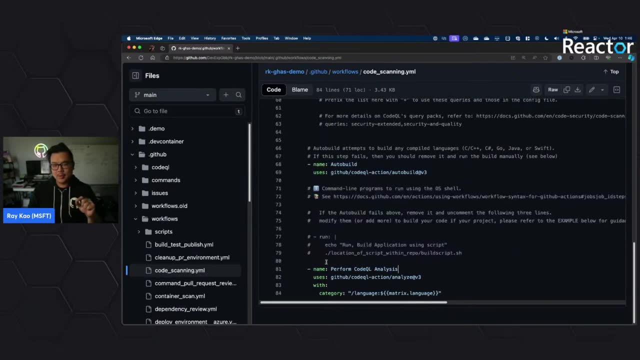 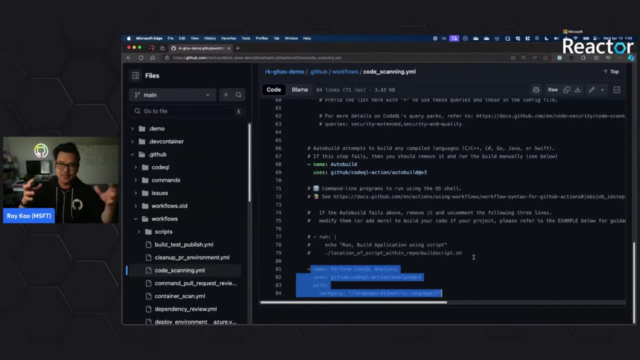 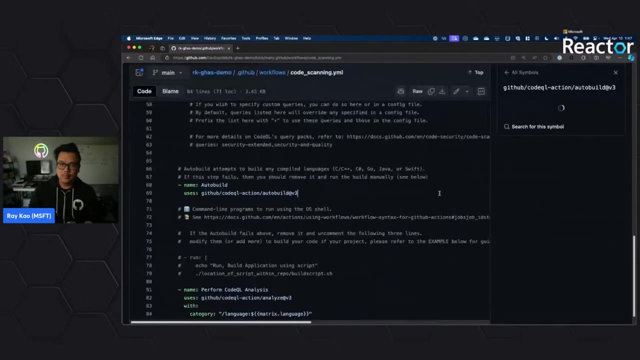 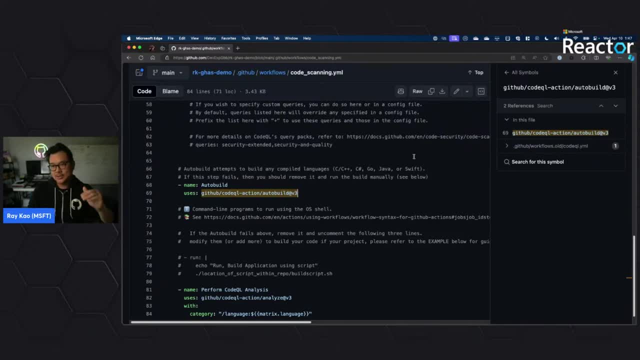 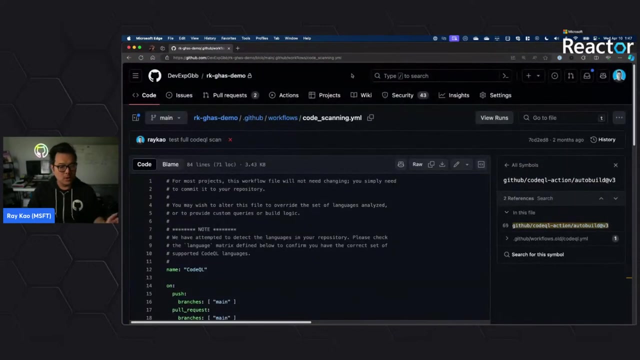 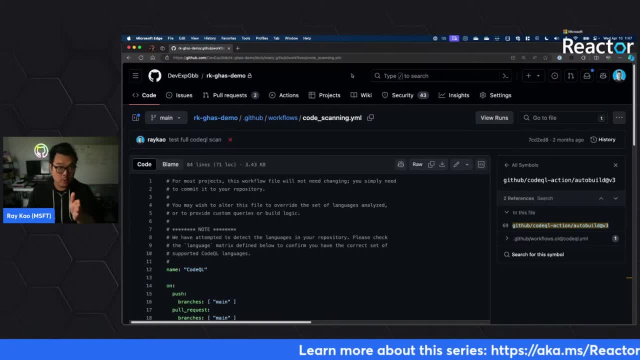 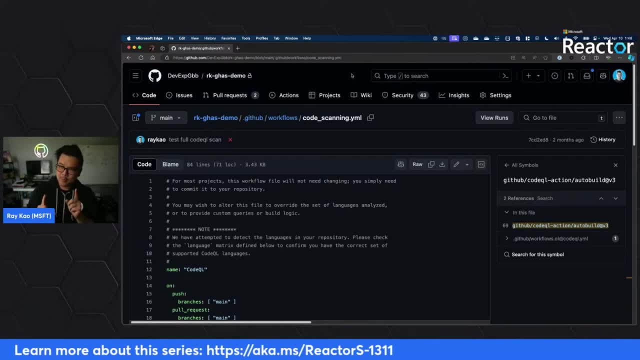 by the github uh security lab team probably butchered that team name, but that's what i remember them being called: uh. they provide that added into the platform and those behind the scenes- um- are not using uh codeql. it's not using um what's probably a combination of like regex. 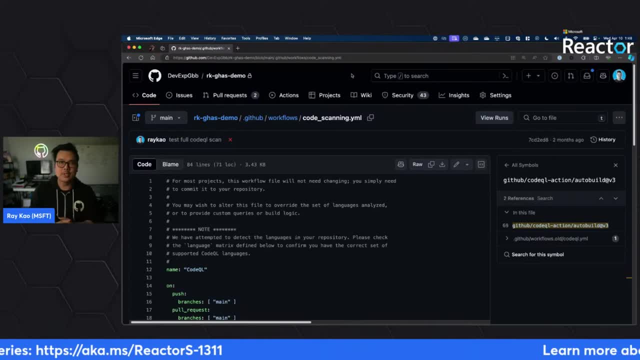 and other ways that pattern recognize. but there are models that will detect, uh, those things as well behind the scenes. so that's a difference, you know, from implementation perspective, in terms of how they actually run behind the scenes. um, so is there a difference between secret scanning code? 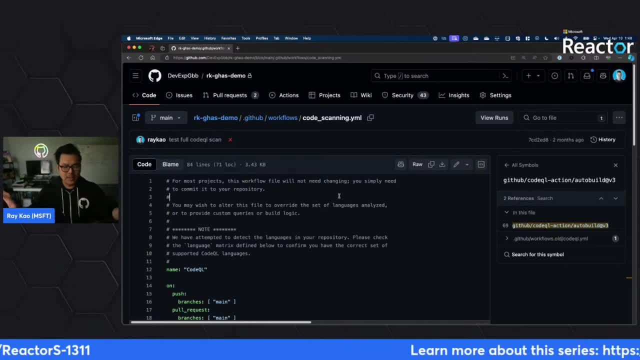 scanning rules for detecting hard code credentials. yeah, so that i mean, that's how they work behind the scenes. hard-coded credentials, um, specifically, is a scope, a secret scanning kind of functionality, um, but the uh code on the code scanning side of things, um, it doesn't really check to see if you've. 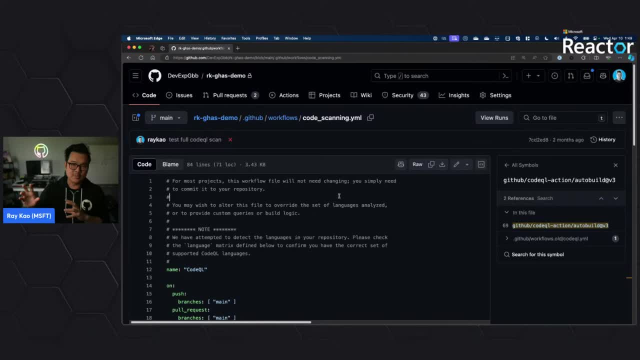 hard-coded a value. what, instead, is the way that it's modeled and graphed is it takes a look at uh sources- or you can think of them as inputs, uh syncs and uh- i forget the um, the term for it- but basically like passed around values and creates relationships around that, so it kind of can see. 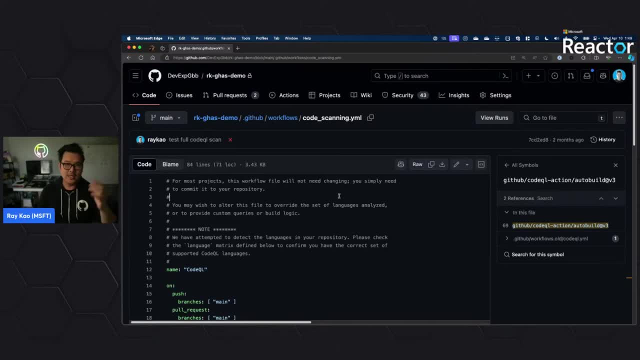 that if you're doing a rest, call, for example, we do like a ht post or put request i may have a payload and that i take, uh, one of those. um, you know, set, convert that, parse it as json, take the value in as unsanitized string value. i can tell from the graph that that is a source of information coming into a given 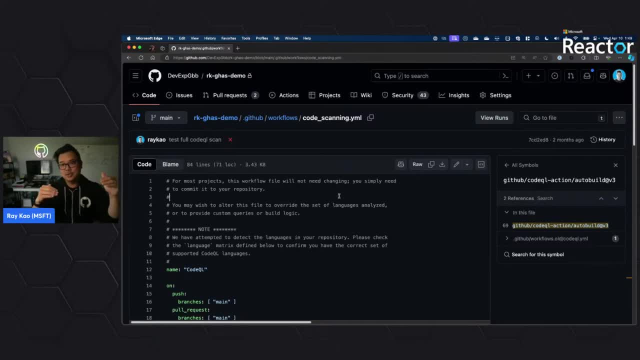 function. i can watch its sort of traversal through my entire application through the graph and be able to see, okay, at the end of the day, the next sync or the final sync, what is that and does that sync or any intermediary uh sync in between? is that causing a potential um attack or problem because it hasn't been sanitized? 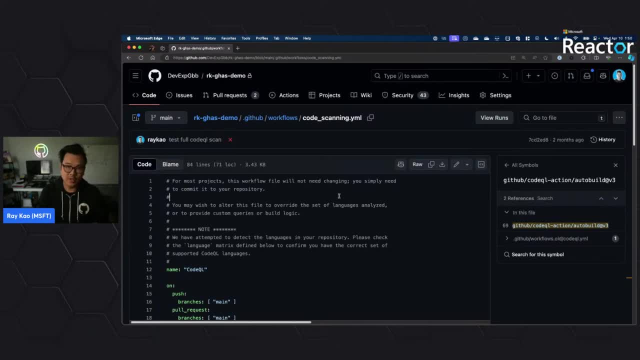 or you know, uh, hey, you're just accepting uh at face value a user input. so that's how the code ql graph mechanism would work. as opposed to code scanning is kind of less intelligent, less less advanced in that sense. it's just straight pattern recognition from a hard-coded string value. 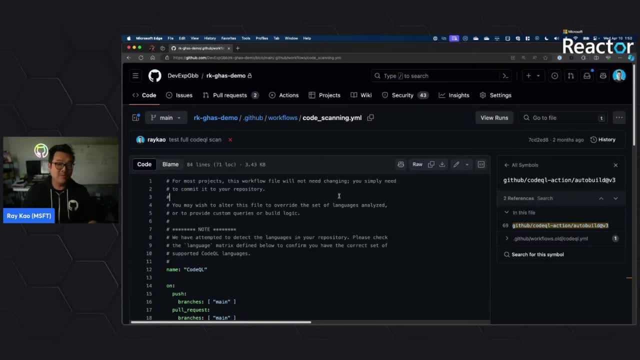 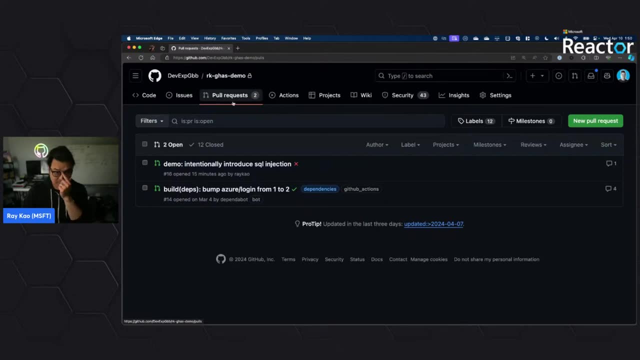 that was a lot of fun. so that's a pretty long-winded five five minute explanation of how those two things work, but hopefully that helps though. um, all right, i'm gonna go back to the pr with a little bit of time. while we have remaining, um, just go back in here. i'll probably mess this up. some checks were not. 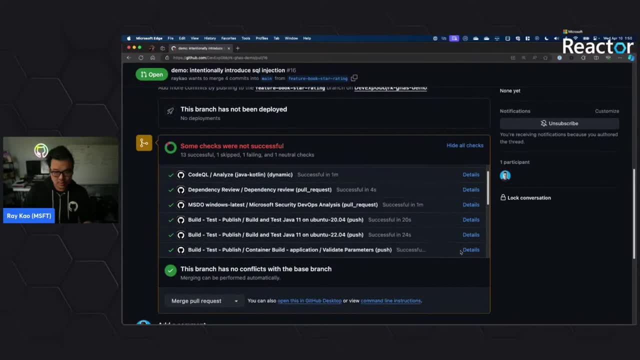 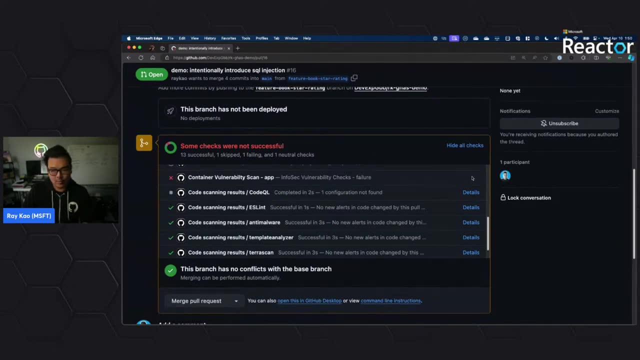 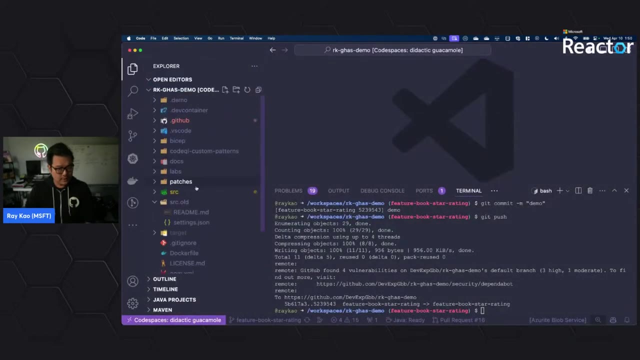 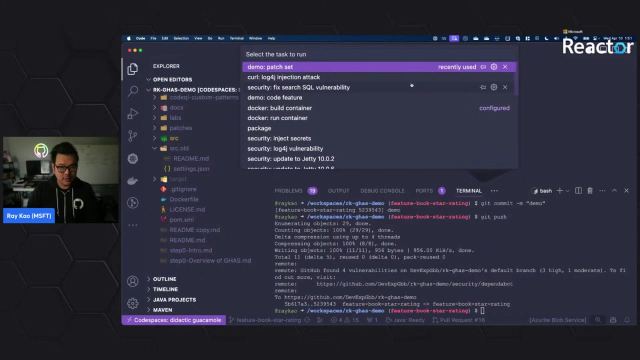 successful. which checks are not successful? what i'm feeling? uh, oh, because i didn't fix, actually, the log4j and roll that back. okay, um, i'm gonna go back to my files here. where did i put that again, that was i run. this is why the task runners are very important. uh, i'm gonna bump the. 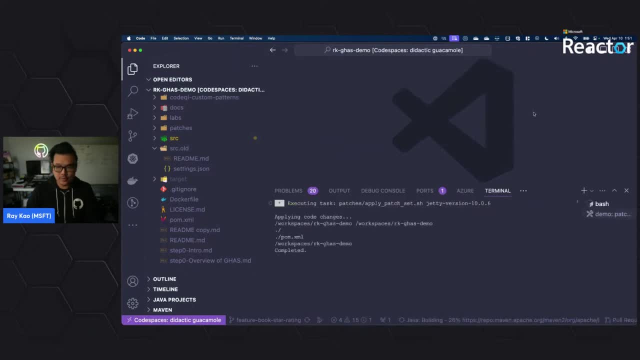 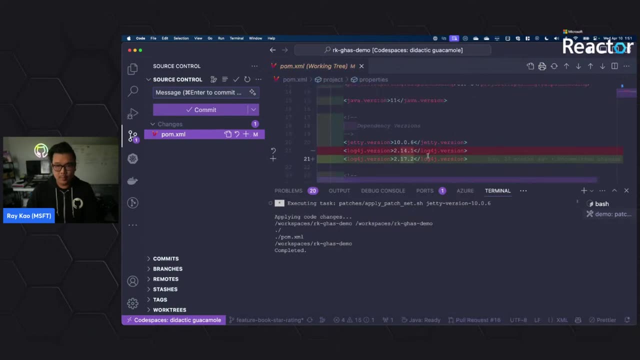 uh, jetty version. i think that's the one that will fix that, um, because it'll, if we take a look here, uh, it'll actually bump it up to a version that is, uh, not going to expose that particular version of log4j. that cause will cause me problems, so you know. 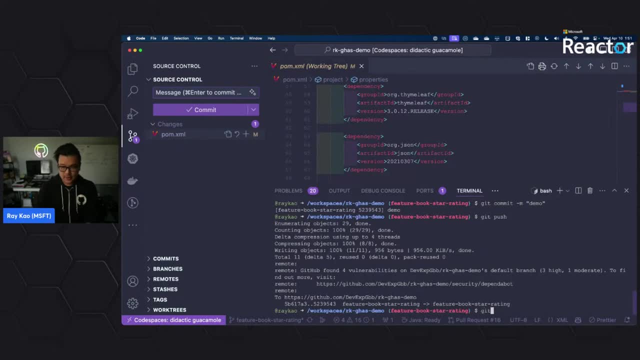 file here, and then what I'm going to do now is the same song and dance. get add everything because it looks good to me. get commit minus m demo fix log for j in palm that should be hopefully writing better commit messages than I am- and then I want to push this up accordingly, and then it will do. 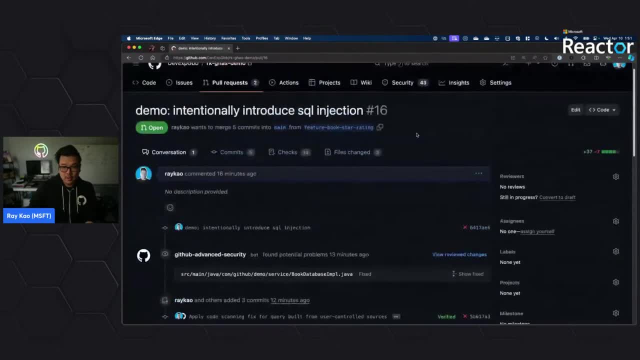 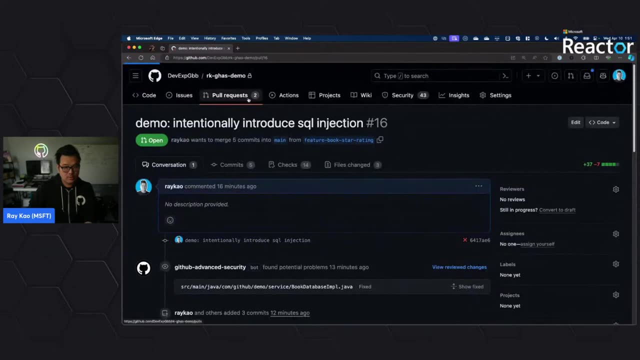 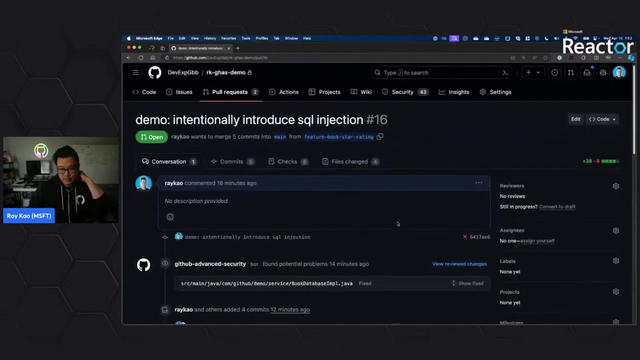 the same song dance and hopefully we can see it go green before the end of the time we have today together, so this will again um in a moment. yeah, there it is. you can see the the amber or yellow um symbol here that it's running through the whole song and dance again. I can see my whole. 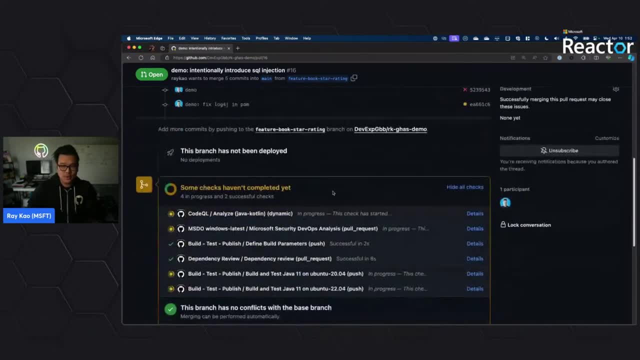 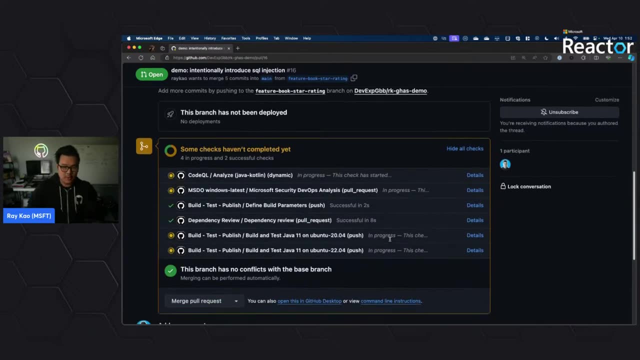 commit history, the fixed log for j and palm and commit message, and it's, it's doing the same thing again. so hopefully this time uh, anchor or gripe, the container scanning tool won't complain, and then I would have fixed everything in here. but again the whole idea, concept, again it's going to. 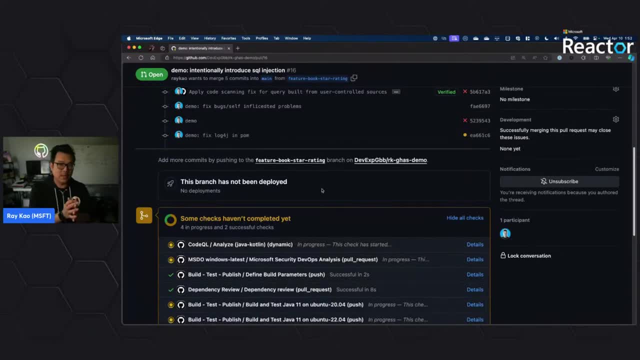 catch these things and it's going to catch these things and it's going to catch these things later on shifting left DevSecOps- all that good stuff built into the same developed workflow that you know and hopefully love in terms of commit messages, issues and inline PR comments. 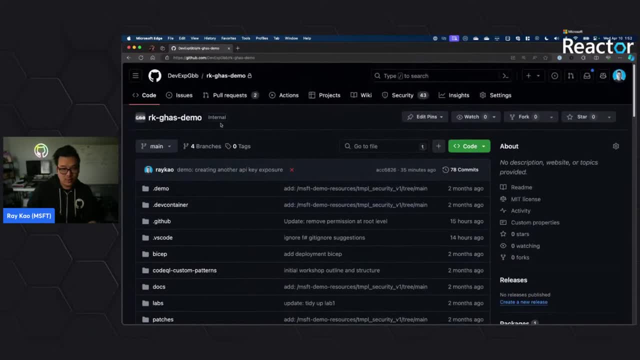 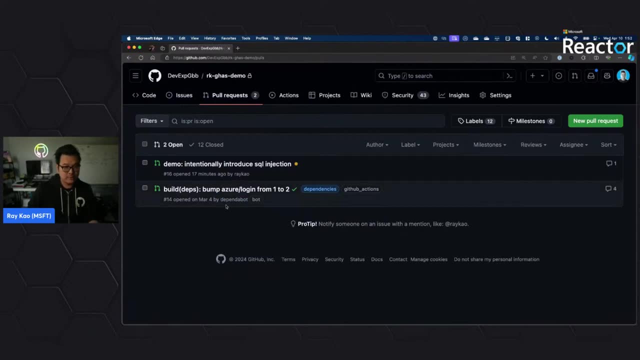 and like. so that's all I had for demo. we'll continue to watch and I'll watch the comments for any questions. additional questions: um, I guess maybe um a question out to the crowd and in terms of uh comments out there, you know how many, how many folks um previously had heard about GitHub, advanced security. um just say yes. 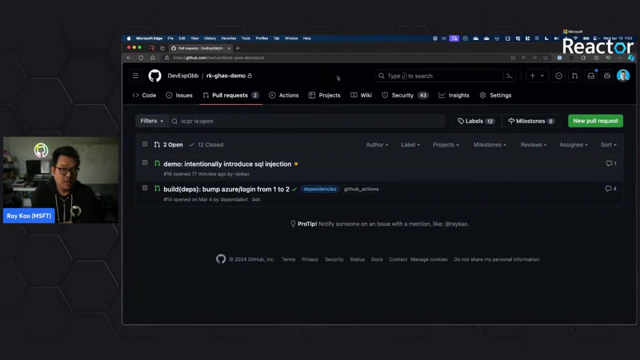 uh in in the chat and then, um, uh, for those who have actually, um, you know, got different static uh analysis tools out there, uh, if you, you know, got questions in terms of comparisons between them, um, go feel free to put it into the chat. um, and if you've, if you've got, uh, any specifics in terms of 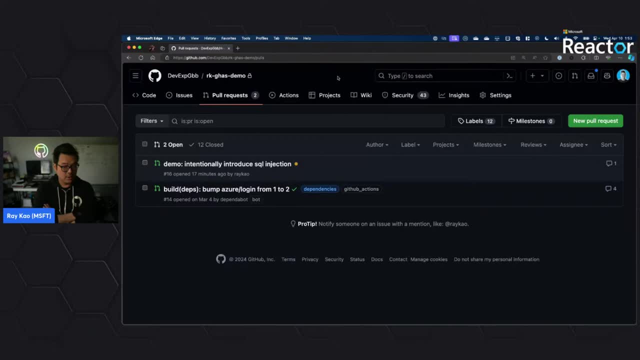 uh, how to use this a little bit more. um goes well, um, one of the big things I would probably mention before we close off is that, um, this is a defense in depth thing. so if you're really in cyber security and application security, there's not going to be a tool that is a silver bullet. uh. 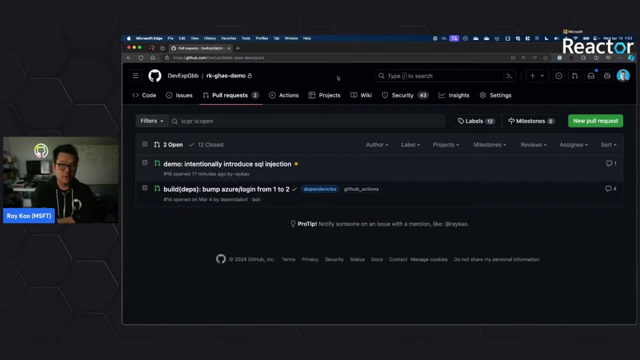 to cover everything. it'll be a combination of all this, and what you're really looking for are additional data points to ensure that you have better and better coverage. I think the one major thing about uh, CodeQL, uh and GitHub- advanced security and code scanning that we uh- I want to use the word pride- 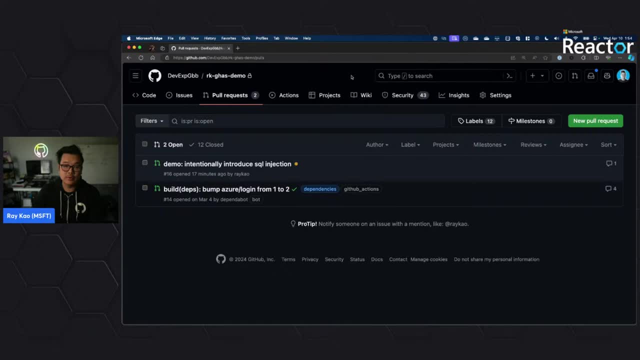 ourselves on, but we we try to do the best. um, and we believe it is the best tool for is reducing the number of false positives. right, um, you don't want to be constantly inundated with alerts. right, you don't want things that are, you know, red herrings or wild goose chases. um, the tool is designed. 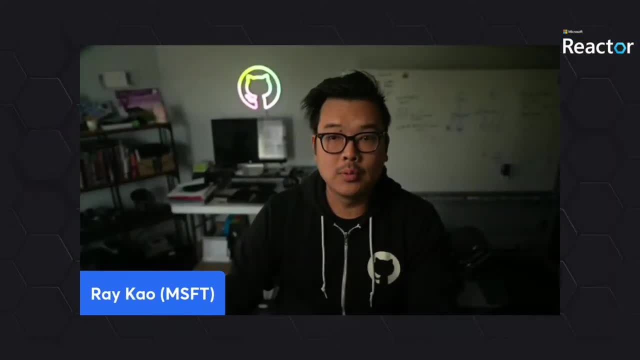 to you know, provide you with accurate um alerts and and things that aren't going to waste your time trying to fix and and to that point we're also trying to make it easier to fix um by introducing those pull requests and issues and things like that that integrate into again your 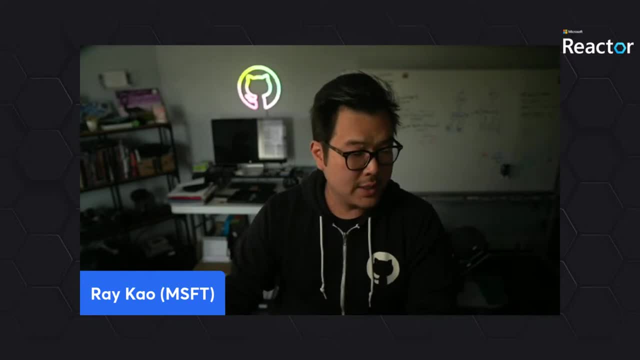 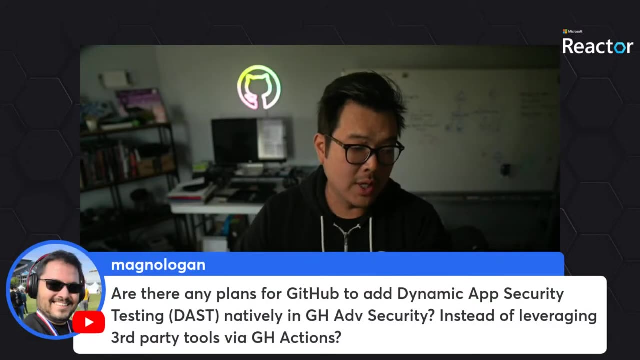 developer experience in there. are there any plans for GitHub to add dynamic app security dast natively in GitHub advanced security instead of leveraging third-party tools via GitHub actions? um, not to my opinion, we're primarily focusing on the sass side of things. uh, so static code analysis, side of 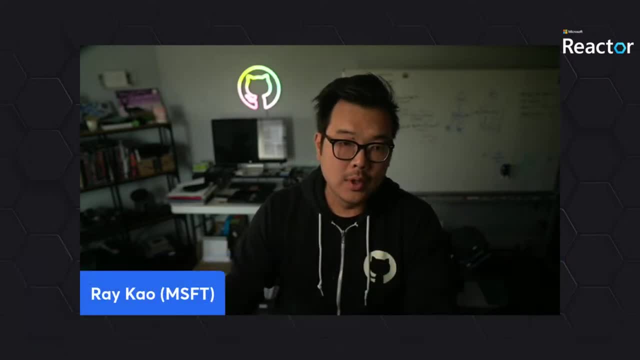 things uh instead of uh, dast, um, mostly because, again, we think that the dynamic side is a little bit more, I don't know, personal opinion. I think it's a little bit hard of a nut to crack. in that sense the sass part of it covers quite a bit. um, I love if we- this is live and we had an in-person. 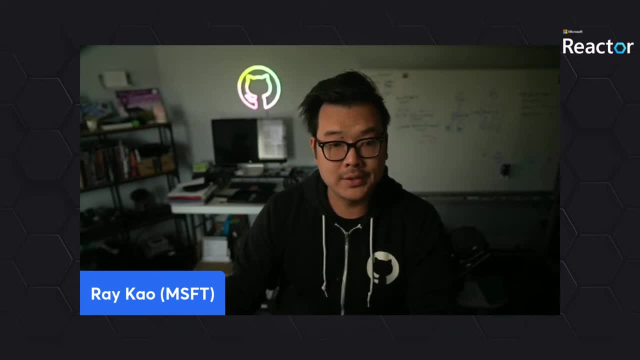 kind of thing conversation afterwards. I'd love to have a chat about it and your thoughts, um, but you know, short answer again. uh, no, not to my knowledge, it's not on the roadmap to have a dast solution there. um, next one is: is there a way to easily? 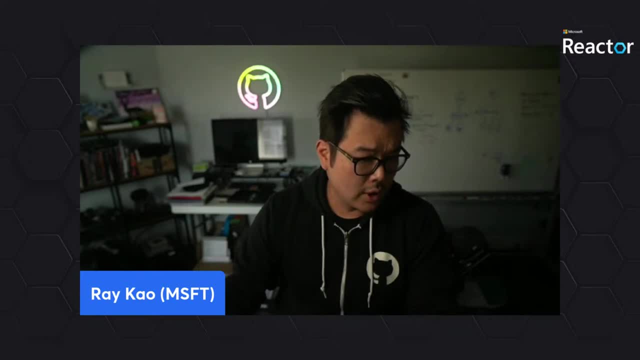 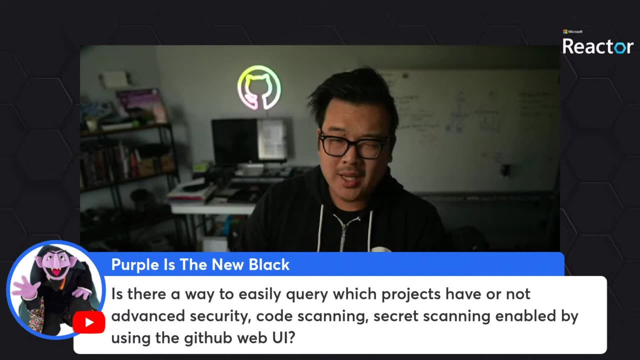 query which projects have or not, have or not advanced security code scanning enable in the GitHub web UI. so, um, yeah, at the org level, um, I can't show you my org only because it might show some things that I shouldn't show, but the org level you can actually go run through. 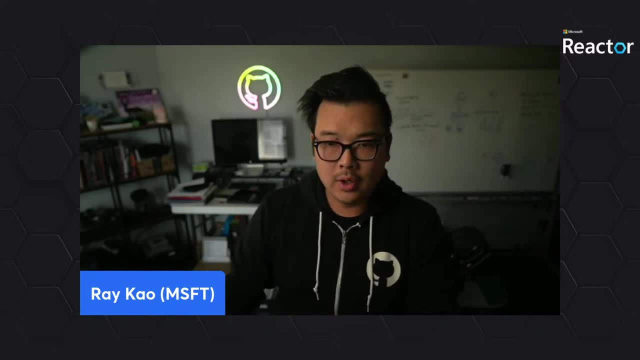 um and see which repositories have GitHub advanced security turned on. you also have the ability to see in billing, because code scanning, for example, is turned on on a per active developer basis. so if you're a developer in five repos and only one of them you're actually using code QL or advanced.